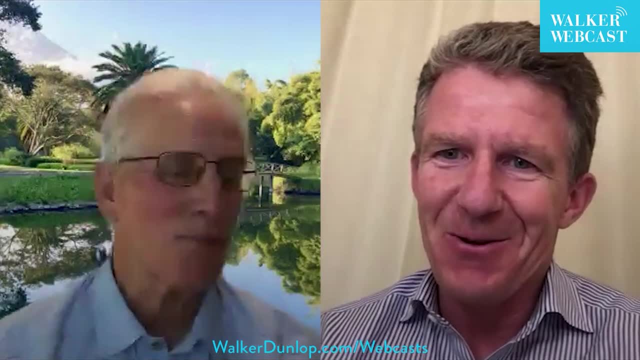 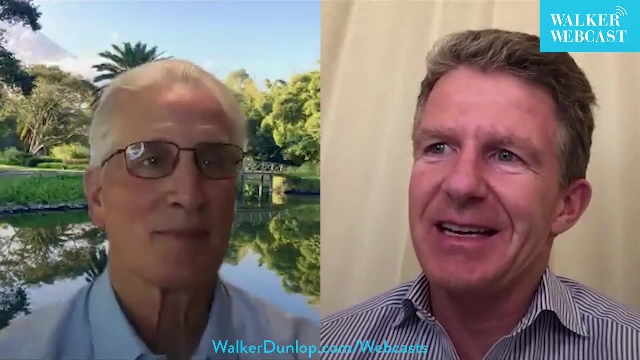 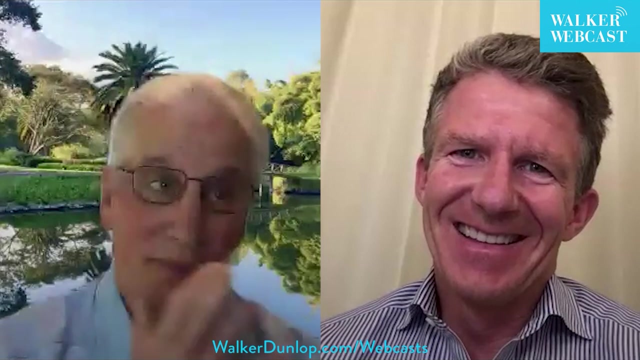 of the world. You've gone back that way. I've come this way. I was in Morocco, which is a fascinating place also. Yeah, And I see you have. is that Augusta behind you? No, it's not Augusta, No, no, no, Although it looks, it's actually in Guatemala. It's not a golf course, actually. 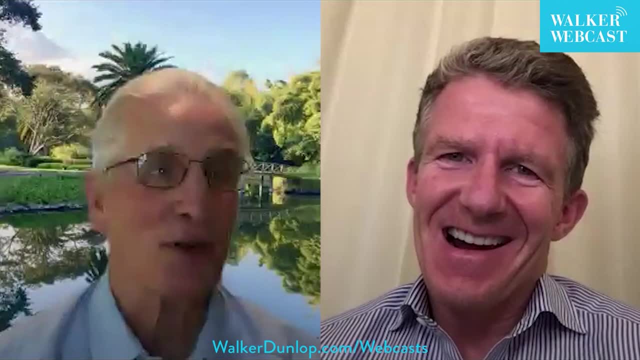 It's just a pretty scene. It's just a pretty scene I took a photo of while I was in Guatemala in January. Oh, it looks a little bit like the 13th at Augusta, And I know a lot of people who are. 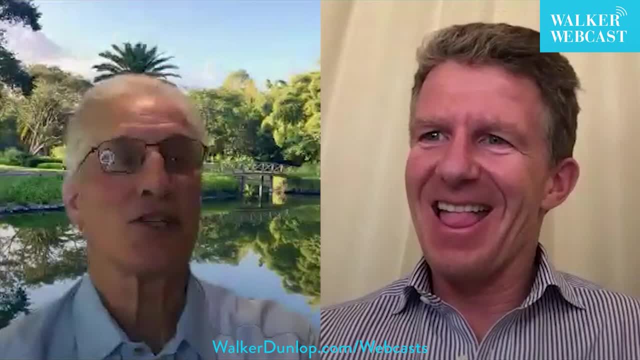 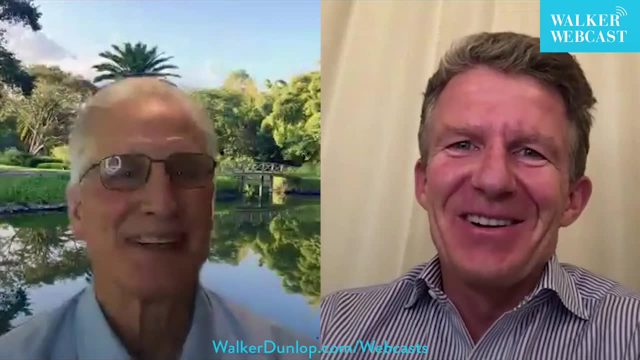 listening today. Look in the distance, you'll see a volcano. I don't think Augusta's got a volcano behind it, That's for sure. All right, We got a lot to talk about. Boy oh boy, do we have a lot? 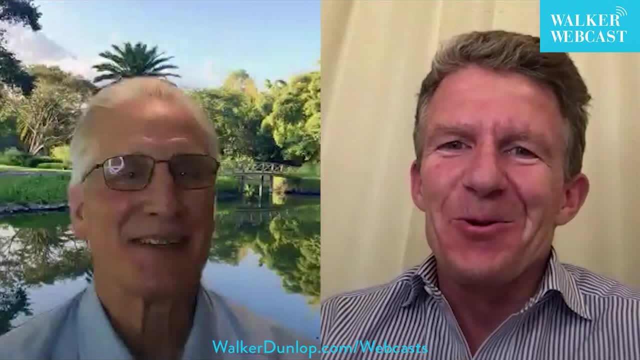 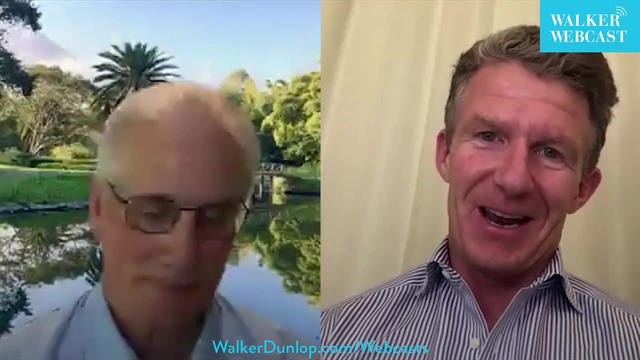 to talk about. I want to. I'll run through a quick summary of everything I want to try to get to, And we will try our darndest to get through it, because I know there are thousands of people listening today. We got a lot of great questions from people And there's some. 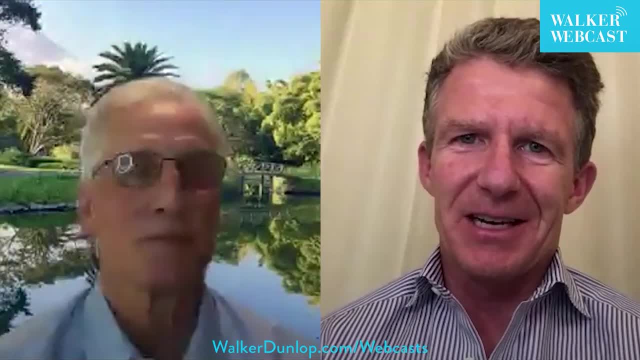 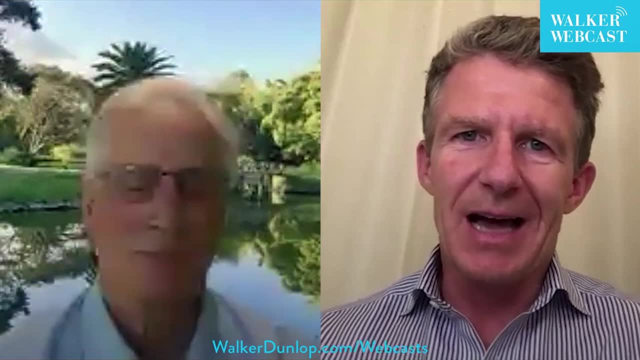 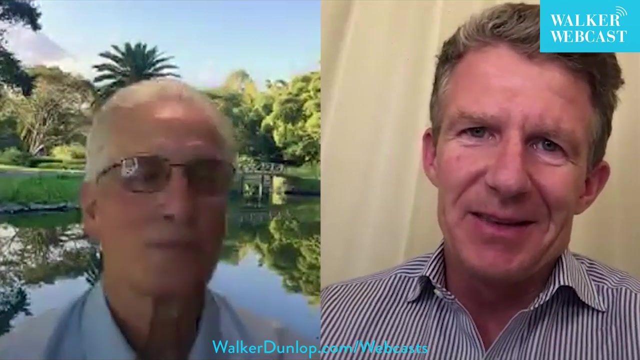 consistent themes that we will definitely hit on in our discussion today. First, obviously, is inflation. The CPI came out this morning. It was hot yet again. You and I will shake our heads at that, But unfortunately, we can shake our heads and look at the data, But 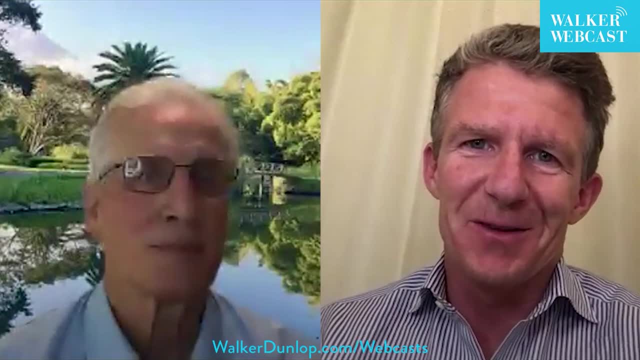 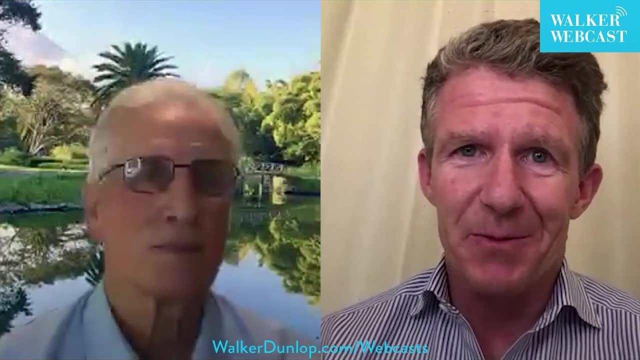 the number that they publish is the number they publish, and the number they publish is what the Fed's going to react to. So we'll talk about that. I want to talk about rates. We're at a 451 10-year when I last checked before we started this call. I want to talk. 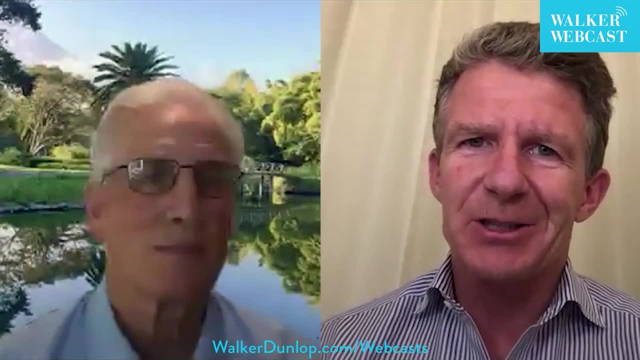 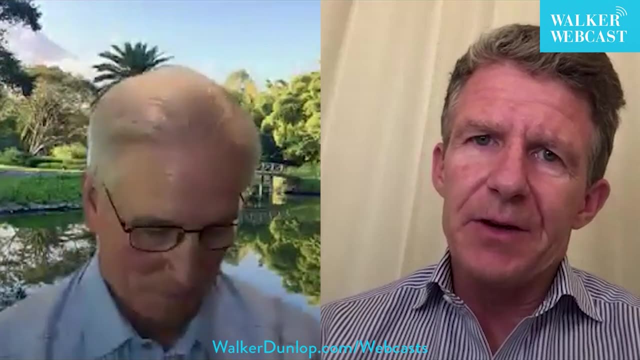 a little bit through your 20% discount world of why transactions aren't happening in commercial real estate right now. Got to talk about jobs. You've got some pretty significant job growth coming into the US economy over the coming years And I want to talk about how that plays. 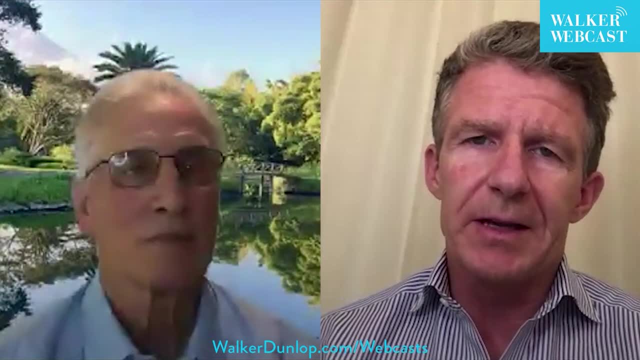 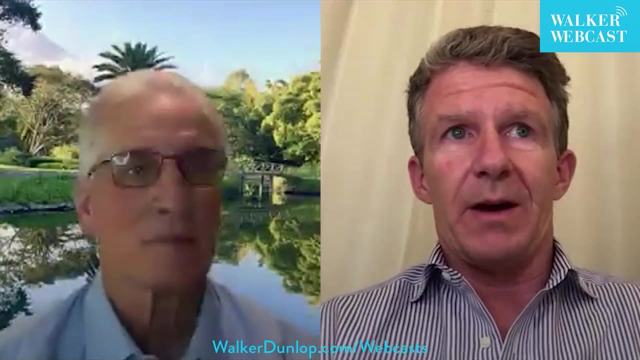 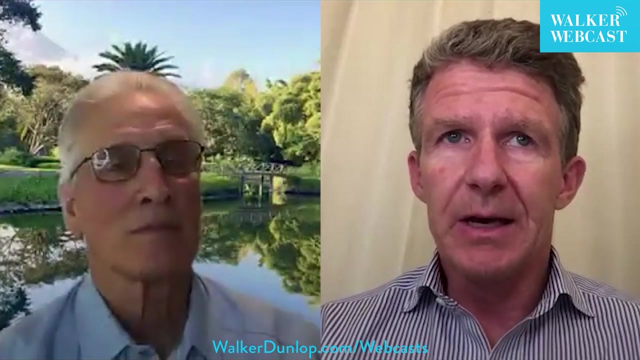 into a number of your projections as it relates to vacancy and absorption across various asset classes. I can't talk with you without talking about GDP growth. You've got some pretty consistent, I would say- GDP growth expectations over the next couple of years. How do those play out? 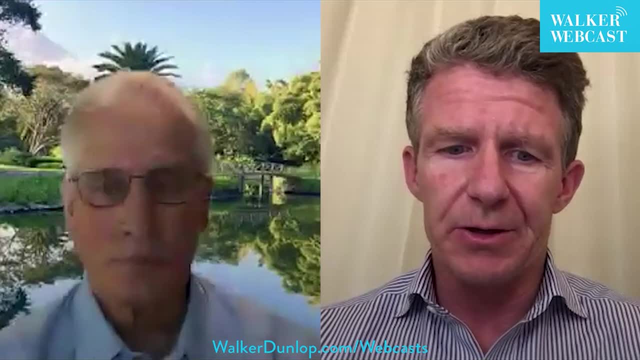 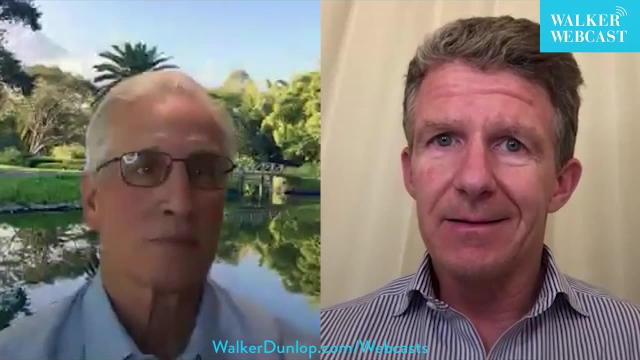 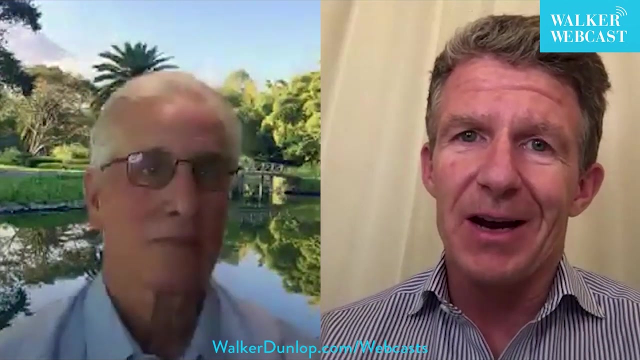 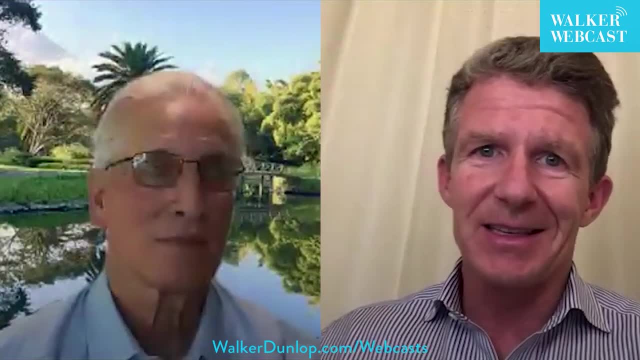 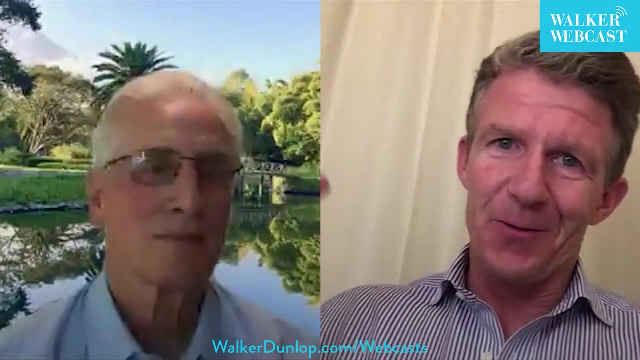 Fed. I'm going to go back to the Fed. We've got all sorts of problems on the horizon as it relates to the economy: overbuilding, oversupply, bank balance sheets, et cetera, et cetera. The idea that they're out of your 45 canaries, there are only four that are dead right now, And those are 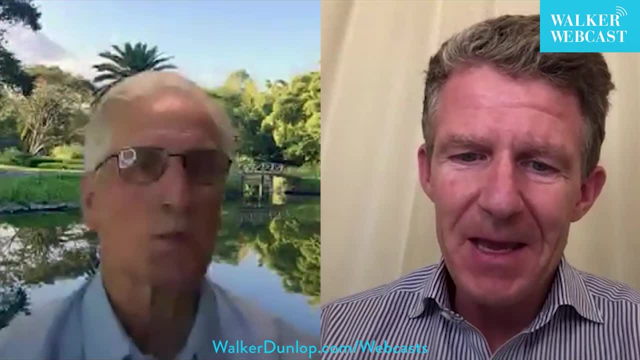 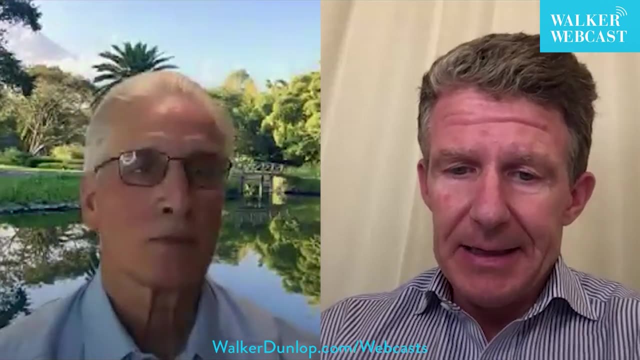 all related to misguided Fed policies. I want to dive into. I want about immigration. Immigration was something that was very big on the precall questions that people had Household wealth. I want to figure out whether your numbers are skewed by the fact that we have eight hundred and sixteen billion. billionaires in the United States that collectively have $5.7 trillion of net worth, and whether your average numbers are actually good average numbers or whether the concentration of wealth at the top of the numbers is skewing everything on a per capita basis: Bank, CRE exposure, the environment. 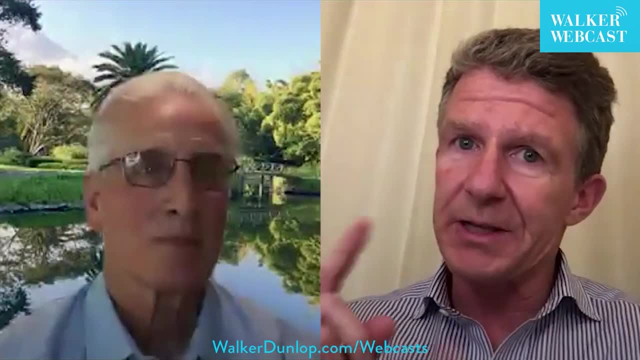 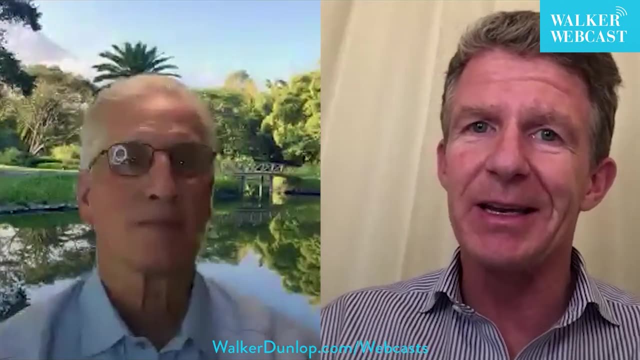 and then a quick dive into various asset classes as it relates to growth, particularly single family and multifamily. But let's back up, Peter. That's a quick outline of what I want to get to and we only got an hour to get to it. But let me run through a little bit of data here, because 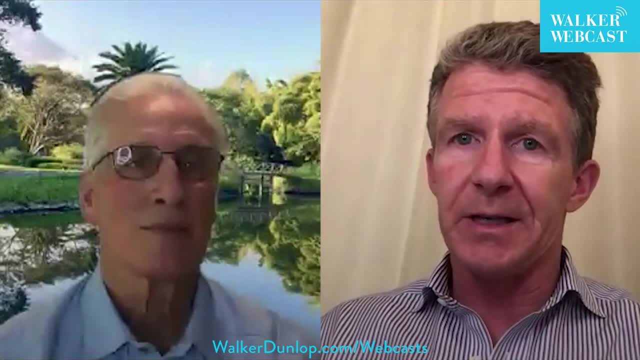 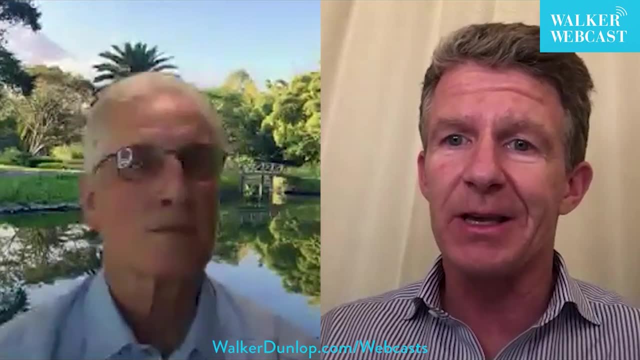 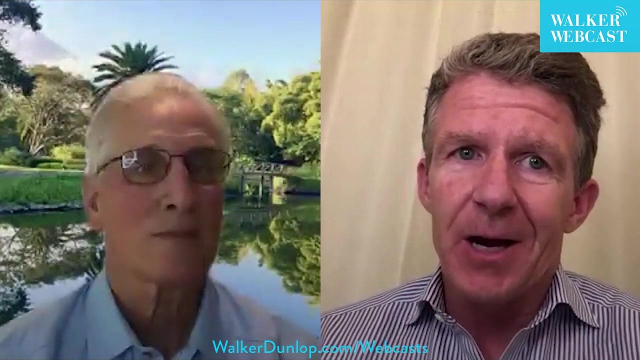 you're really good in having highlighted this before today's CPI print, But, as I sent you before this because I spent a flight from India to Dubai today looking into the actual CPI numbers, if you look at food, it's 13% of the CPI. It's up 2.2% over the last 12 months. 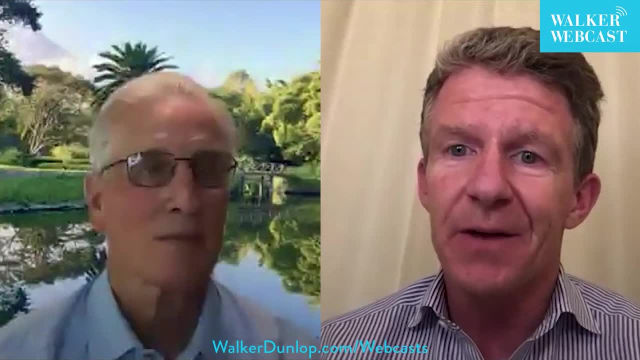 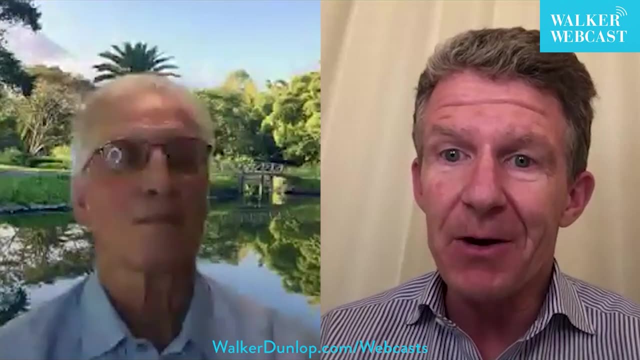 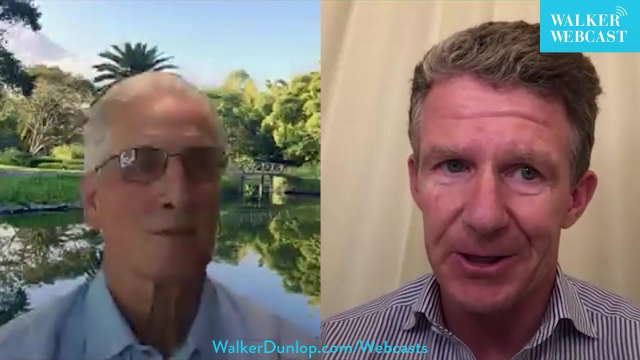 Energy: it's 6.7% of the CPI. It includes everything: Households, Households, Households, Housing fuel, Gas to put into your pickup truck. It's up 2.1% over the last year. Medical care: a very significant component: 6.5%. It's up 2.1% over the last year. 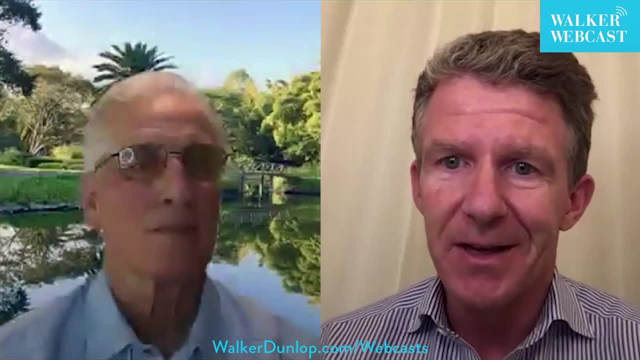 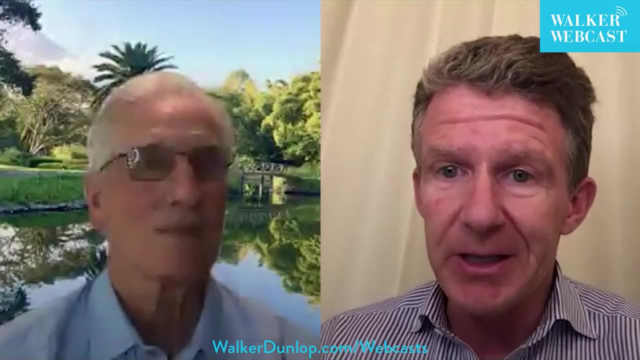 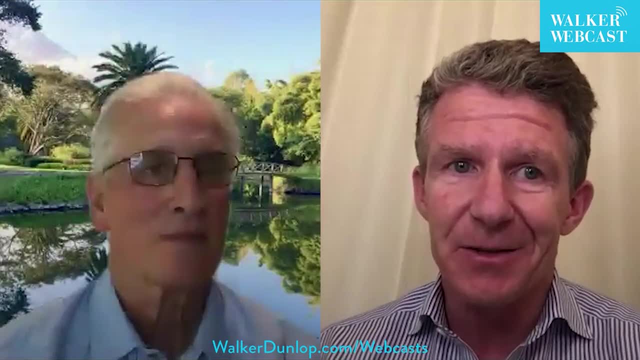 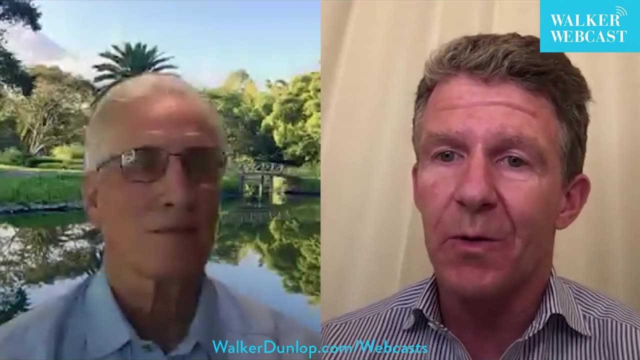 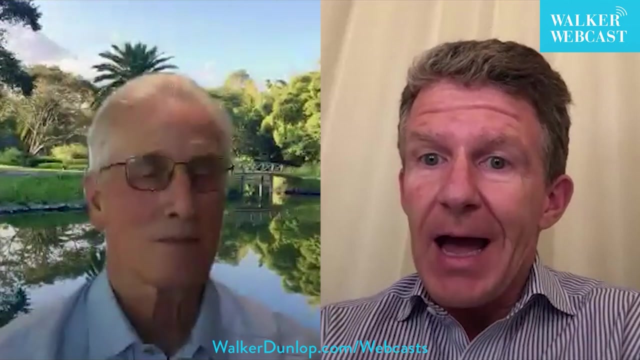 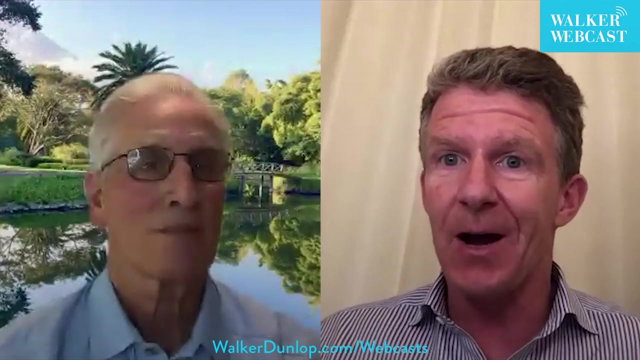 And, as you and I have discussed extensively, that 5.9% for single family is pulled from a survey of people of what they would rent their home to someone else for, Just to give a data point on that, Peter Zellman, which is our research group, tracks single family housing rental prices across the United States- Actual data, not a survey. We actually go in and find out what an SFR rented for a year ago and what it's running for today. 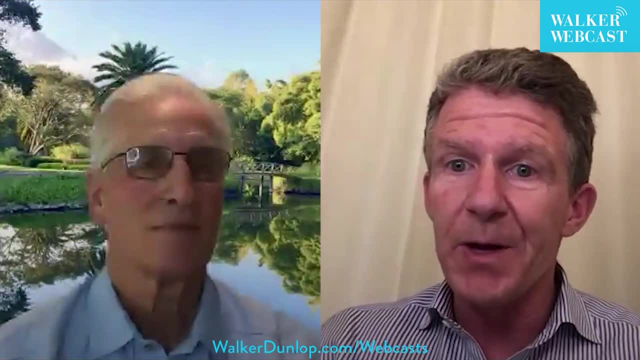 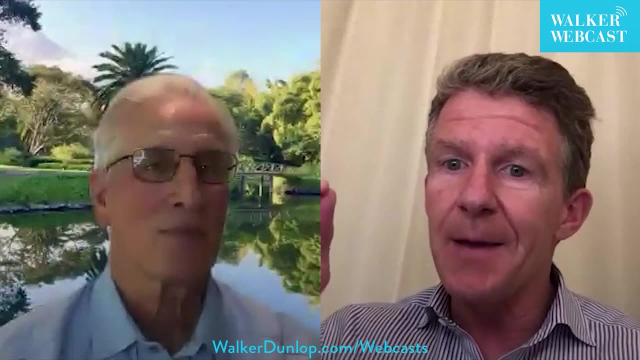 And in February, on February we have 3.3% growth, 3.3% growth in single-family rentals across the country. So here's a BLM number that says 5.9% on single-family when the actual single-family 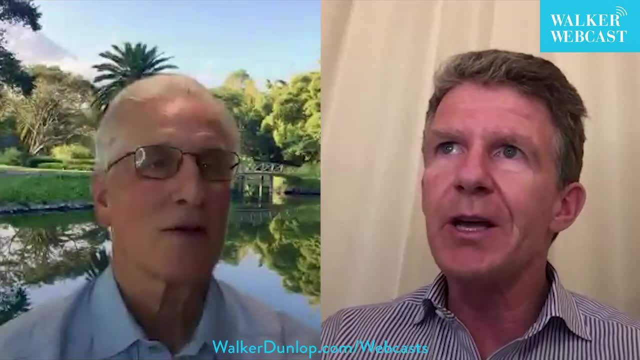 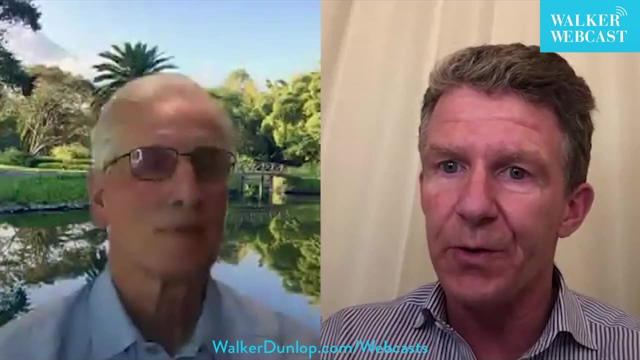 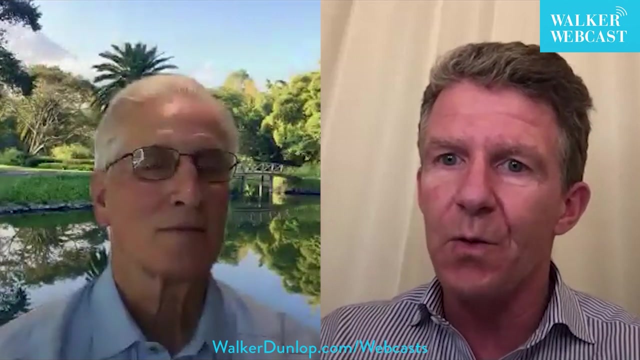 rental number is 3.3.. So you think about what that 260 basis points, taken out of today's CPI print, would mean. That's an actual number on 3.3% versus a subjective 5.9% survey number And as a result of that we've got a 451 10-year. 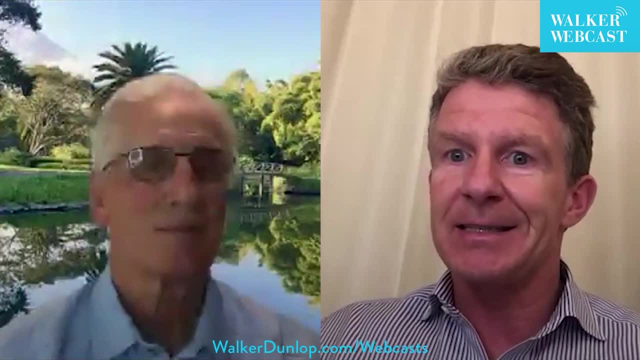 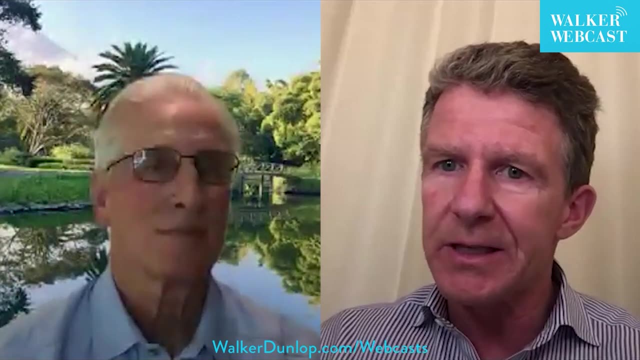 We've got every interest rate intensive industry down dramatically today. Rocket Mortgage last I looked at was off 11% on the day And it clearly seems like we've got a Fed that's misreading the data. Yeah, I mean the index is whatever the index is. 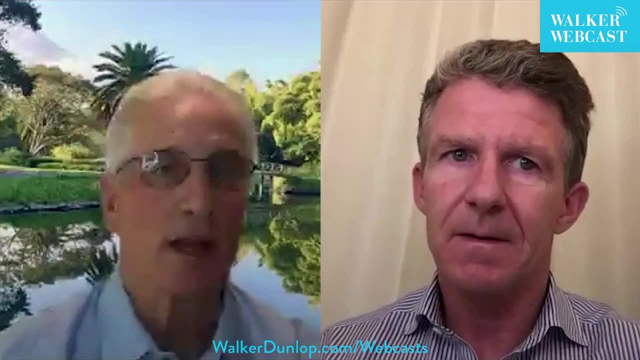 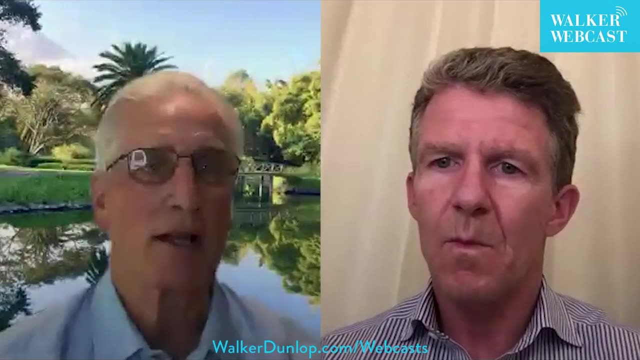 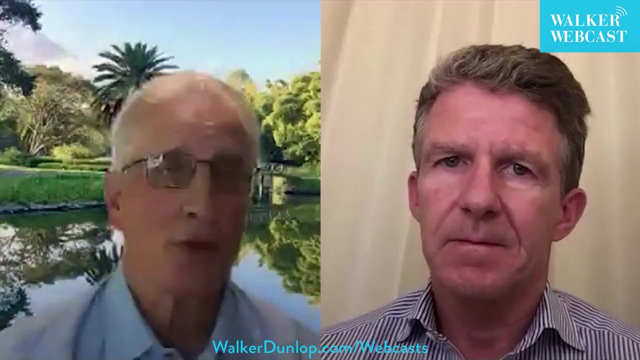 But the Fed doesn't have to read it superficially And in fact anybody with nuance looks at any piece of data and says: let me understand what's behind it. And, as you're pointing out, single-family true rental is not going up anywhere near. their number. But, even more fundamentally, two-thirds of all households own their home. If I say to a homeowner a very simple question: how much did your rent go up this last year? What are they all going to say: Zero. And that's one of the advantages of owning a home. You don't have your rent going up. It is fixed when you bought it. Yes, your gutter spout costs a little more if you have to repair it right. So for two-thirds of the households that own there, basically is zero inflation of their housing. 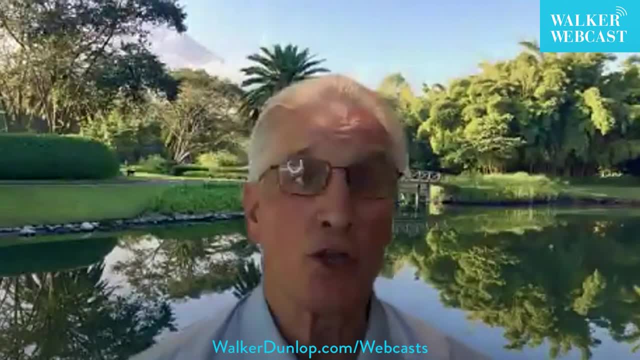 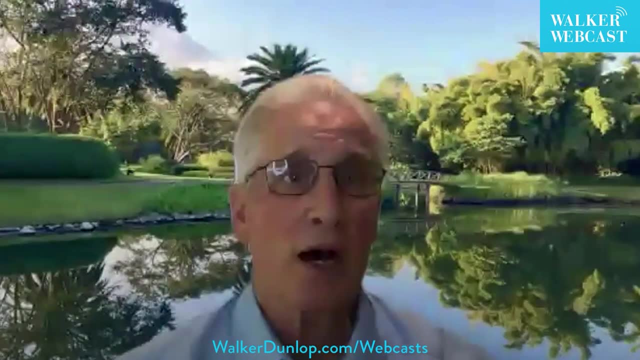 Then you go to the renters And on the renter side, you know this as well as anybody. I was just looking at what is it called The current market tenants. I see rent It's down. It's a minus 4% in the past month. Not up Minus, Not 5.8% up, It's minus. And of course anybody in the business knows rents aren't rising If you take the 3.5% inflation that they just reported this morning and you say: but I'm 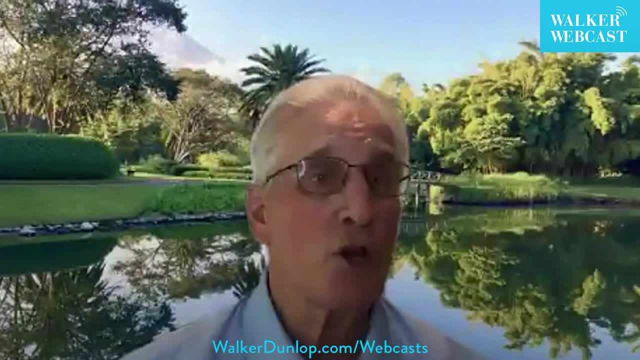 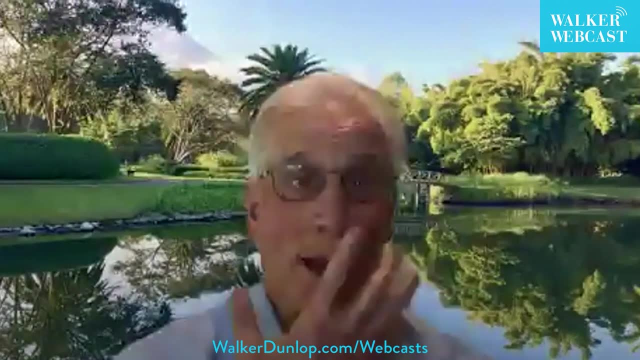 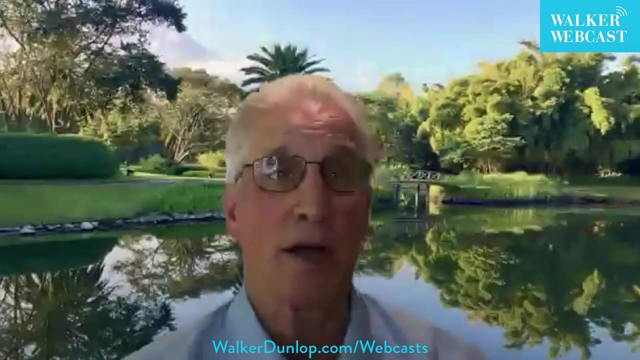 not going to take it at face value. I know Homeowners had no increase in their rental price, so to speak. a very small sliver, or single family renters. I put in your number and I know what's happening on the rent side at the bloodbath right now temporarily, and you're 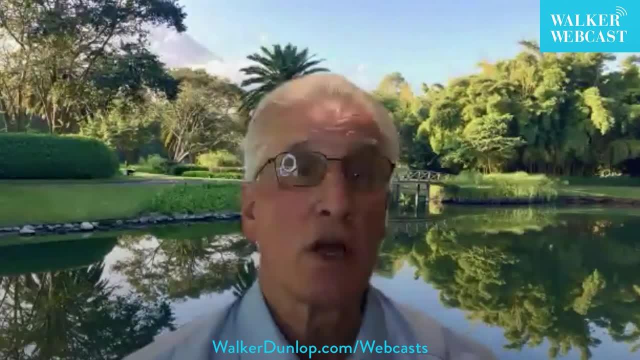 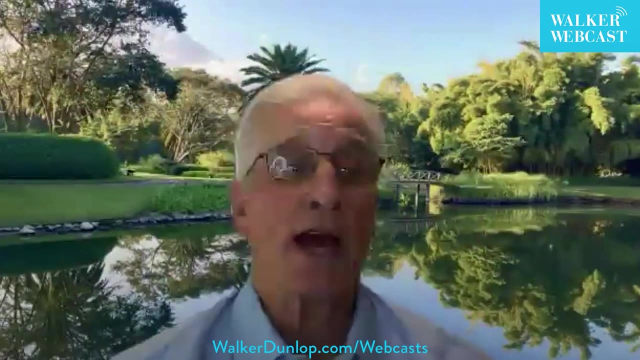 down to like a 1% inflation, which is consistent with what you were saying about food and this and that the other. you would hope the fed could do the math. that a couple of broken down guys. This is not rocket science and they don't get it. 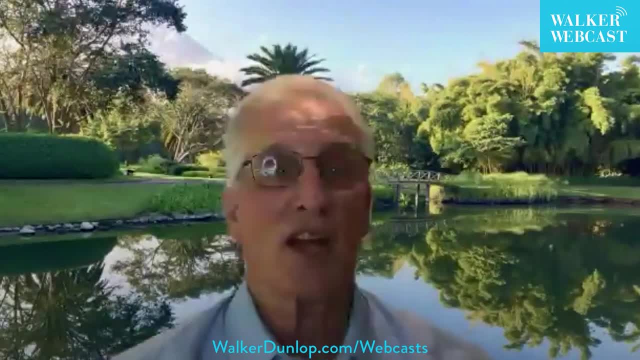 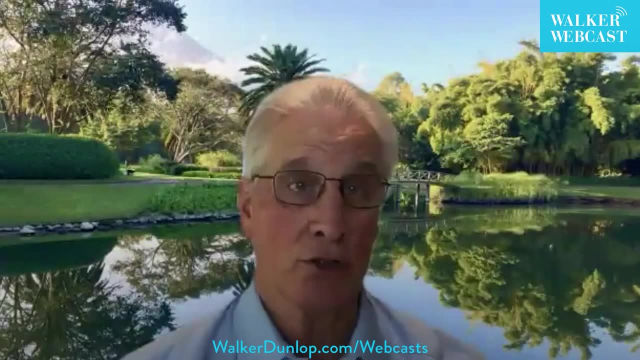 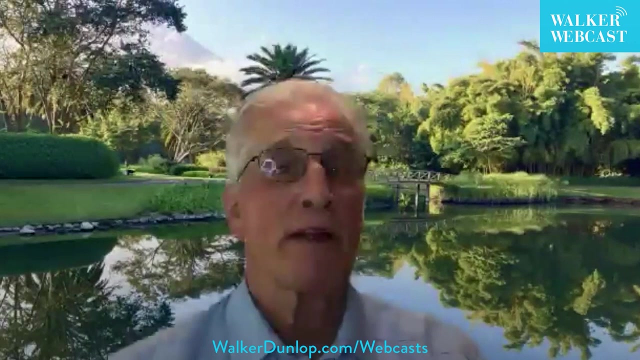 Even more so you would hope that if they saw essentially 100% of the inflation they identify is coming from one sector, That's not inflation in the economy, That's prices rising in one sector. So even if it was true That it was 5.8% in housing, That is causing that is the sole reason, inflation, and by that metric is above 2%, the sole reason. Wouldn't you think that you then say: well, we have whatever 75,000 items, and they all basically showed nothing, but one shows a lot of inflation, but they don't control that one, even if it really was that number. 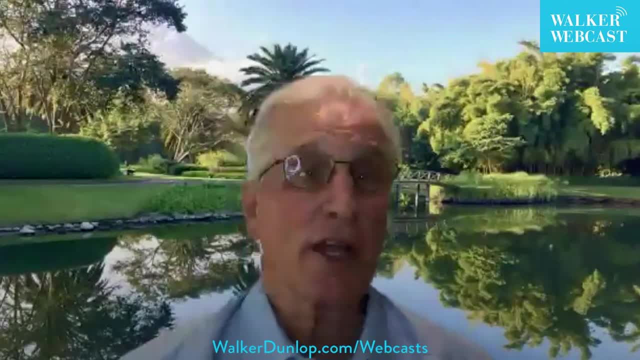 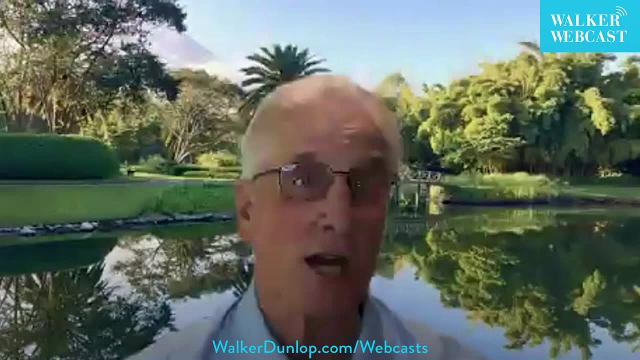 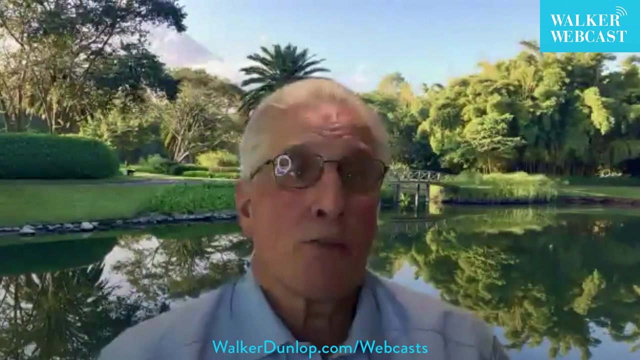 Which isn't So. it's baffling. Now, the problem the market has is when the government does dumb things, it has big repercussions. When I do something dumb, which happens a lot, it doesn't have big repercussions. But if you put me on the Fed and I was equally dumb, it's going to have big repercussions. 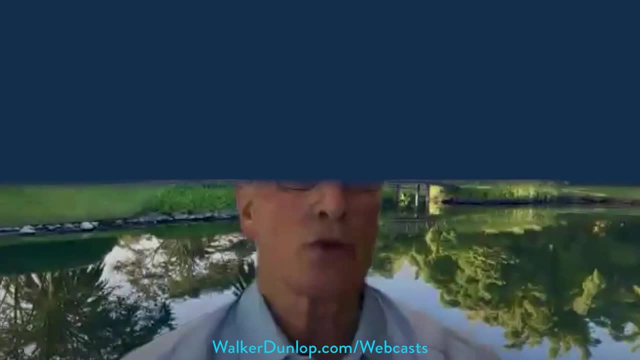 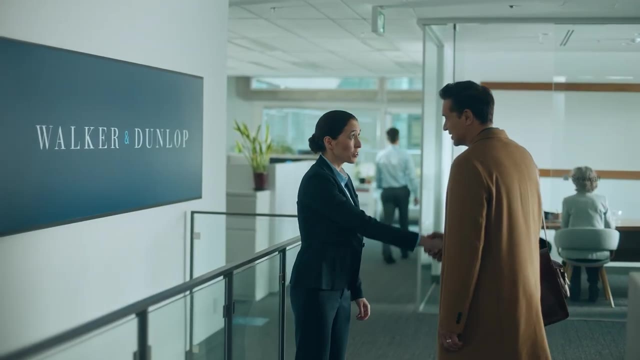 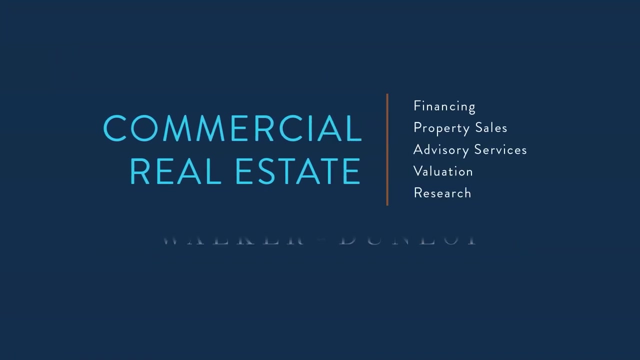 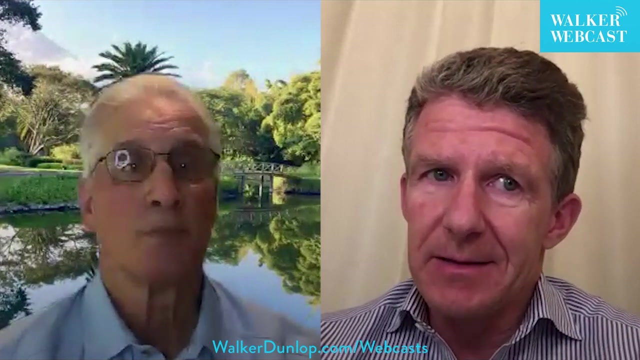 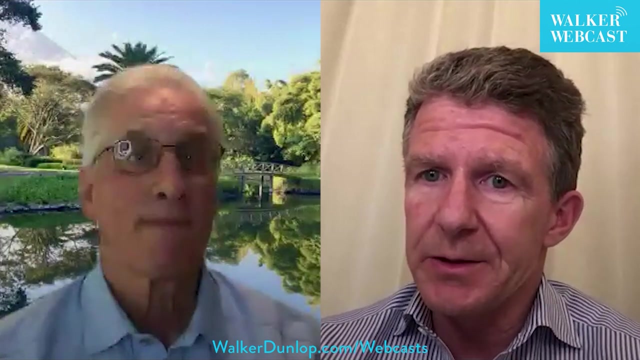 And so the market is trying to figure all this stuff out. Start A legacy, Start turning dreams into realities. A better world begins with you. Better communities start with us. So you have. you wrote in this quarter lever that you expect the Fed to cut 75 to 200 basis points in 2024. after today's print, 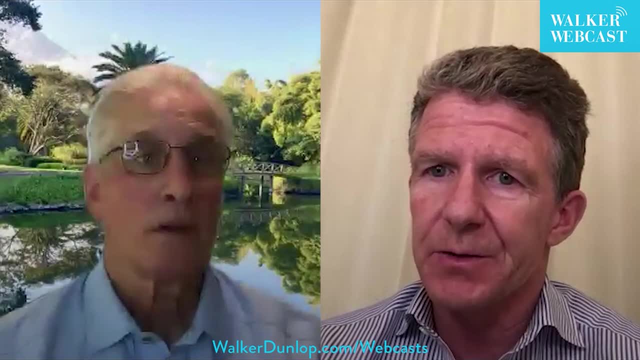 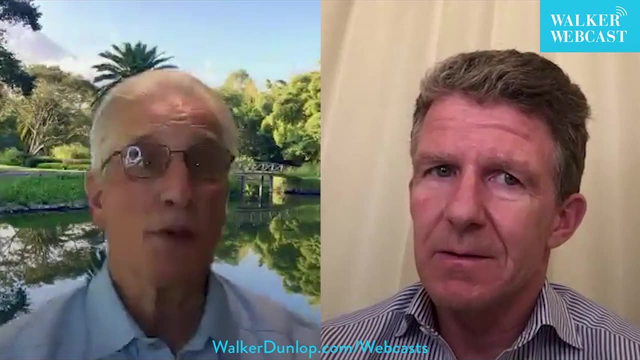 Do you still believe you got 75 to 200 basis points coming out of the Fed funds rate by the end of the year? Absolutely, For the reasons we just said. At some point they have to be smarter than just looking at a headline number. 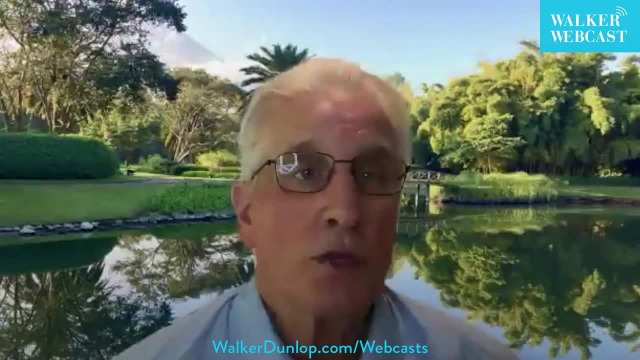 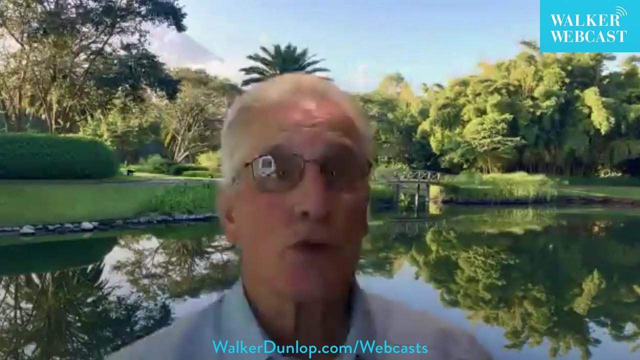 I mean we're, we're paying them all this money simply to look at a headline number. You mean they were supposed to be reading tea leaves and looking deep and digging. They have a whole staff. They have a whole staff of people, Don't you think again? 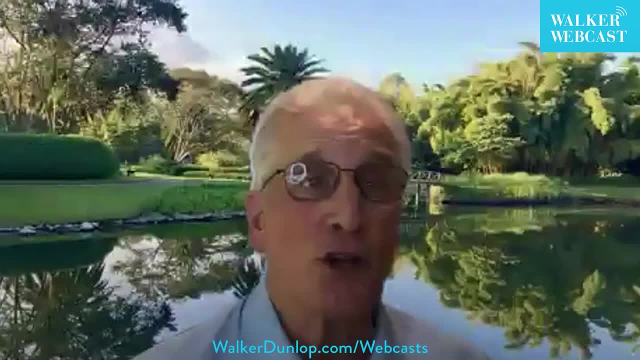 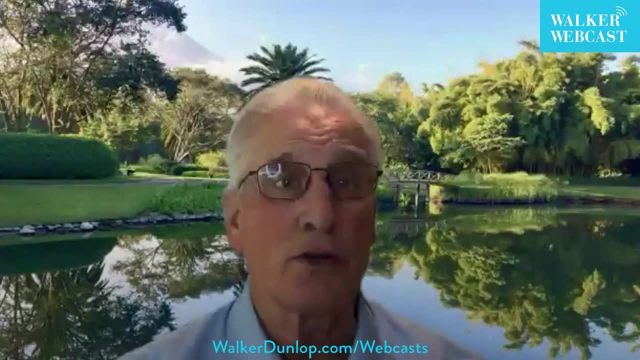 If the guys, If Graystar can figure it out, if the guys at Cortland, if a guy at Willie Walker Dunlap can figure it out, if a broken down retired schoolteacher can figure it out, don't you think a whole staff. so sooner or later they're going to see this. 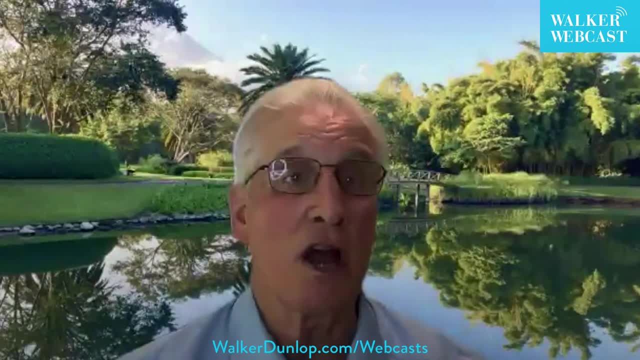 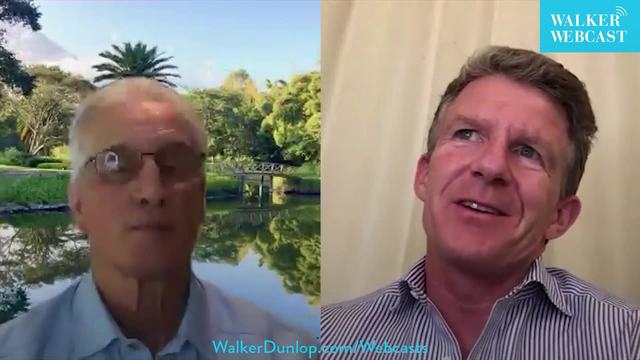 The good news is, most of the economy is not sensitive to short term interest rates. That's just my concern, But that's my big concern. I sit there and watch them and they say, OK, great. Well, you know what: The economy keeps going along. 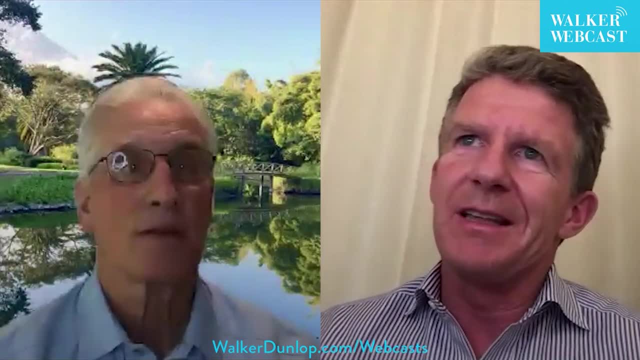 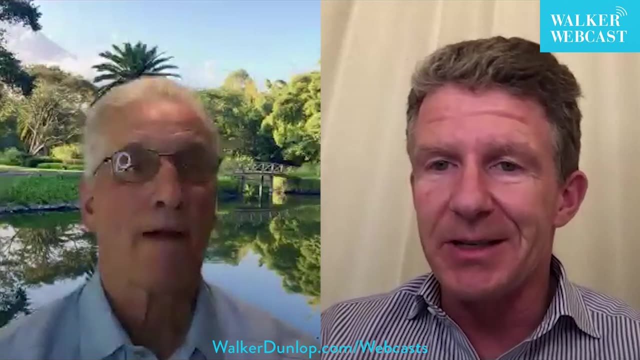 We keep adding 350,000 jobs. We keep you know. we see the GDP growth keeps going, The S&P keeps moving up. They sit there and say: OK, there's. there are these a couple industries which are very interest rate dependent: housing, autos, commercial real estate. 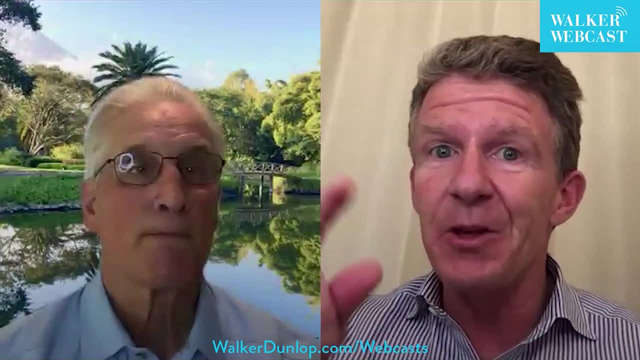 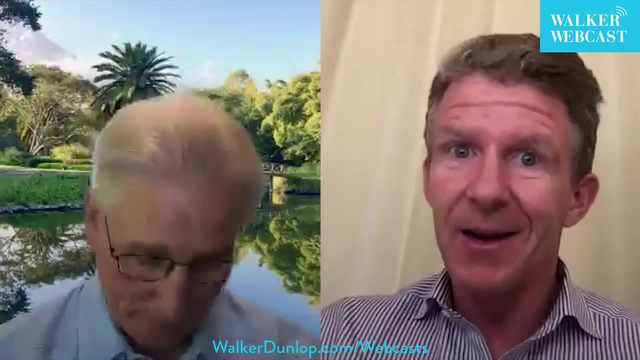 But you know- and, by the way, those are the sectors of the economy that you continue to underline as being the reason our GDP growth is lagging- I guess those are the two that you outline are. those are the two that you need to put more capital into, because that's where our GDP is lagging. 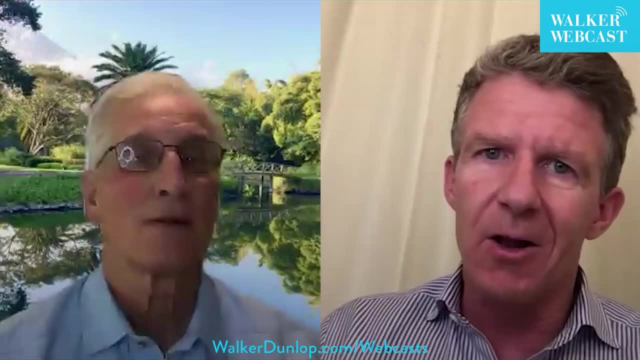 Yeah, But they say: but there are only 20 percent of the economy and the rest is all cranking along. So why do we need to do anything? Because we don't want to screw up the other 80 percent. They're captured by. 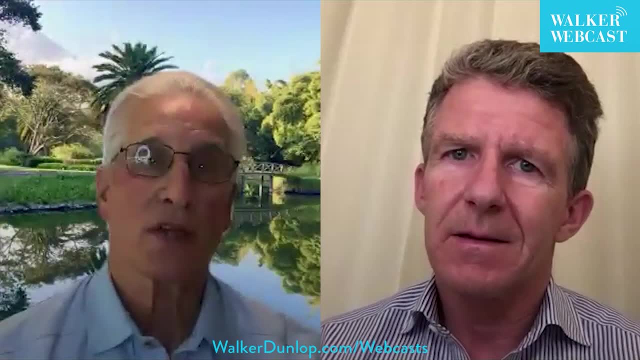 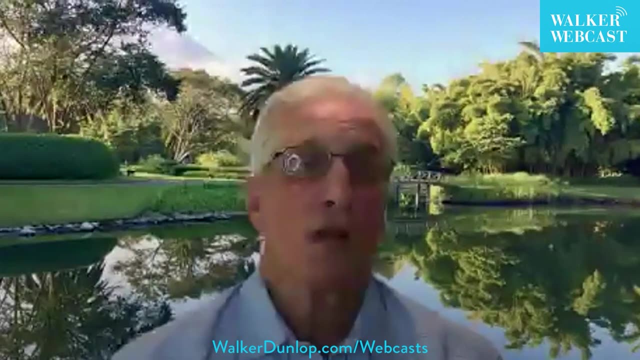 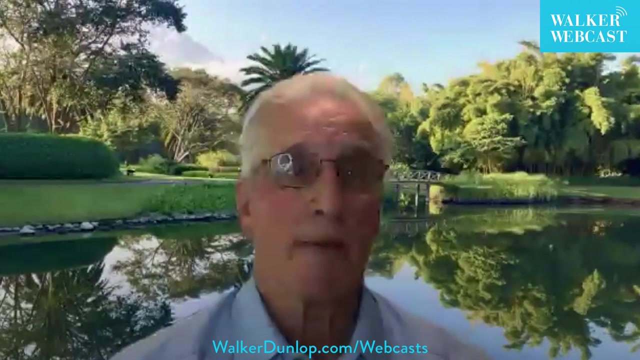 An antiquated model. they really are, if you think about it. and, by the way, everybody learned that model in school, which is you raise interest rates and everybody borrows less and they do less and the economy grows. The government's not going to do anything different because of interest rates. 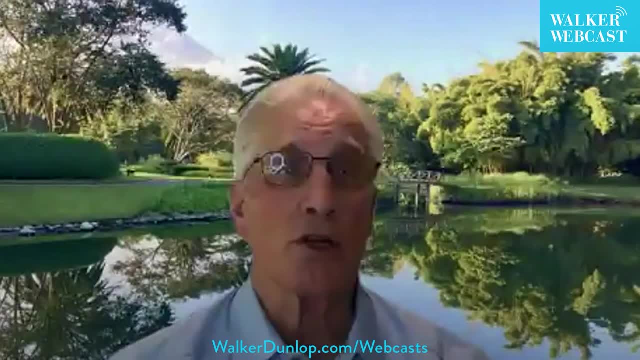 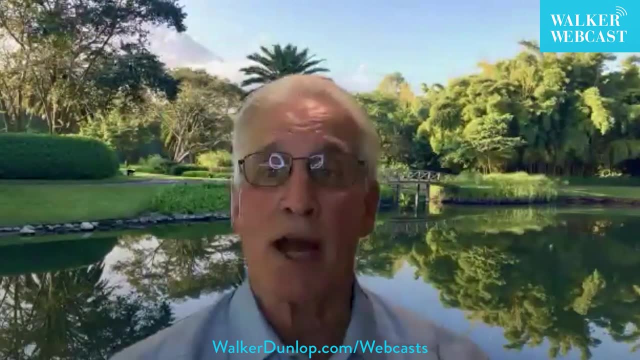 They might do Things different for other reasons. education: There's nobody saying, oh, the interest rates up, I'm not sending my kids to school. There's tomorrow. There's nobody saying I'm not going to have my baby tomorrow. in the health care sector: 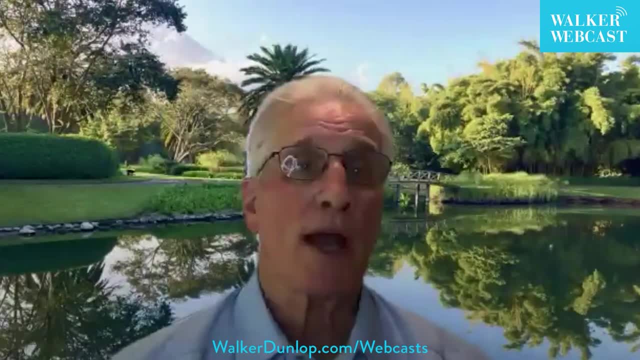 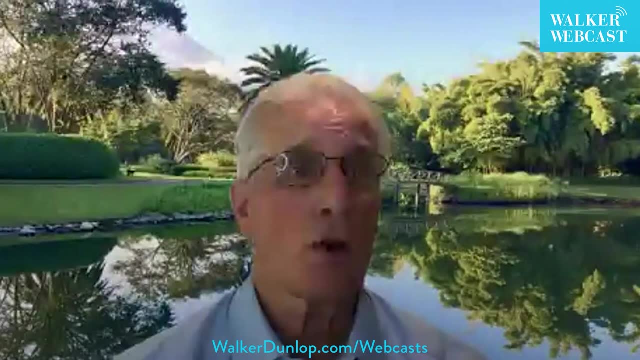 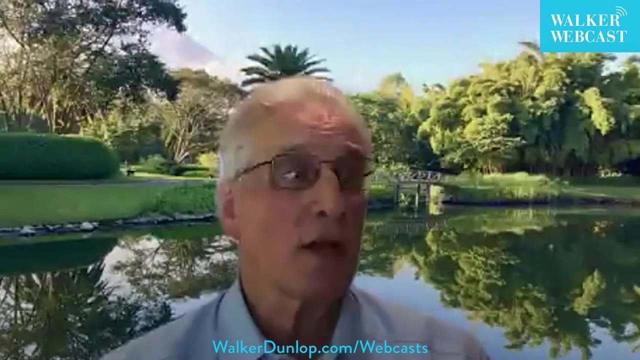 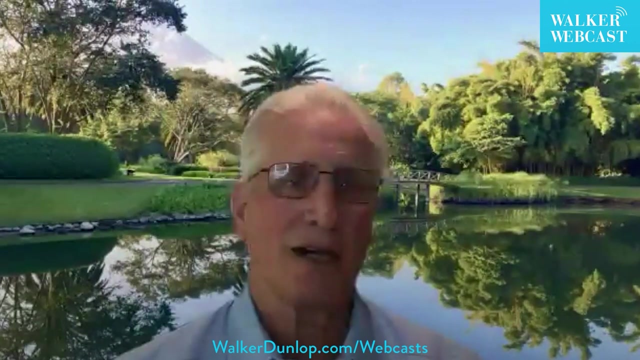 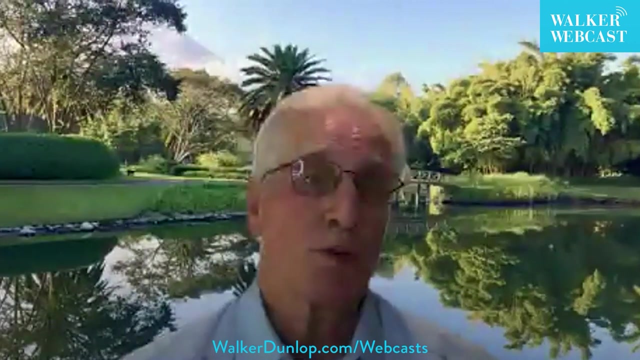 There's. so when you do education, health care, government, these are huge sectors of the economy, totally insensitive interest rates, totally insensitive interest rates. That's the mass of the economy. And you can put another sector. You're right, About 20 percent is interest rate sensitive. so you're essentially, they're essentially have this misguided view and, by the way, that includes, I think, there's a trade off between employment and inflation, even though all the data always shows there is no trade off between inflation and employment. 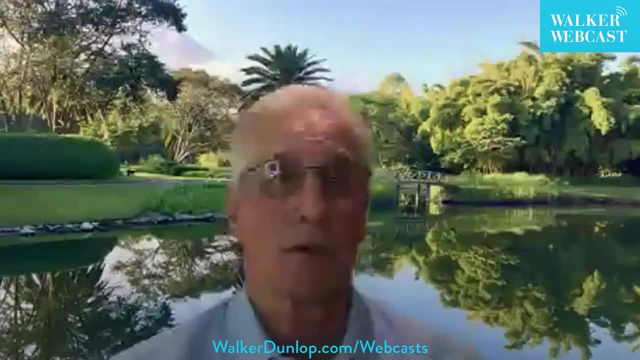 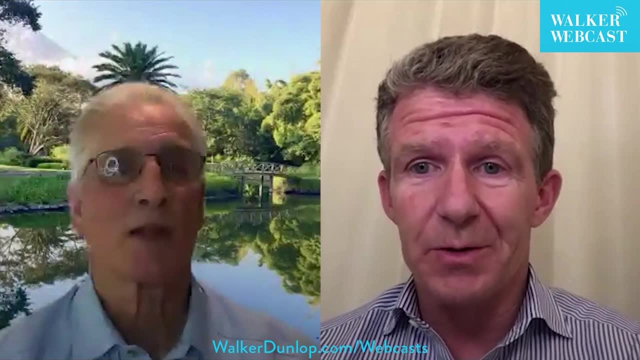 But other than that, these guys have got it pretty accurate. So I want to, I want to highlight one thing, which is just to remind you that a year ago, on this call, you said the Fed would cut by August of last year. 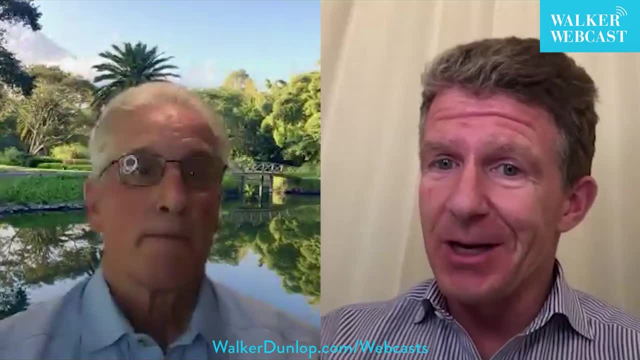 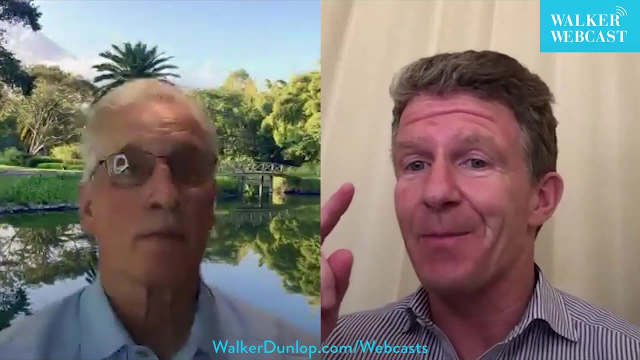 So let's be, let's be understanding here. You just said that you think they're still going to do seventy five to two hundred this year because they got at some point wake up. But it was a year ago now that you said they'd cut by August and we haven't seen anything up until now. 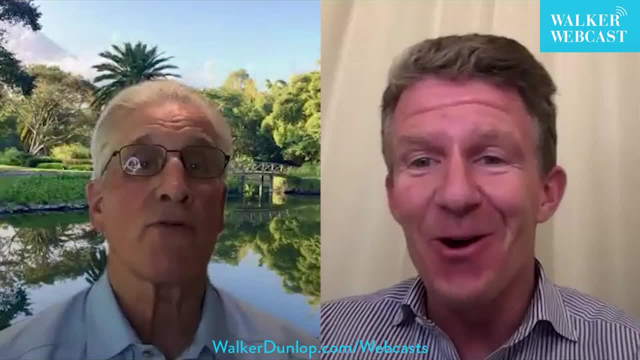 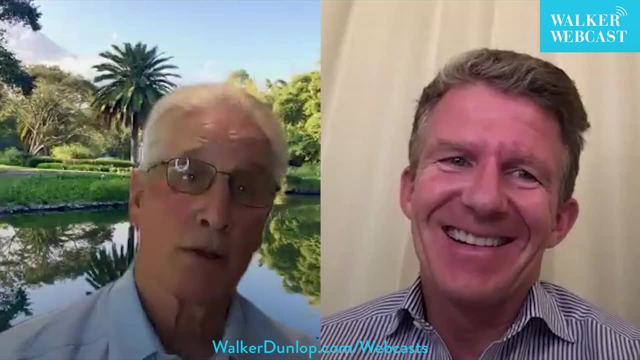 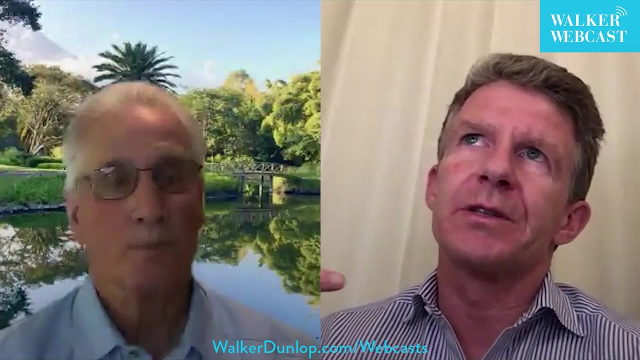 So I shame on me, You know I'm not going to No. no, Shame on me for expecting rationality from a government agency. OK, so let's. let's go into GDP growth for a second, because in, in your GDP growth. you're sitting there and you're basically saying you've got GDP growth of two point four percent in two thousand twenty four. 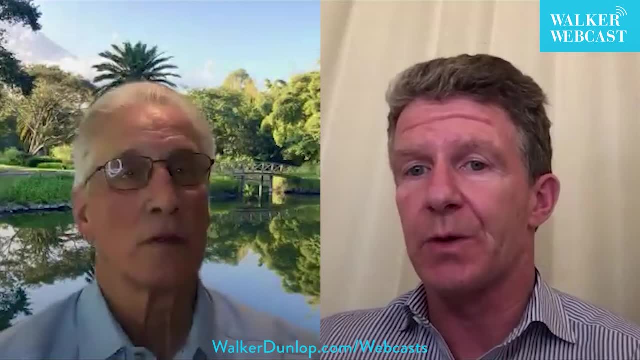 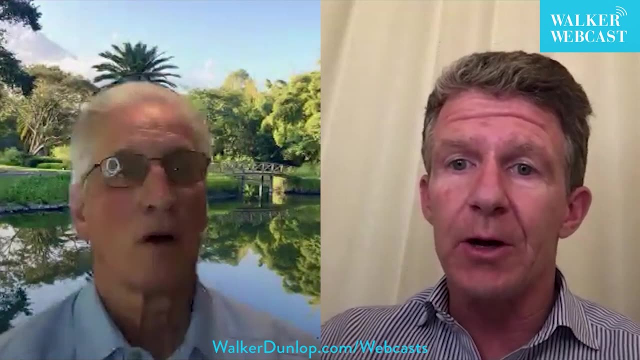 You've got GDP growth of two point five percent every year for twenty five, twenty six, twenty seven, up to twenty eight. But you- you put those numbers out there, Peter, pulling back your employment growth expectations. So a year ago you had adding three million jobs in. 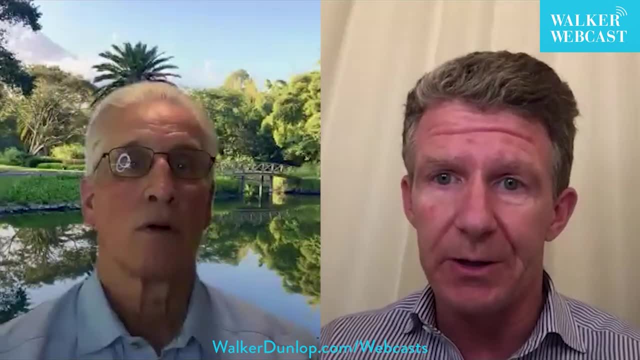 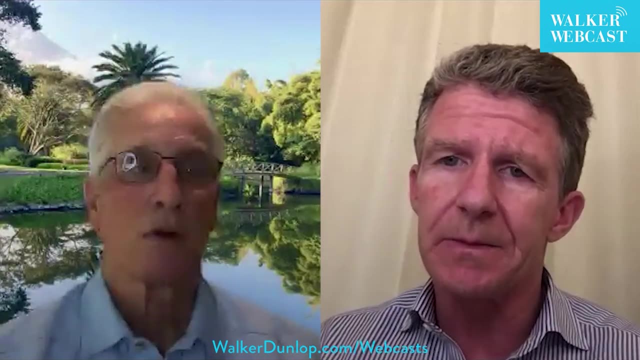 Twenty four and you peeled that back to two point two million jobs, And so my question to you is: how can you hold your GDP growth numbers steady, pulling back on the amount of job growth? you see in the US? We're- we're getting back to normal. 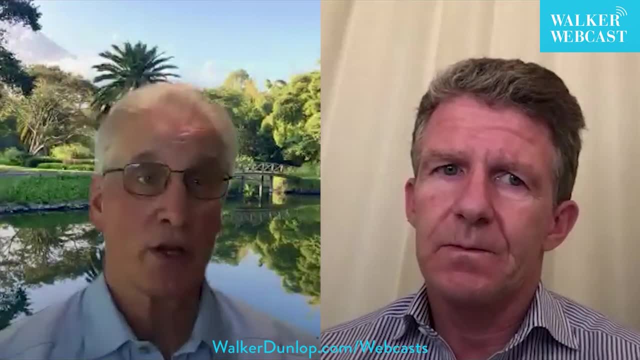 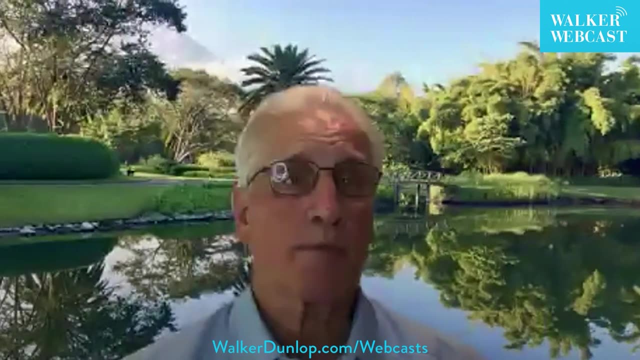 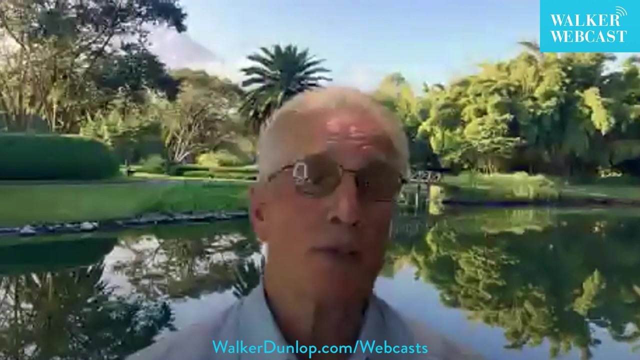 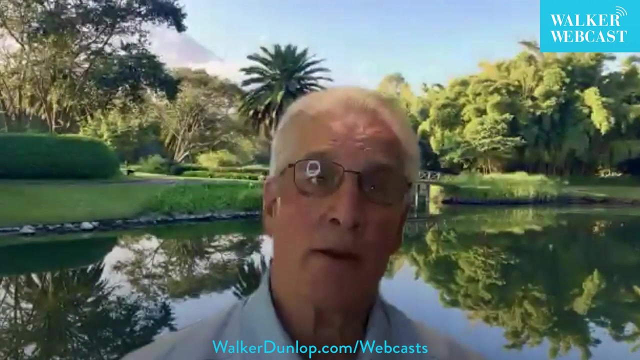 We, after this bizarre episode that covid and all the policies created, we're going to get something like one point five to two percent productivity growth and we're going to get something like 70 basis points Of population growth and, if immigration continues, could be higher than 70 basis points of population growth. 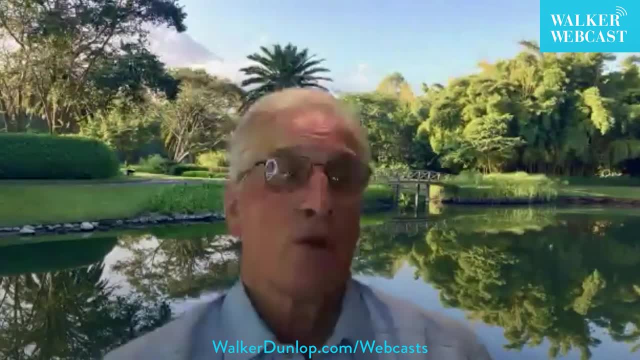 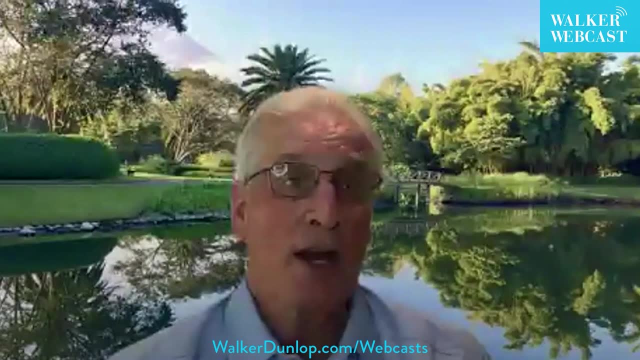 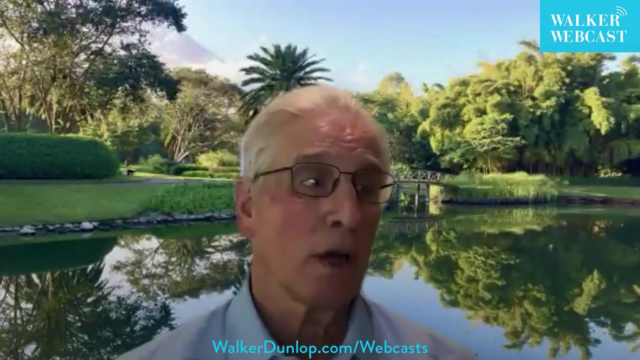 So that's kind of all you're doing is saying over the long term we have around one and a half percent productivity growth, maybe a little higher given some of the things going on, and add to that population, and population Population has grown more in the last. 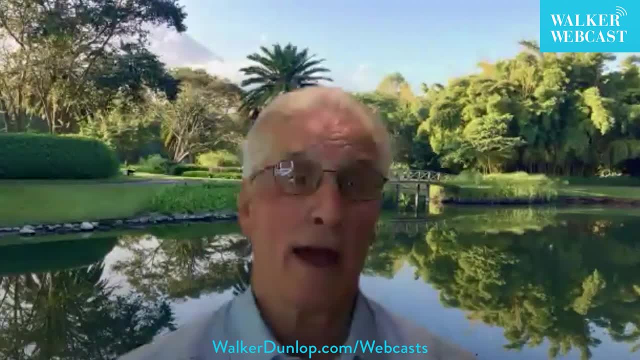 Fourteen months than people thought, And that's. you know, this is not a comment, good or bad. We're apprehending something like two hundred and forty thousand a month at the southern border. You know a lot, are getting in a lot. 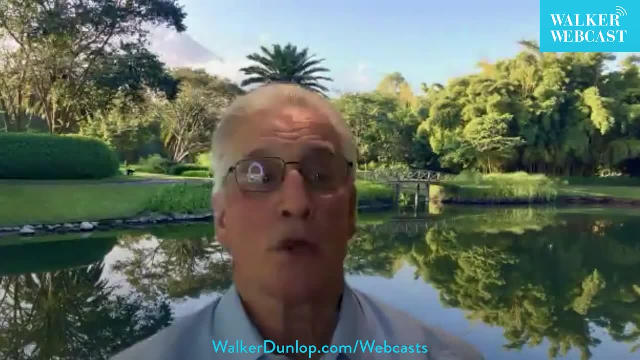 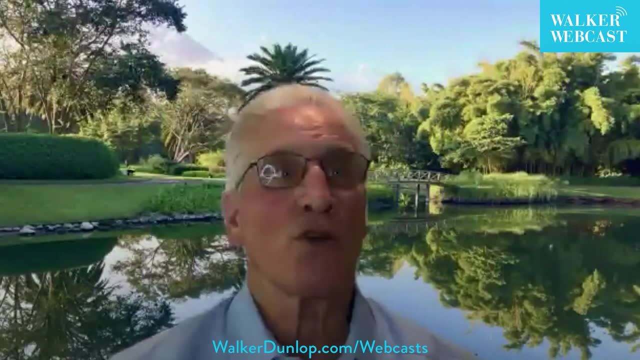 And so the population growth has gone up, and you're seeing it in job growth. That's why job growth is kind of looking stronger than you'd expect. But at the same time, how do you look at the population growth, by the way, of how much we've benefited from population? Couple of recent studies have kind of Not confirmed have supported that. Remember, it's very difficult to pick up immigrants and survey data because it's like a new business. I don't know who to survey. Right, I know who to go to if they're existing businesses. 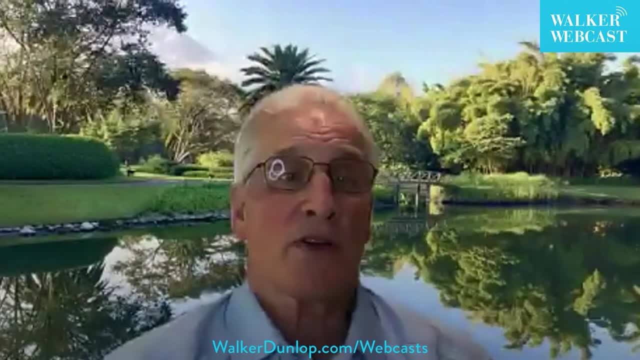 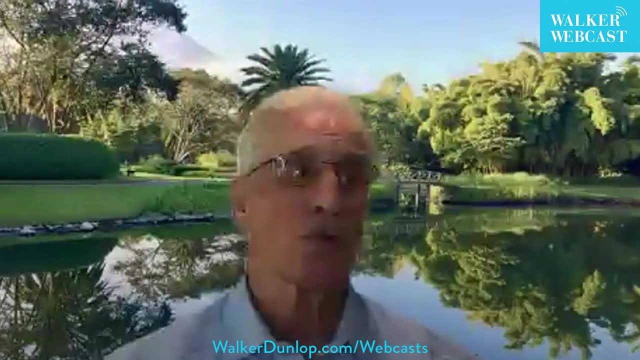 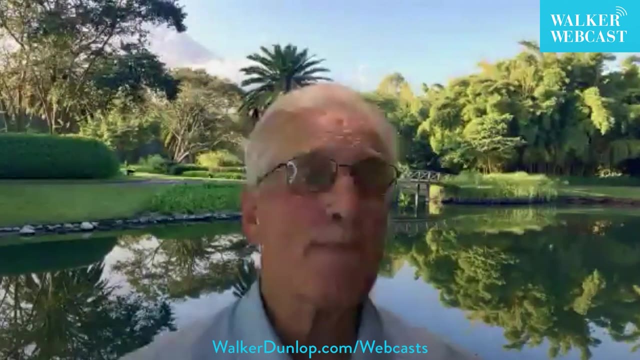 But to find the new business takes a while for me to survey them. Same with population. It's hard for me to give go exist, particularly if they're illegal. It makes it doubly harder, And so the surge at the border clearly has increased illegal immigration. Remember what a lot of this border surge is. It. has a lot of reasons, But remember when the pandemic hit and there were no jobs and no work going on here, if you were in Los Angeles area and you're illegal, why would you pay Los Angeles prices rather than go back home to your family, where it's a lot cheaper? So a lot of people went. back. Now they want to come back to where they had been, maybe for 10 years, and resume their life, because there are jobs again. They got to come back in illegally again. Now, that's not, It's not the only source of the surge, right, But some of it is people who had been living here for. 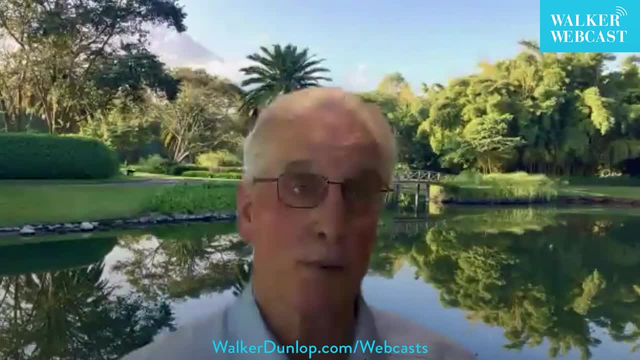 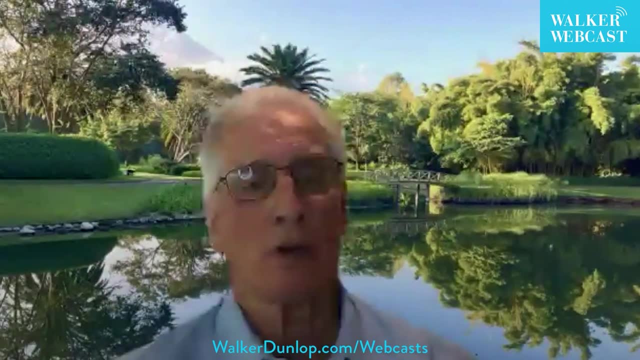 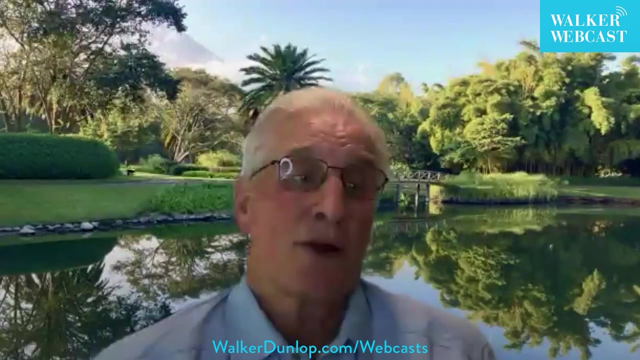 some time went back home because it was cheaper and there was no job here. Now there are jobs here. They want to come back and they're figuring out a way. So it's a complicated issue. I'm not trying to minimize, But I think we end up around 80 to 90 basis points of population growth and 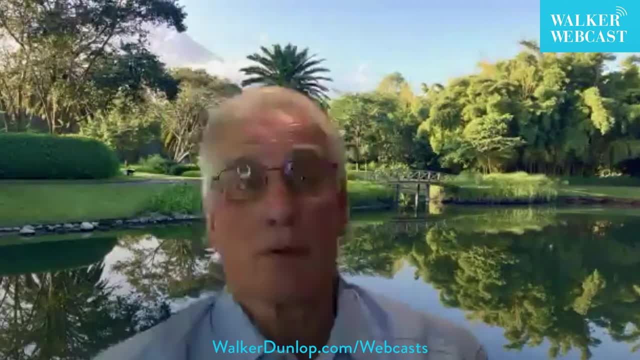 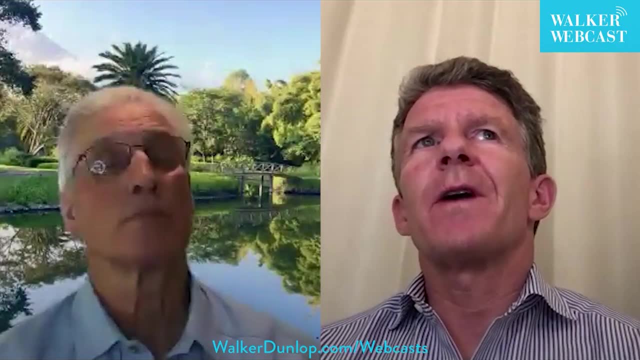 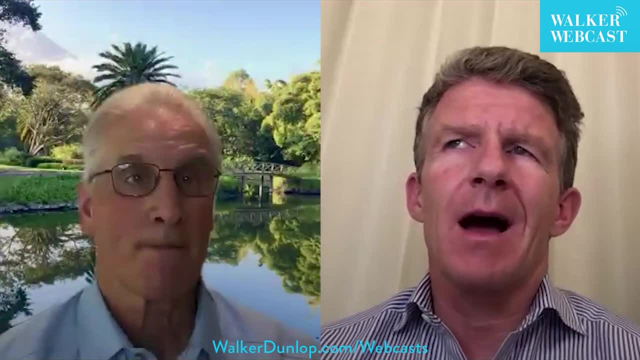 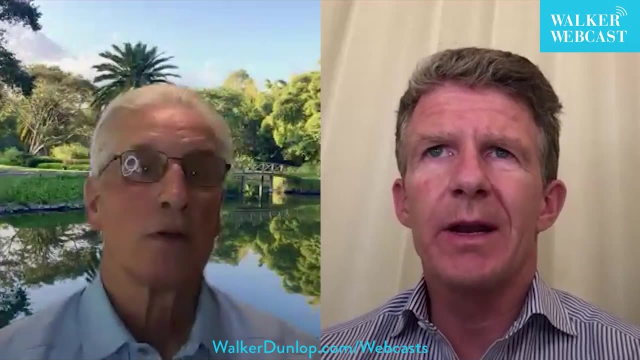 the sense of: are we going to get higher occupancy rates in multifamily because there are a lot of people here who need homes that haven't sort of been registered as being homes? Are we going to get a boost to GDP because there are more people driving economic growth, even though they're not? 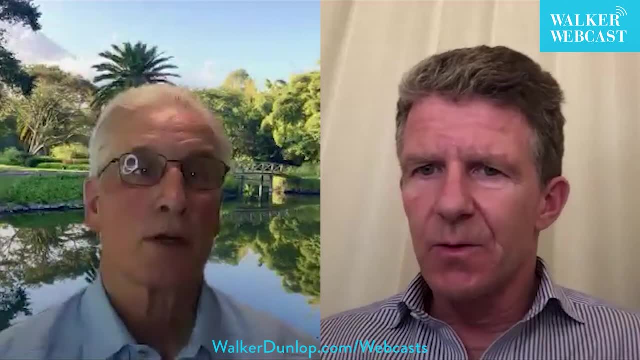 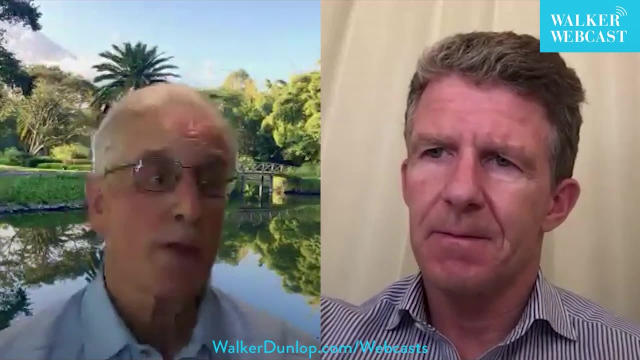 They don't show up in the actual numbers. I mean, where does this sort of show up? So it's a great question. Some of them, some of the illegals, show up, For example, if I go to an HR department and I ask how much- which they do with the payroll. 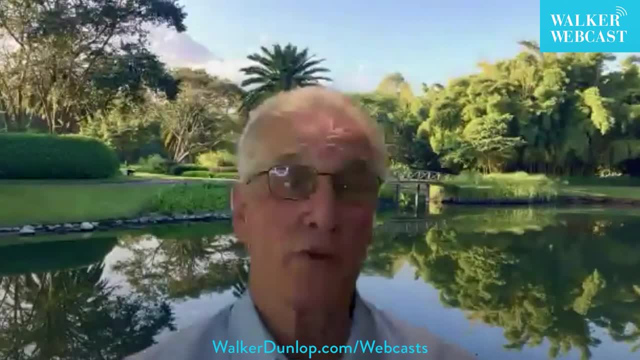 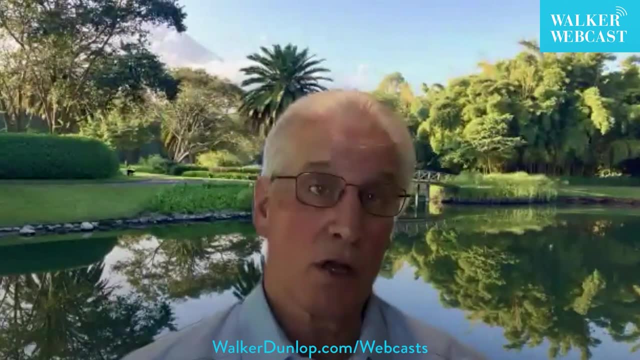 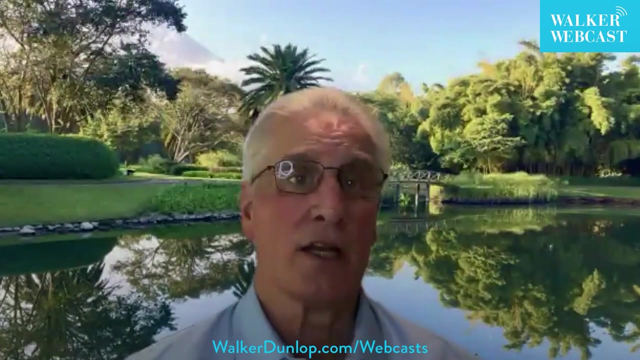 survey and I say: how many employees do you have? And they say: well, I've got 52,. right And okay. now four of those are quote illegals rather than two. So they show up somewhat in the jobs data, not perfectly, somewhat up to the sophistication. 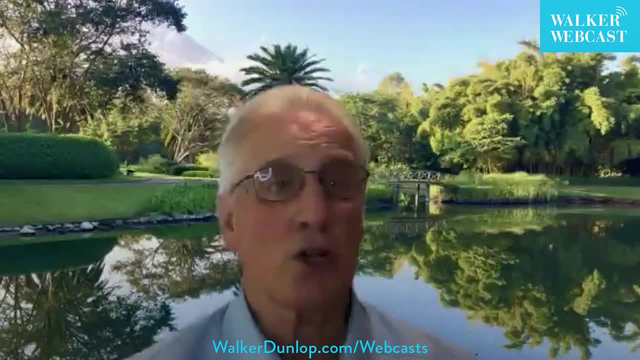 of the firm answer. They clearly show up in demand for apartments. They clearly show up in the demand for groceries, which, to your point, is GDP right. They show up in the demand for stuff that people do And it shows up in output. Because one thing we know about immigrants is that they They work at much higher rates than do native born, And so they show up everywhere. They show up everywhere in groceries and gasoline and so forth and so on, to push GDP. That's one of the great myths about quote: they take our jobs and they sit. 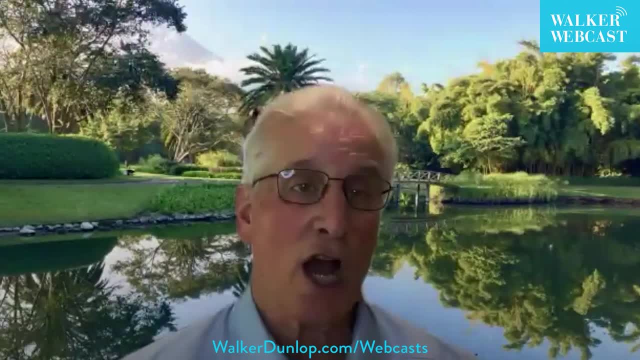 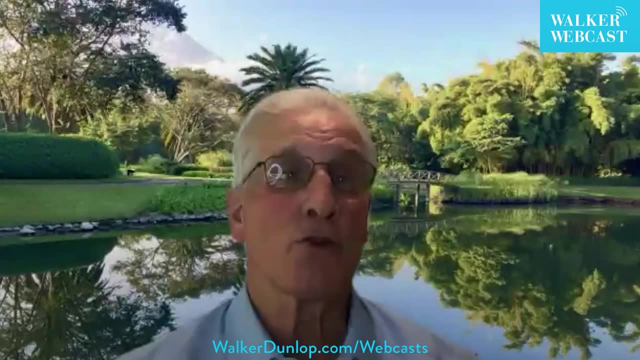 I always love it. People say: immigrants take our jobs and they just collect welfare. Well, take, Make a choice. They can't be doing both of those right, And the truth is they basically work, But they aren't taking our jobs. 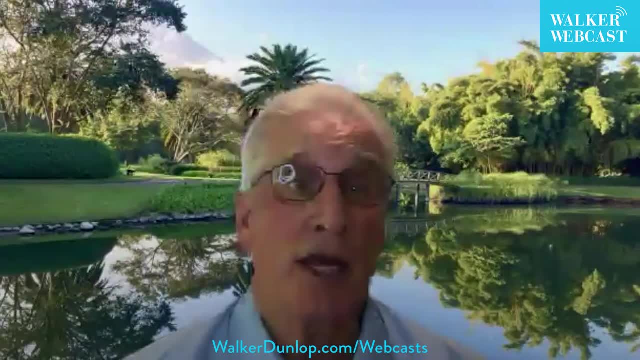 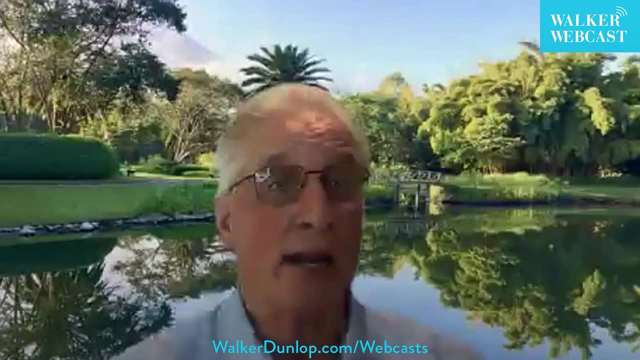 They're creating jobs because they're buying potato chips, They're buying shoestrings, They're buying glasses And that's creating demand for the people who make eyeglasses. That's creating demand for everything across. It's not a fixed pie. 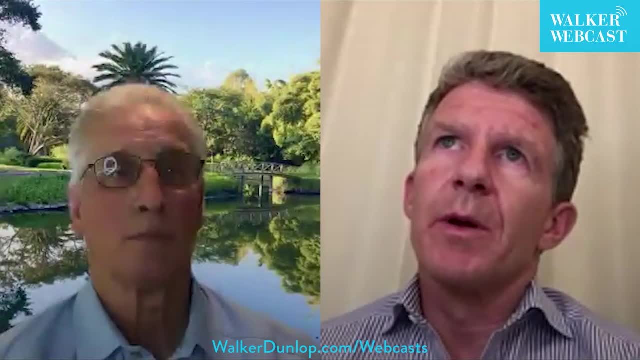 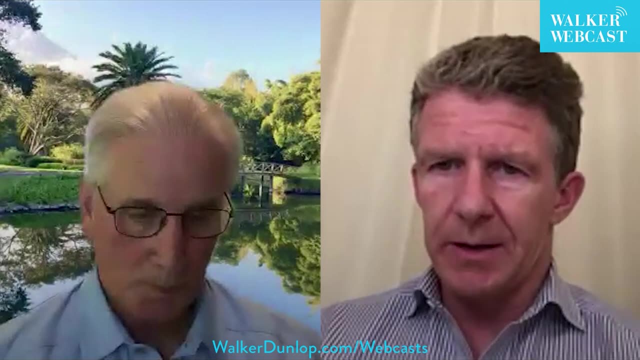 It's a growing pie. So go for a moment to employment and unemployment, Because I'm You're Your analysis. Peter has it that your unemployment rate is actually 270 basis points higher than the stated unemployment rate in the United States today. 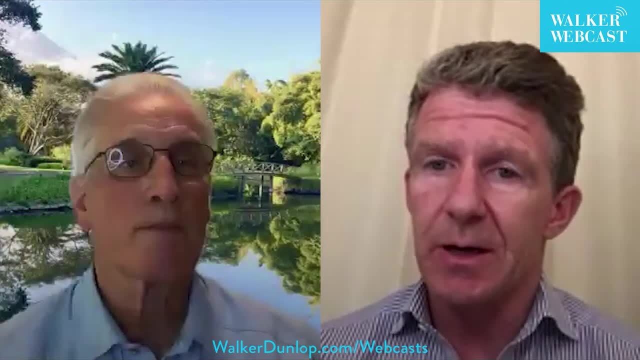 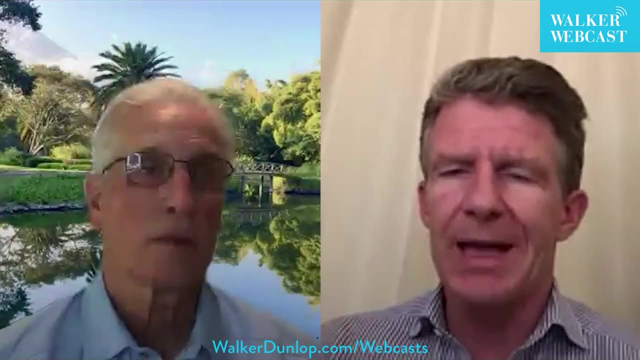 And so you've got right now a calculation of 6.6% unemployment versus the stated 3.5% of pre-pandemic- excuse me, and we're now at 3.8, I think it is in the actual number. 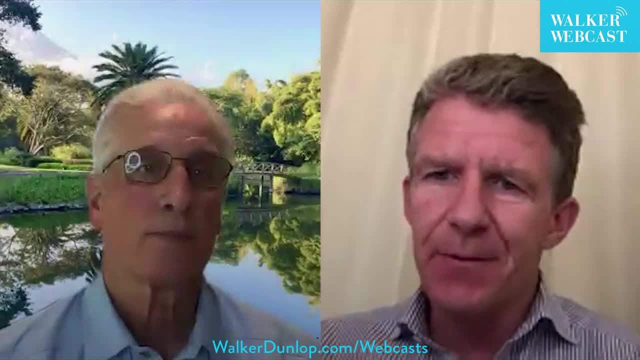 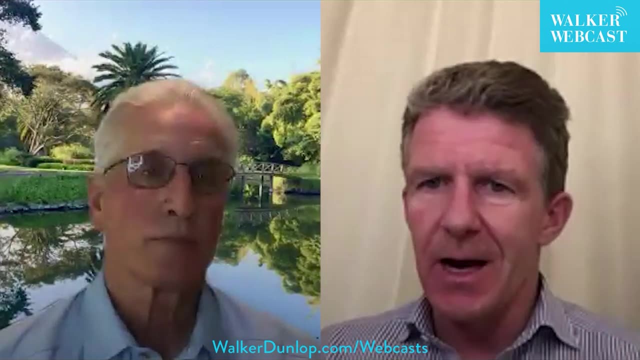 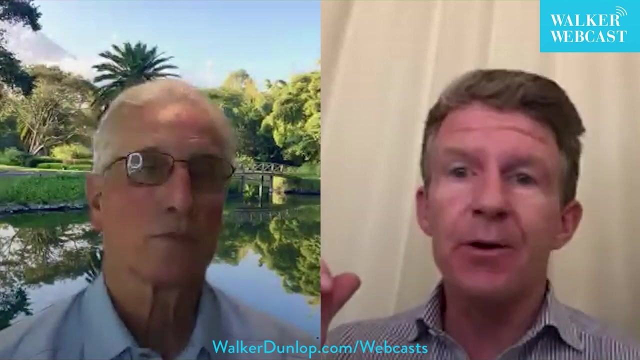 that's out. That's not a minor difference as it relates to consumer sentiment, Right? So one of the things that you track all the time is consumer confidence and consumer seminate, And one of the things that that number peaked at, I think, 132 in 2019, and it's now down. 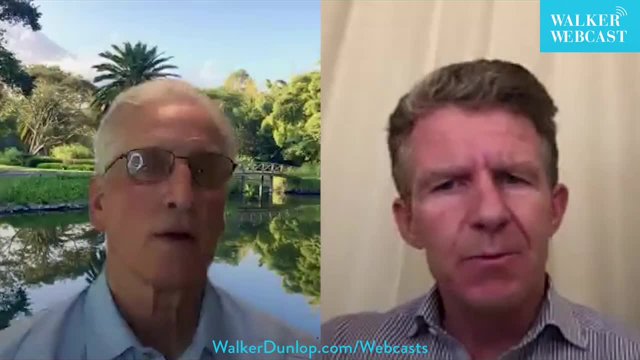 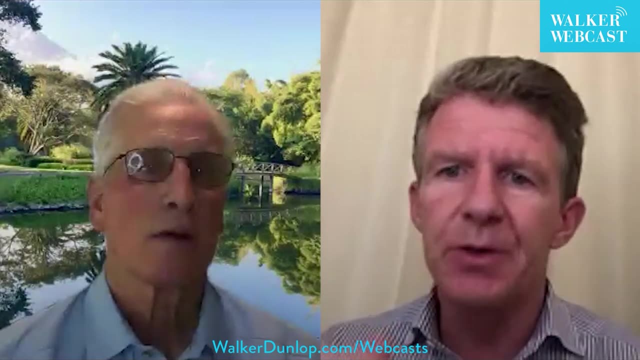 at like 132,, excuse me- and it's now down at like just below 100, right around 100. So the consumer doesn't have the same confidence in the economy today that it had in 2019.. And I keep looking at all these data points that talk about average household. 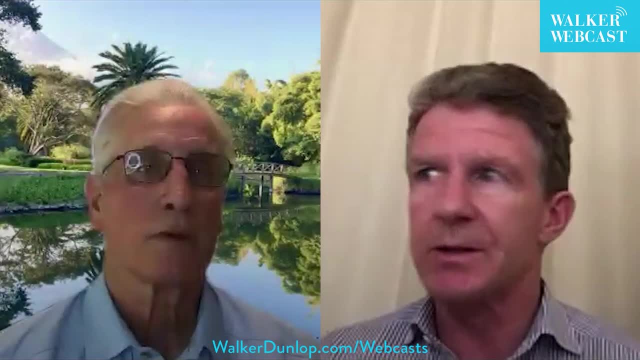 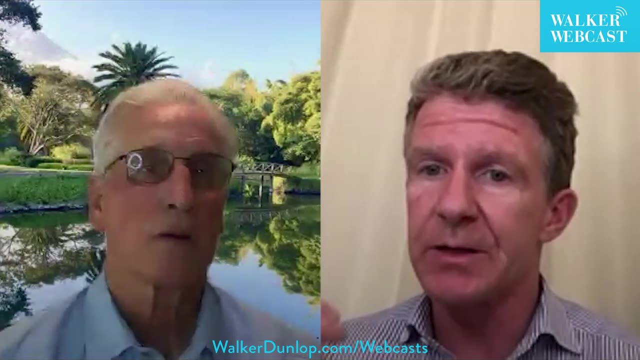 well, average debt burden, et cetera, et cetera. And you look at the actual numbers and you say consumer ought to be in a better mood today than the consumer was in 2019.. But that is not what the read comes out of the consumer confidence survey. 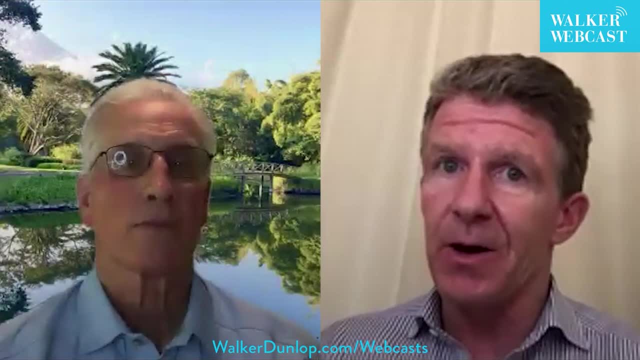 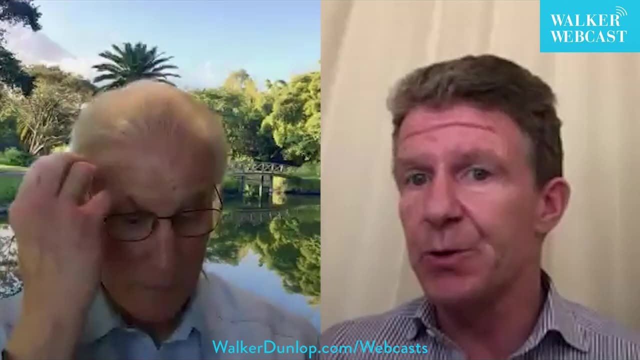 And one of the things that I keep thinking about in that is: is it that there are a bunch of people who are actually unemployed, who we're counting as employed or just aren't showing up in the numbers? and that difference between a 3.8% unemployment rate and a 6.6%? 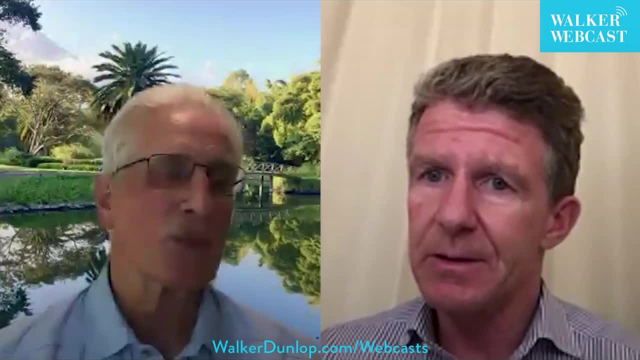 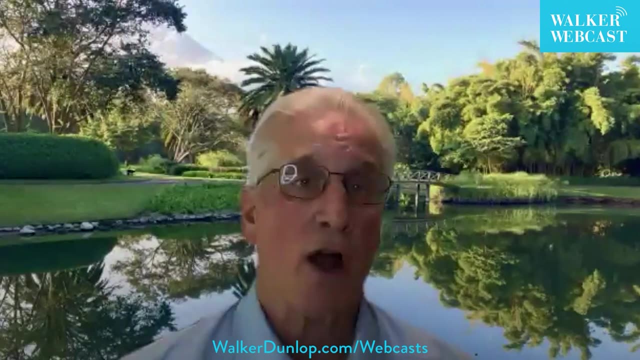 unemployment rate, because that is not a small factor. Not a small factor, It's largely people, People 62 and older, who just didn't come back to the labor force. They dropped out and they haven't come back to the labor force. 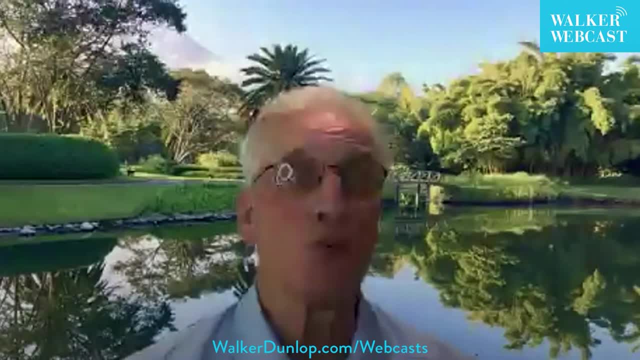 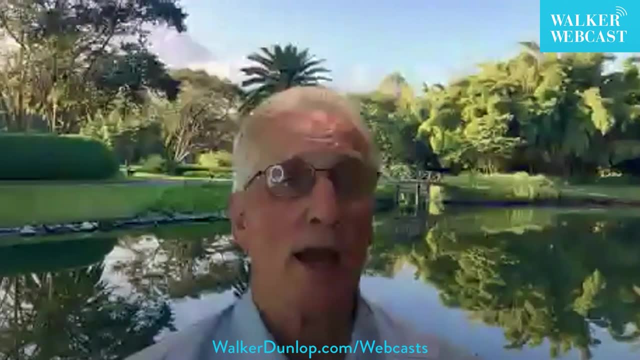 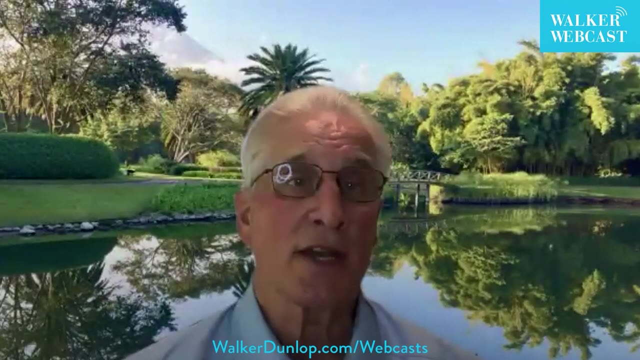 All the other age categories have resumed their pre-pandemic labor force participation rates. The 62 and over have not, And there's a lot of reasons, but they have not. That is the main source that we had Those workers that we don't have now that gap that you're referring to, the labor 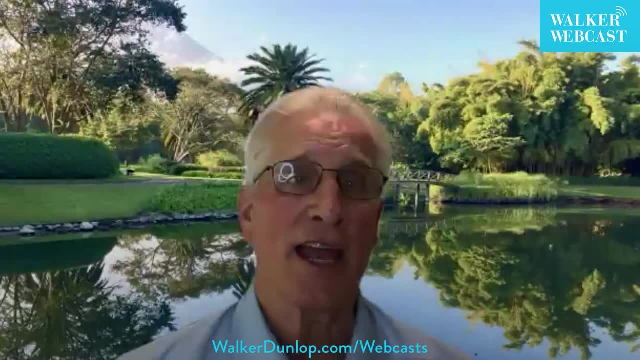 why are people not as happy as they? quote should be right, And you know there are a lot of reasons, but I think one of the simplest is: we're still below trend. We're still below trend And if you can be going 50 miles an hour on an expressway, which is an amazing- 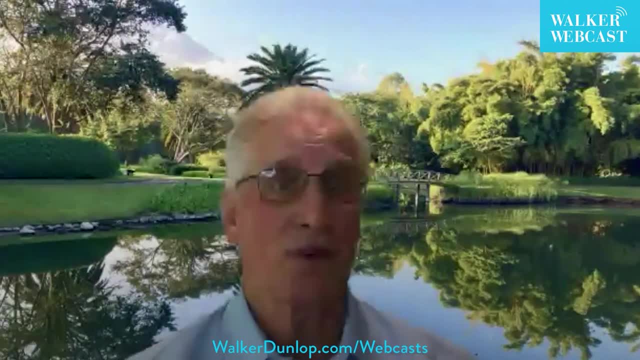 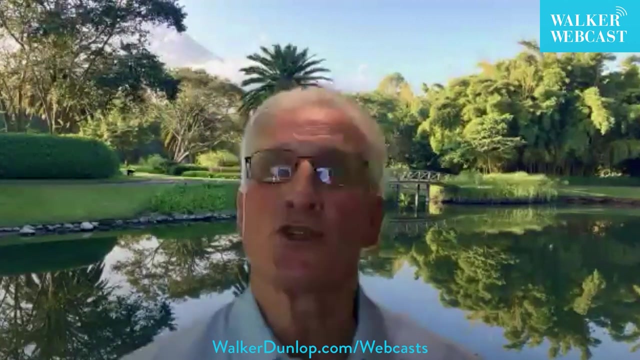 amazing speed in the context of life to be able to go 50 miles an hour. but if you believe you should be going 70 miles an hour, it feels you're at a crawl, right Even though by you just got back from India. the notion of going 50 miles an hour is stunning. right, if you're in India, It doesn't happen. And so that's what's happened. GDP is still about a percent and a half below trend, Employment still A couple of million below trend. That is to say that, yep, we're at higher levels than pre-pandemic, but we're not going. 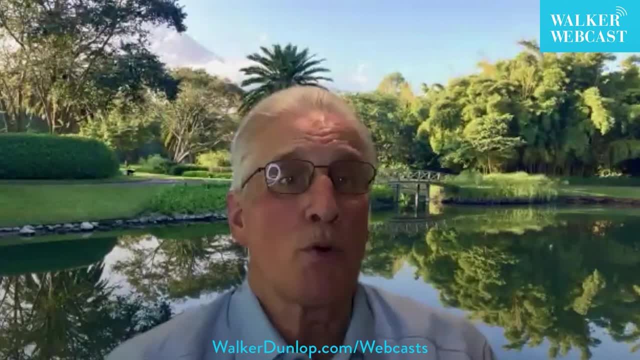 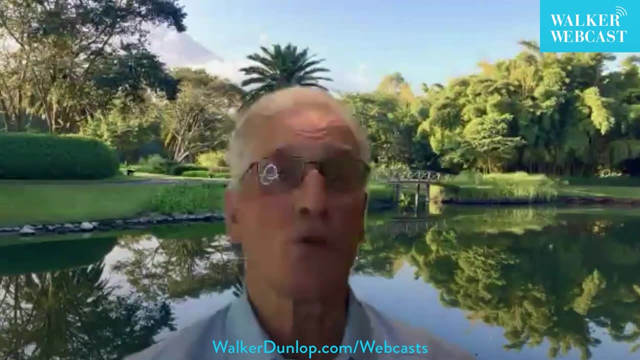 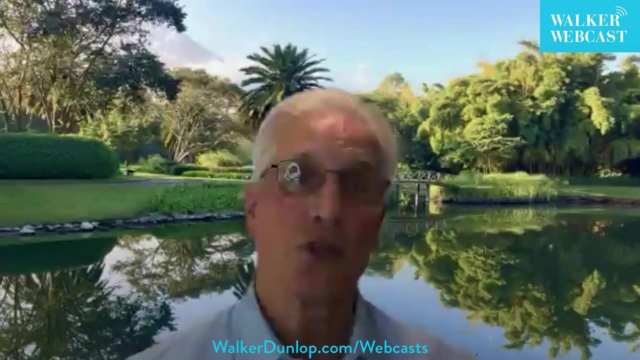 the speed we want to be going And you get used to growth And so I think people got used to a degree of growth. Yes, they are better off If you. so it depends what question you ask, right, If you kind of pose the question: are you better off than pre-pandemic, the generic? 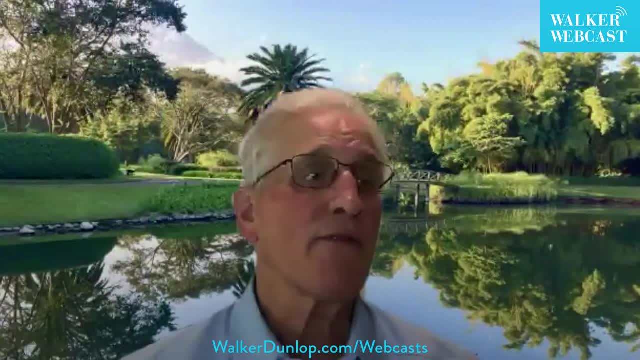 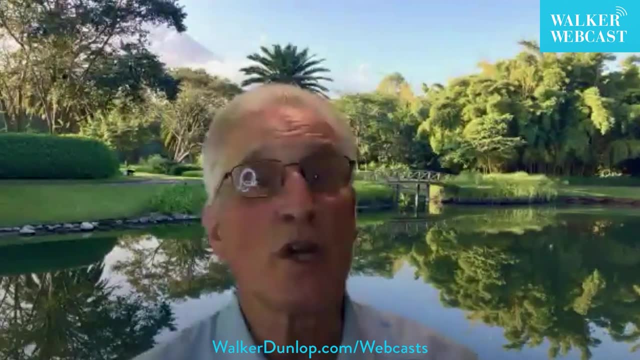 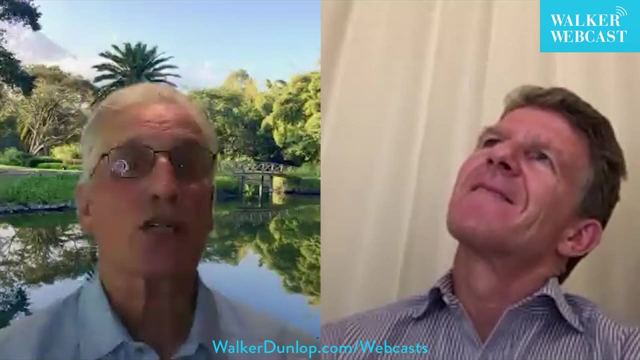 answer is yes For more people than not. If you say: are you as much better off as you believe you would have, as you believe you would have been, And the answer is no, I'm not. And expectations are important in life. 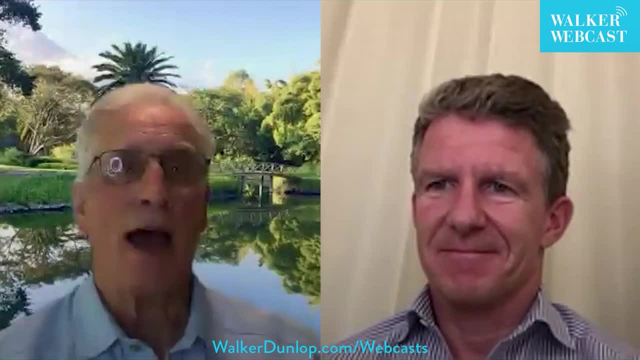 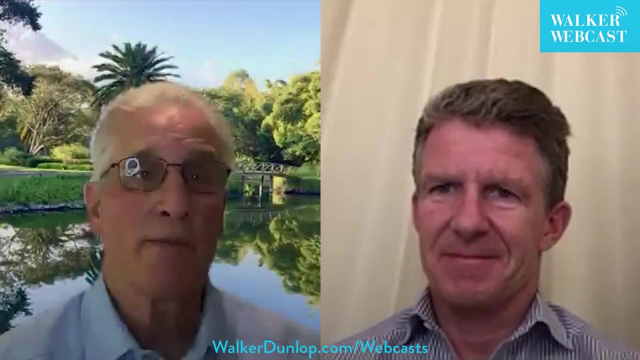 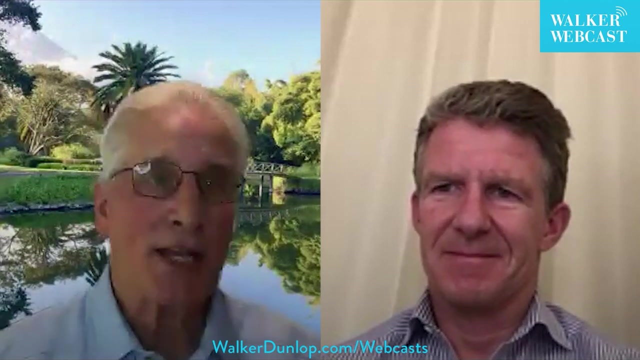 Now, do I think people in their head, or? I'm not saying, they've got a mathematical question, mathematical formula, but they all had expectations of where they would be in four years, In 2019, they all, not all. they basically, though, are all better off than 19, and yet, 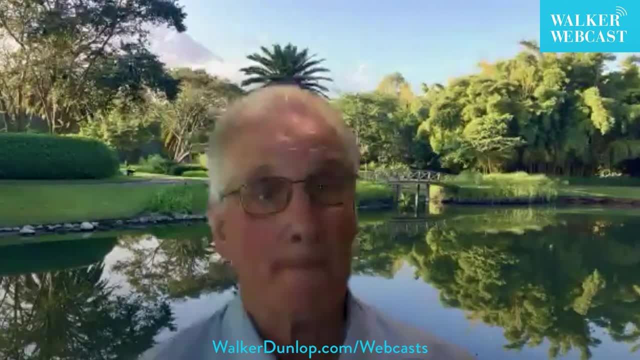 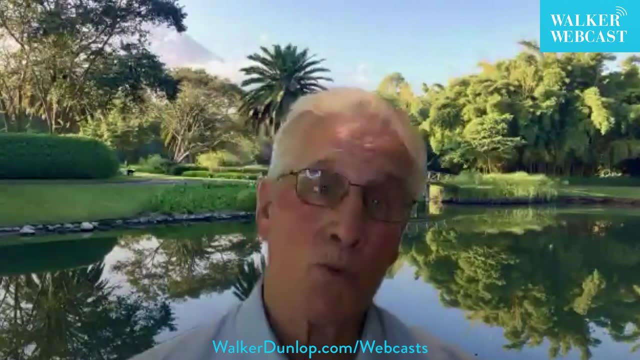 short of where they thought they would be okay, And not every individual. So that if I ask you, are you happy? Well, at one level, yes, And if I ask you, are you unhappy? The answer is yes, I should be even happier. 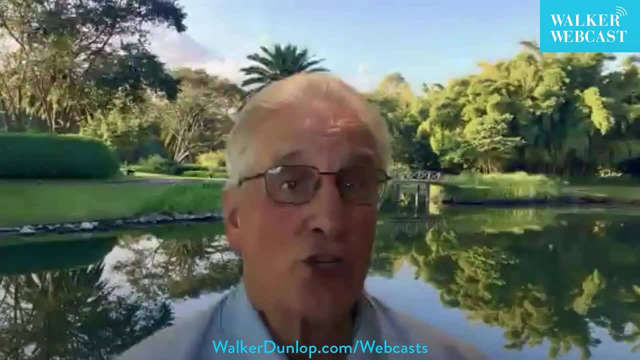 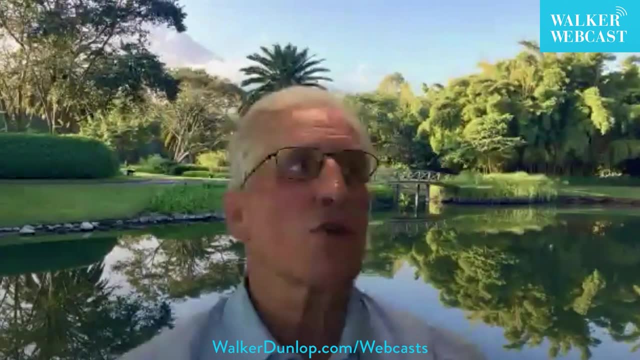 And, by the way, I have reason to believe I should be. It's not like a crazy. I should have won the lottery right. This is just a trend, pre-pandemic trend. So if I had the intellectualized and then you threw in all the geopolitical and all, 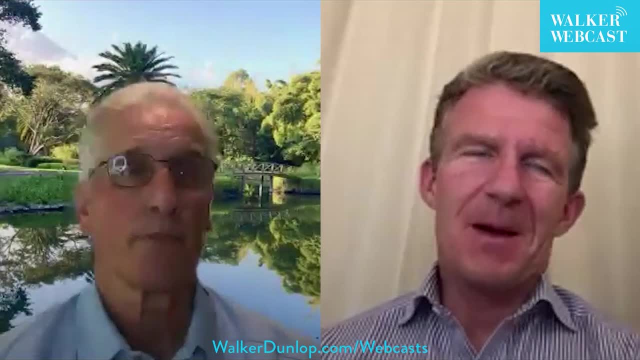 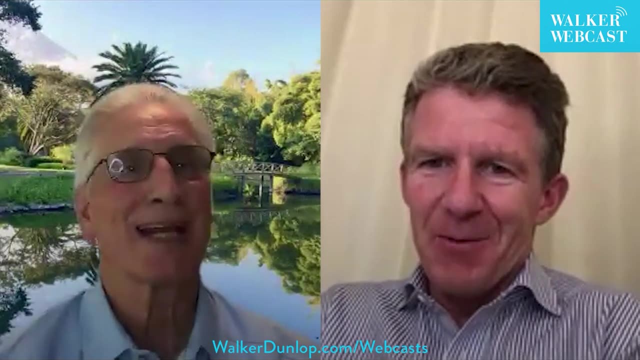 this kind of stuff. yeah, it's not so surprising. Yeah, You mentioned happiness and how happy people are. As I told you at the top of the call, I was with the Dalai Lama yesterday and the day before, And so, to everybody who's watching this call, happiness to you all. 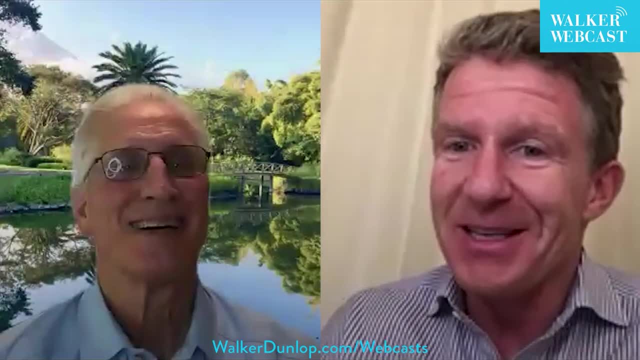 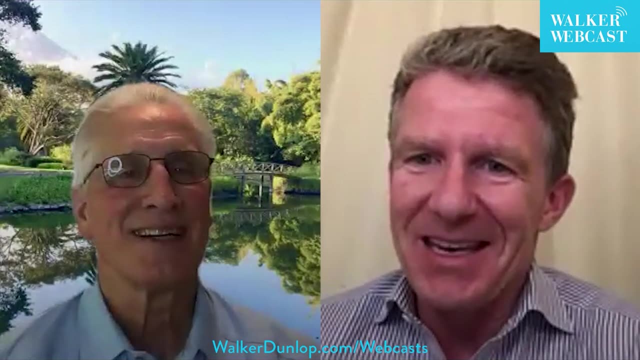 I've been getting a big dose of happiness from His Holiness Himself over the last two days, And it was really quite an experience to be in Dharash Lama, India, with the Dalai Lama. But, Peter, let me just one other thing that I thought was interesting, that you pointed. 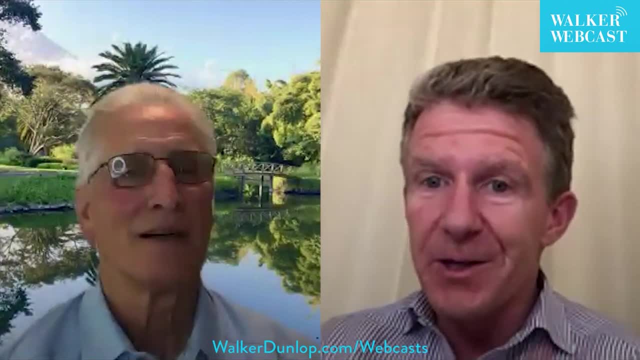 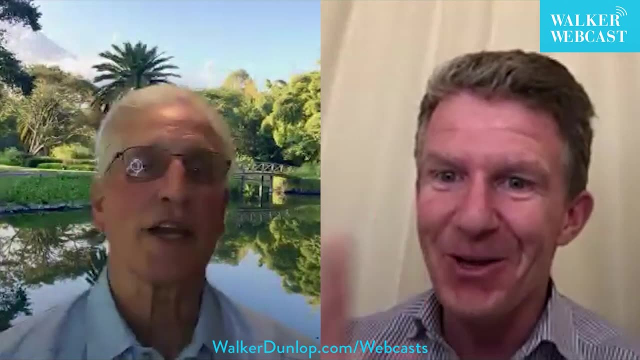 out in the letter was to go back four years. So four years ago this week, four years ago this week, 6.1 million Americans filed for unemployment. 6.1 million, okay. And then- throughout 2020, we had 1%. 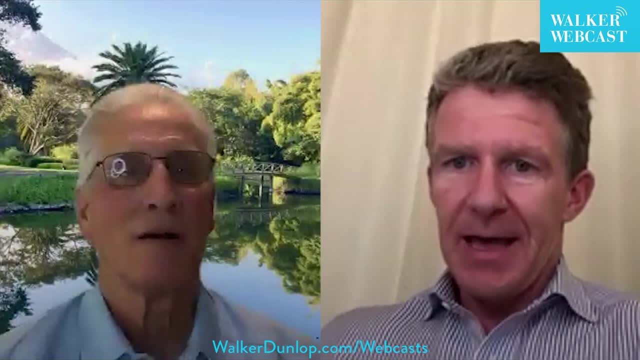 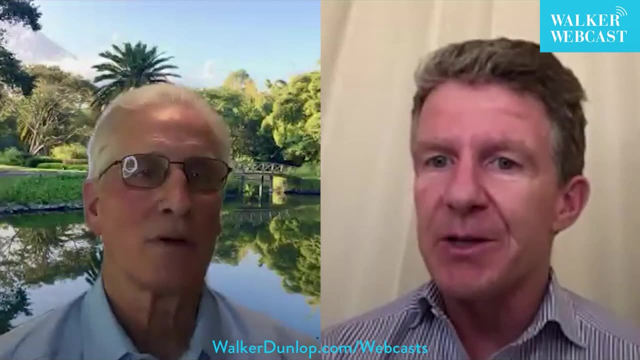 We had 1.4 million people a week file for unemployment And this past week- or I guess it was the last week that you covered in this- we had 210,000 people file for unemployment and we're still well below the trend of 365,000. 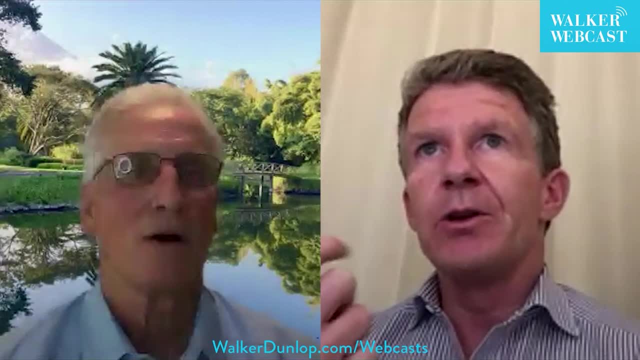 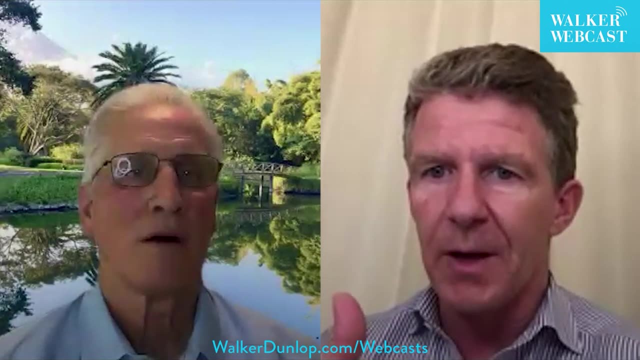 So that's one of the other things that just doesn't kind of put to me is your number is that you think there's 6.6% unemployment, but those people who have left the workforce aren't filing for unemployment. They're basically just saying: I'm not going to take a check from the government, nor am 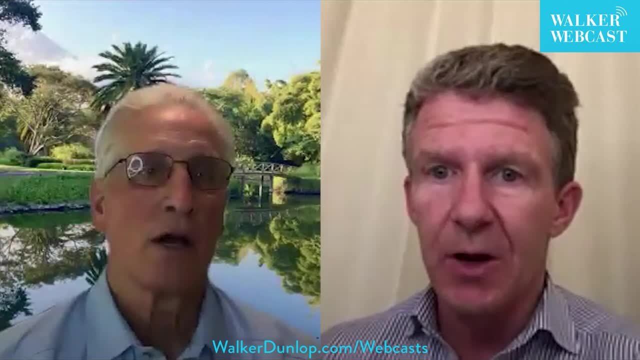 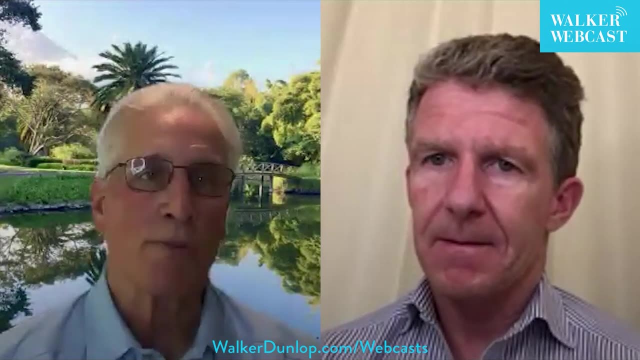 I going to go try and find a job. I'm just happy with what I've saved up and I'm done. They're basically saying I'm done and it's. you can find it in every age category, but it's basically concentrated in the 62 and over. 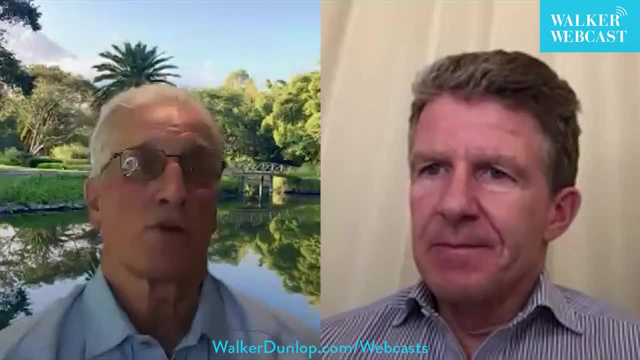 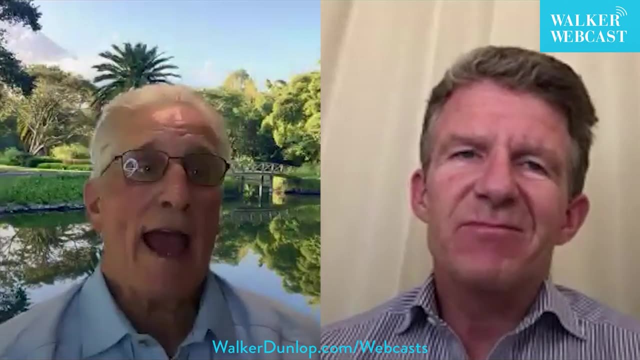 Some may have long COVID. some just said I was going to work four more years. I'm only working, you know I'm done. I'm done, Right. And eventually they were going to get extruded out of the economy, right? 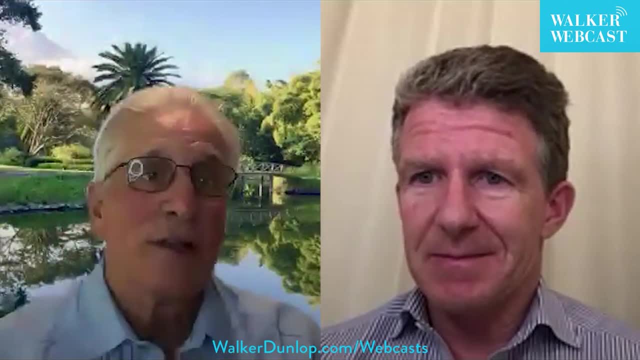 Just like that. Let's think of the toothpaste right. The 70 year old worker eventually was going to retire. They did it a few years early is what we've seen and they've not come back. They've just not come back. 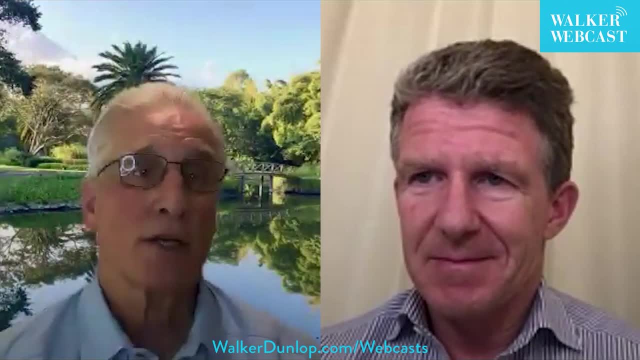 So let me go to that. These people who have retired clearly think that they have enough household net worth to be able to live the rest of their lives and have enough money to put food on the table, particularly if they're not filing for unemployment insurance. 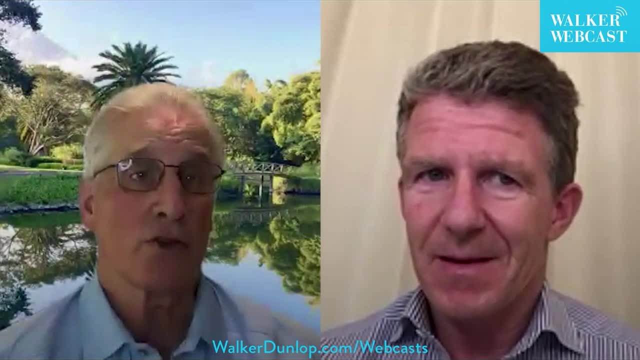 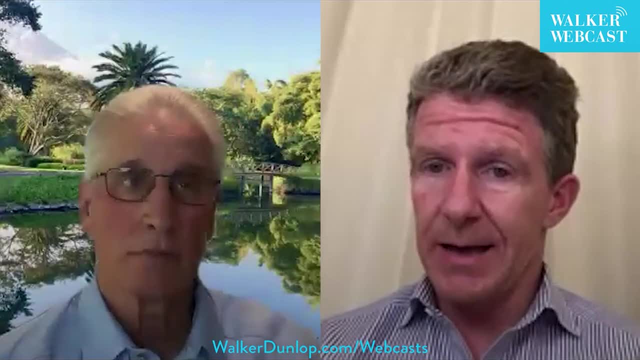 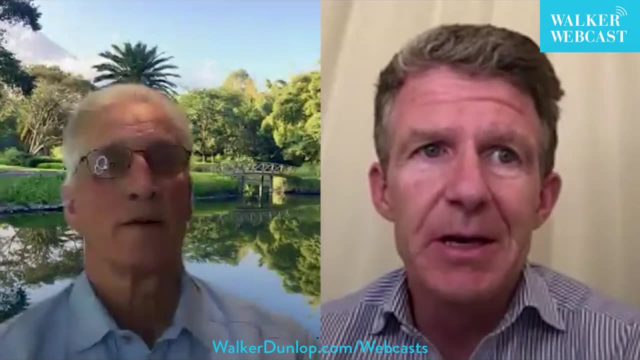 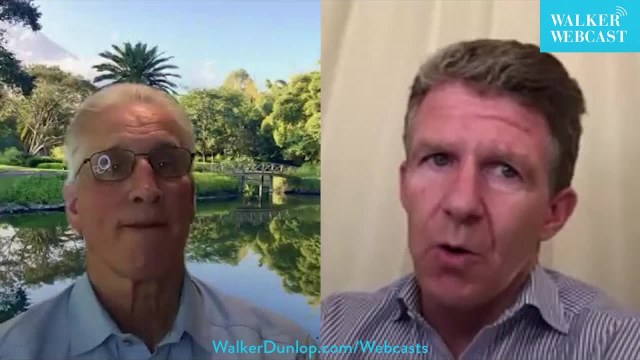 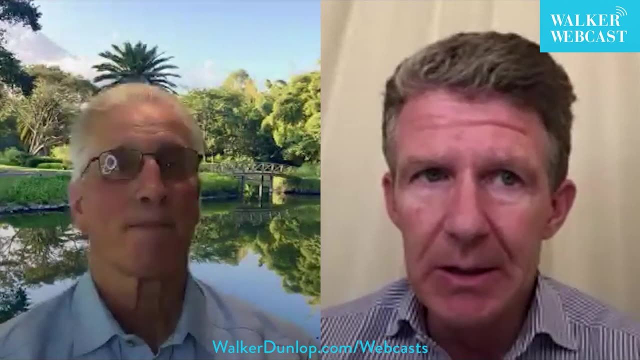 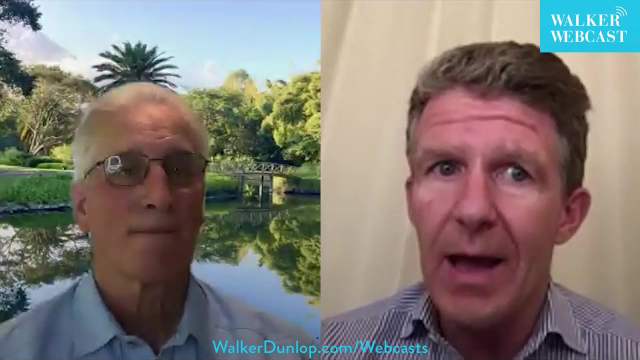 You have in the Letterman letter. real household net wealth stood at $154.5 trillion at the end of 2023. A big number And that is $461,000 per capita and way, way, way ahead of the long term average since 1955. 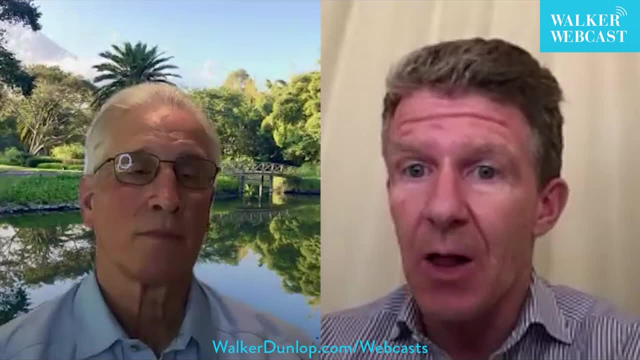 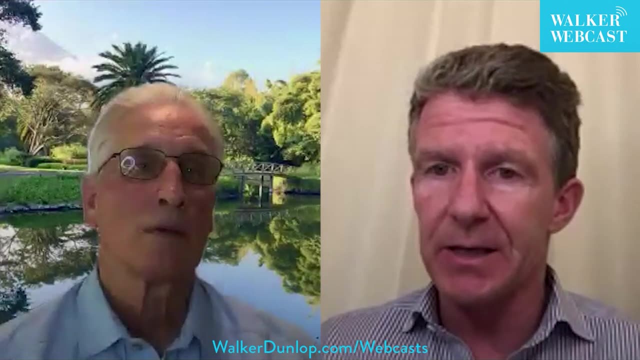 on a real basis of $223,000.. Right, on a per capita basis. And that all sounds good And it says, hey, the average person in America on a per capita basis is worth a heck of a lot more money than the trend has ever been, And it's. 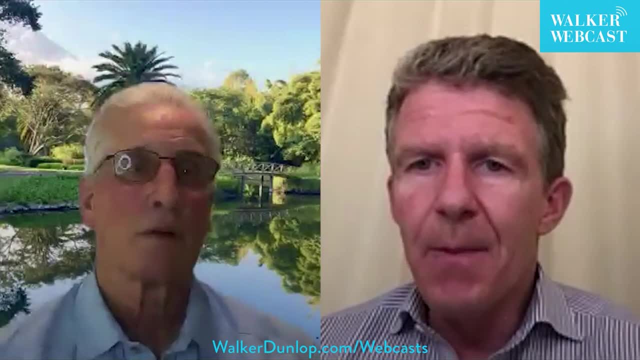 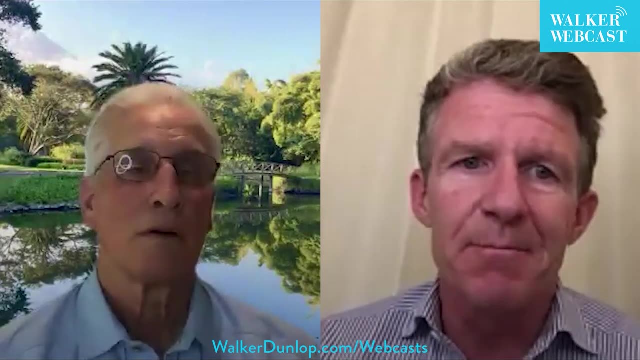 gone up precipitously in the past couple of years. You should say that's all great, But I want to ask you, Peter- I mentioned it a little bit at the beginning- I just went and looked at the 813 billionaires in the United States And that cohort of 813 people has a net worth of $5.7. 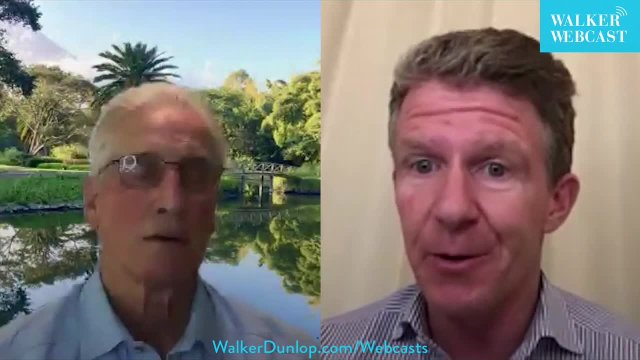 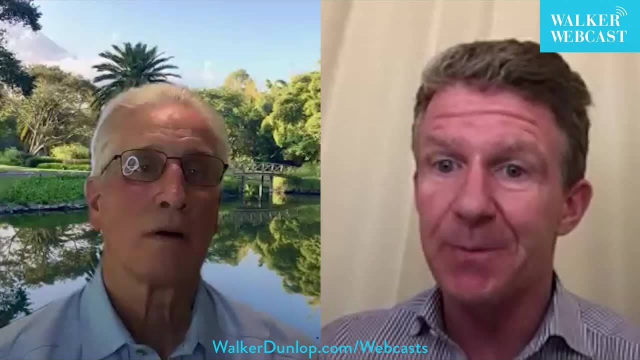 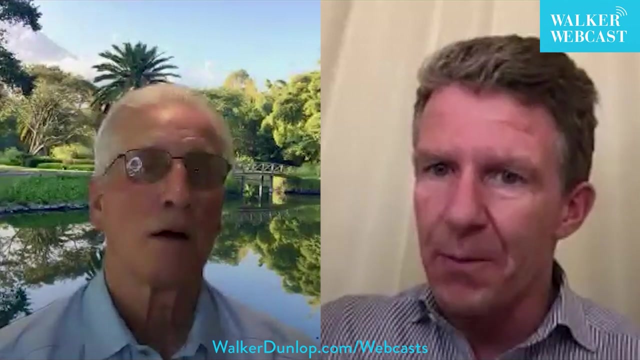 trillion, $5.7 trillion- in 813 people. So you just pull those 813 people out of the number and you bring down the average on a per capita basis by $14,000.. And so my question to you is: should we go and then peel back the top 1% that have an average net worth of $35 million or $33.5? 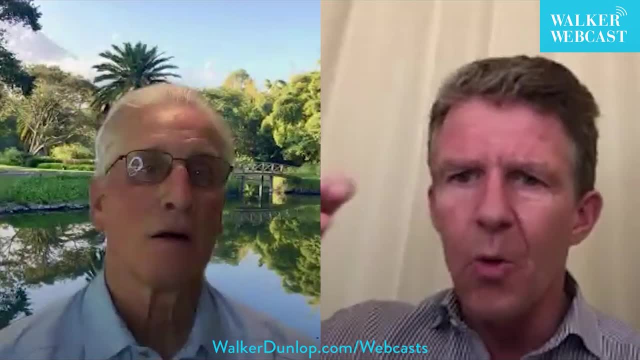 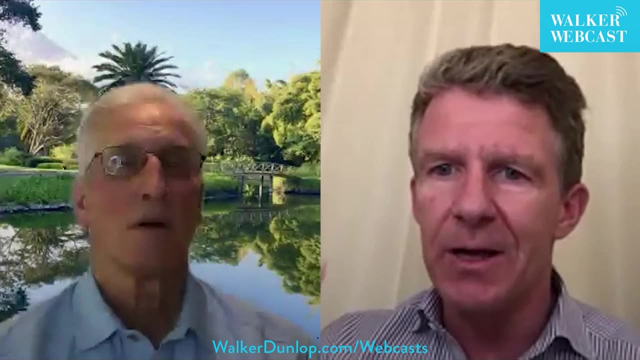 million And you pull that cohort out And all of a sudden, as you pull away some of those people at the top, that average number doesn't quite look so good. Are we fooling ourselves by looking at these big numbers on a per capita basis rather than really? 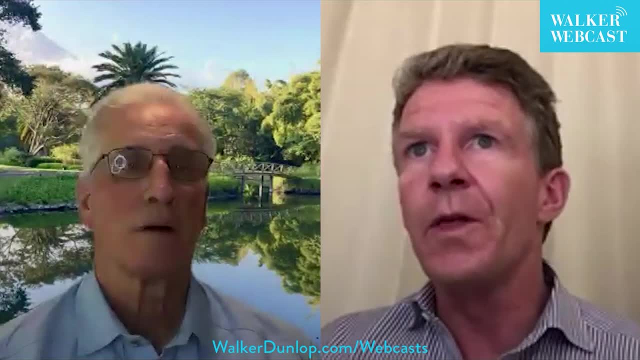 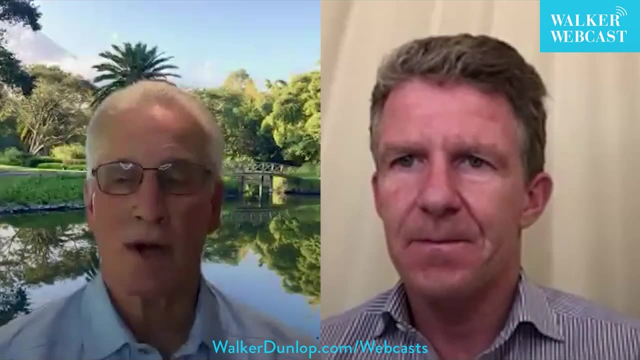 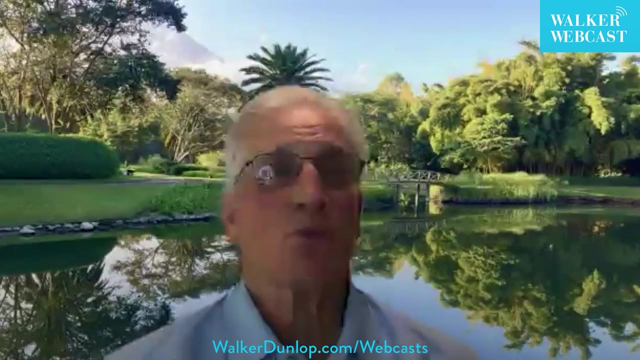 looking at income disparity and therefore getting fooled that the consumer is doing a little bit better today than they actually are. The Fed puts out a median number every so often. They don't put out the median number every time. That's why you're forced to use the average. 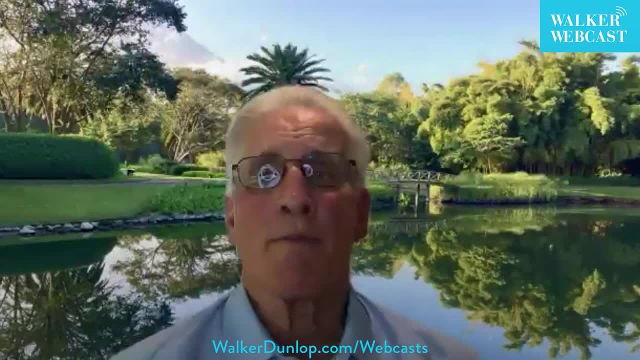 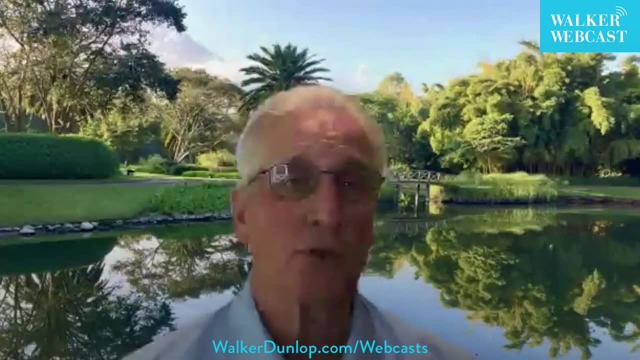 by the way, A median would be a more indicator. Remember that most people who are young have never had any wealth. They didn't have it when I was young and they don't have it today. You just haven't had any chance to build up wealth. That hasn't. 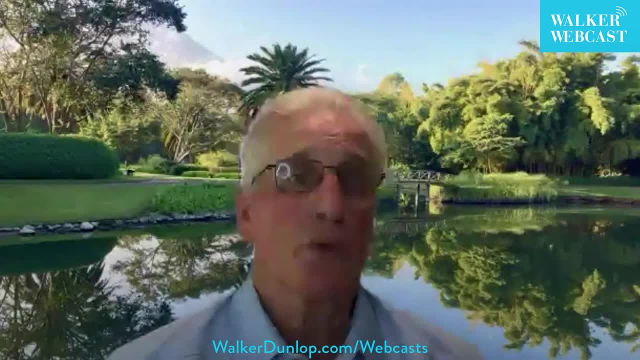 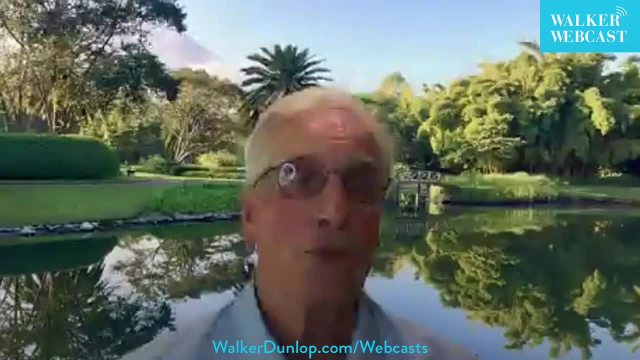 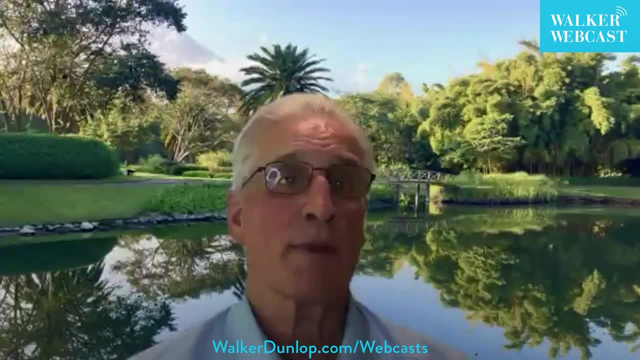 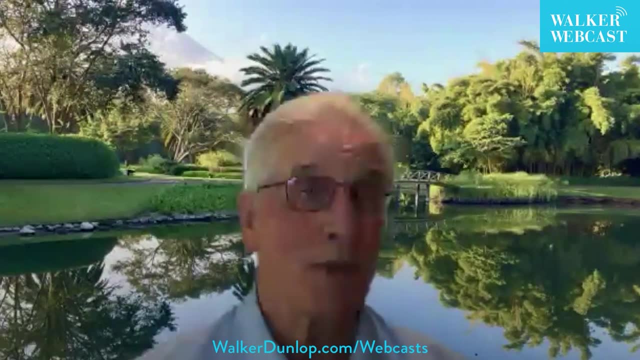 but it's an indicative metric. Namely, if that metric was down, it would mean a lot. The fact that it's up- and it's up notably- means something. Remember who's the primary owner of stocks In the United States? It's retirement funds. It's retirement funds, Most of those retirees. 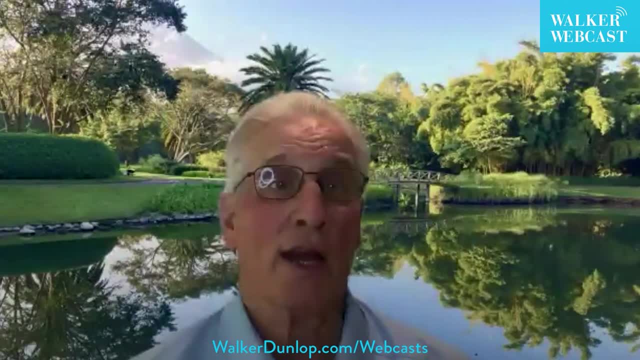 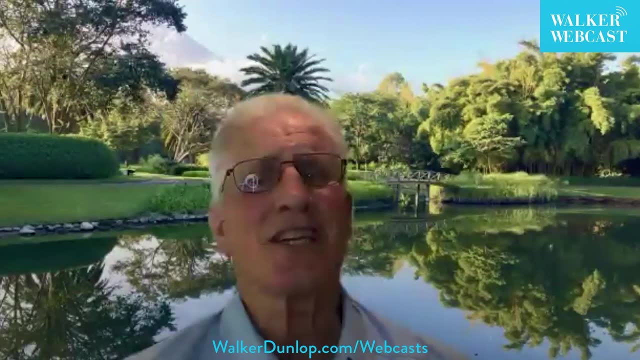 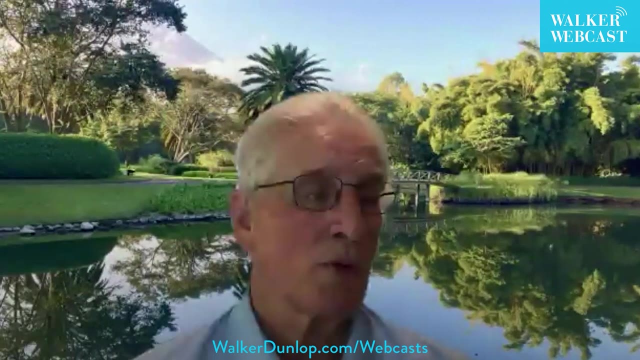 are not billionaires, Most of those retirees. they aren't even retired yet. It's in their retirement fund. They're not even retired. It's indicative. I don't hold it out as definitive, though I will hold it out in one way. We got a lot of questions pre-sent to us about the deficit. 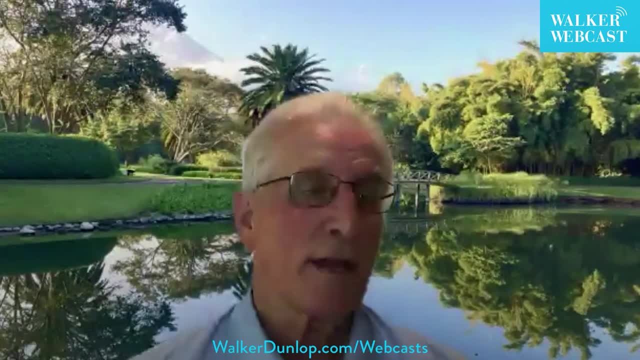 The deficit, The federal deficit. We've talked about that. if you take out the money the federal government owes itself, that's intra-company debt. One department would pay and another department would receive, so that's a wash. You net out the Fed, which is effectively a branch of the government with your federal government. same way. If paid off the debt that the Fed holds, the Fed would then just basically give it back to the Treasury. The Fed would then pay off the debt that the Fed owes itself, and it would be a half-billion. 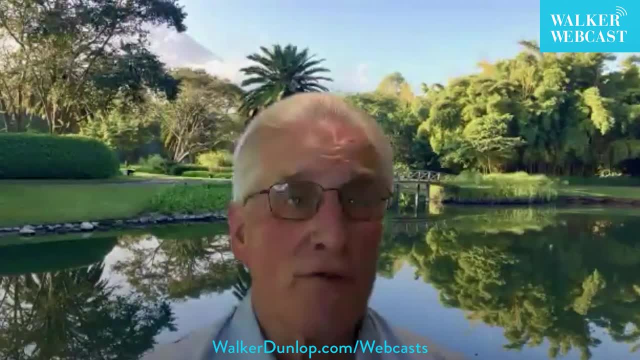 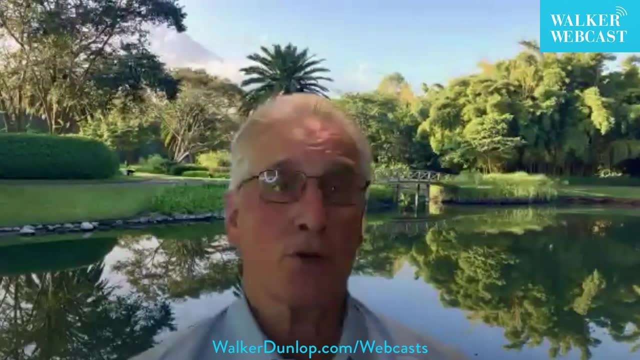 dollars of federal debt. Okay, What did we just say? that household wealth is 150 trillion. 150 trillion. We could take basically 10 percent of our total wealth and pay off 100 percent of our debt. What that doesn't even pick up is who would be the recipient of a lot of that money. that got paid off when we paid off our debt, off our debt Citizens. So citizens would take the $150,000.. Of that, about $7 trillion would go overseas, right Gone, And the remaining $11 trillion gets paid to US citizens. 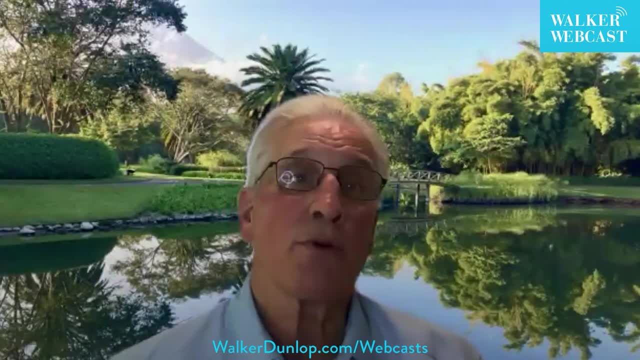 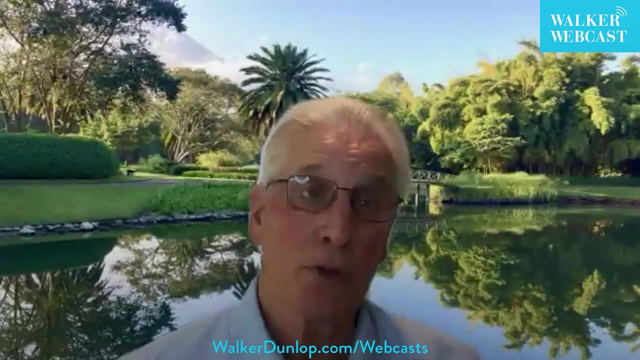 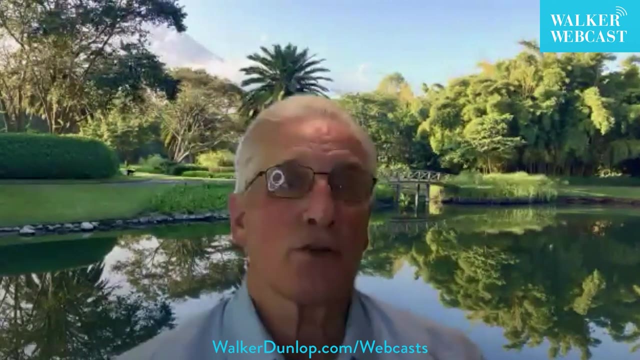 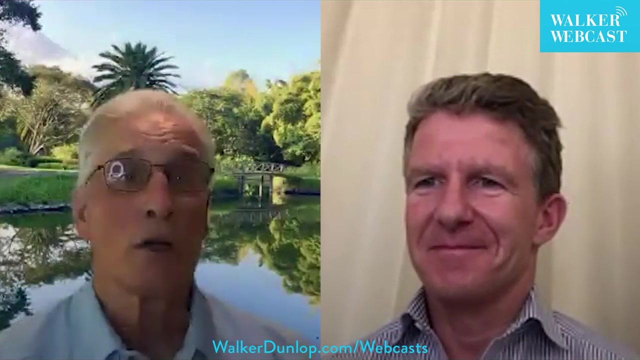 And so we go from $150 trillion wealth to $143 trillion wealth. right, If we paid. And so when people say the debt is big, of course it's a big number, Trillions are big numbers. I keep telling people: I don't care how big the deficit is, because it's small compared to our capacity. 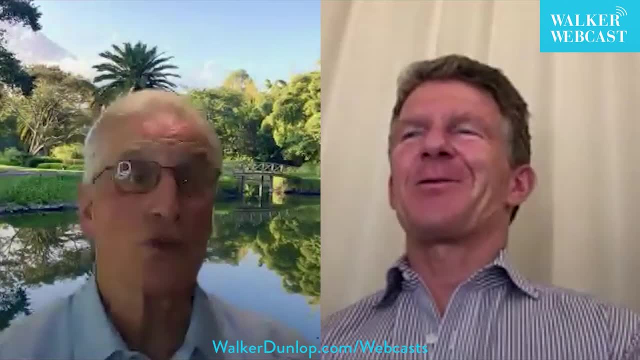 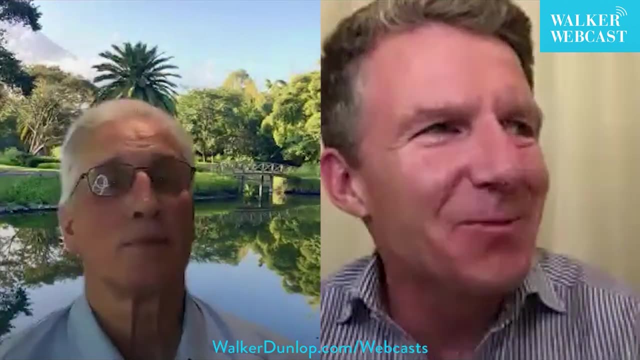 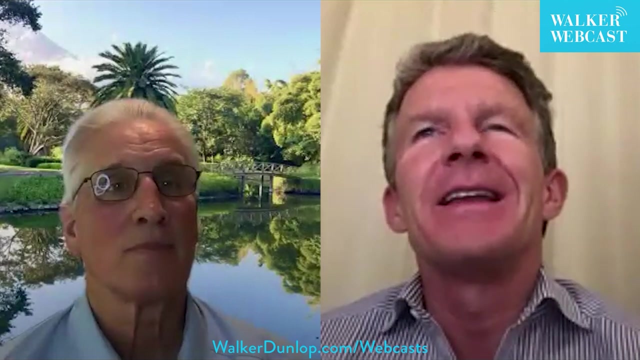 right, It's small compared to our capacity. I just did the work And that doesn't even count future earnings. I hear that. I hear that, And so when I saw that analysis again- and you're very straightforward in it and I understand the numbers, but I tried to think about it in another context- I sort of 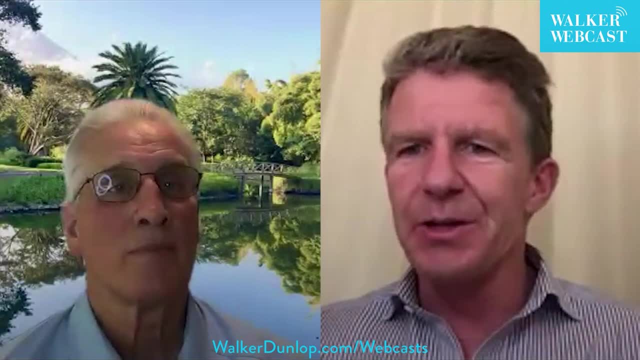 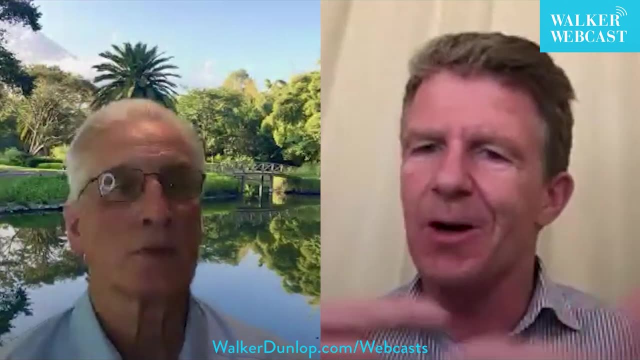 said: okay, the inner company is: let's just say we're using JP Morgan as the example And let's just say that the commercial bank has a loan out to the investment bank and they go back and forth. So all the inner company stuff you talked about in the US government, that all makes perfect. 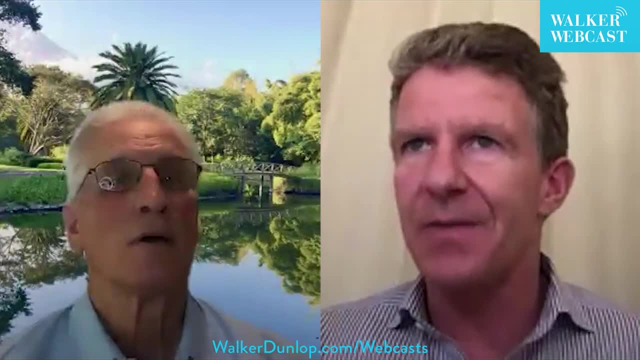 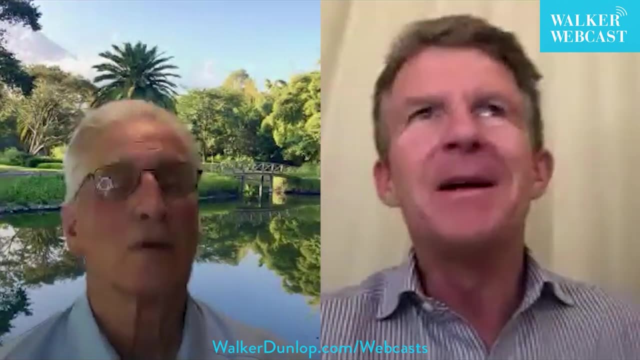 sense, right. So- That's all just kind of double counting. We're paying ourselves, Got that, But on your 17,, 18 trillion, which is with the US taxpayer and foreign entities, okay, I saw it there and said: 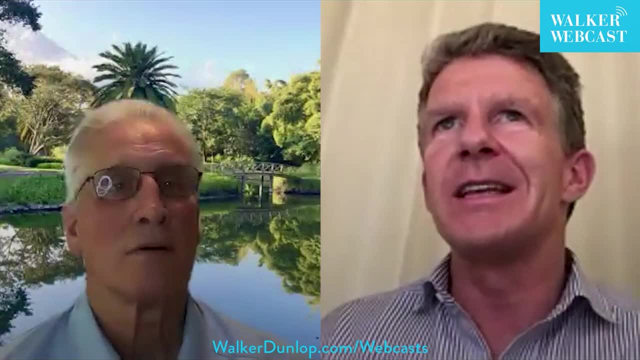 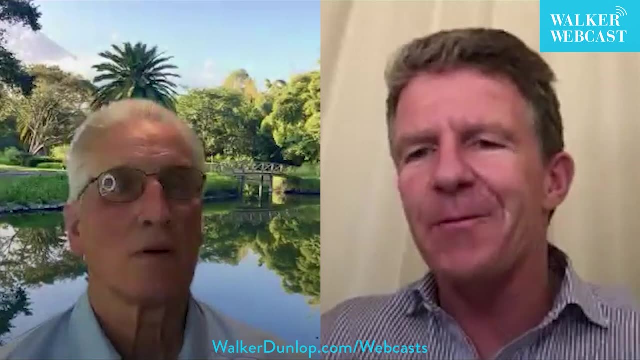 okay. well, Peter says basically that if you're a US citizen, the 11,, 12 trillion that's outstanding to US citizens, we can just sort of like forget, not forget about it, but we'd be paying ourselves, essentially. And then I thought: but if I own equity in JP Morgan? 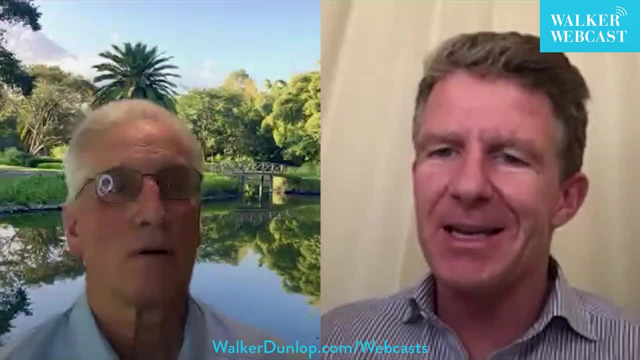 and I also own debt in JP Morgan and JP- and I also own debt in JP Morgan and I also own debt in JP Morgan and I also own debt in JP Morgan- decides to default on their debt. not only am I pissed off that they're not paying me off on my 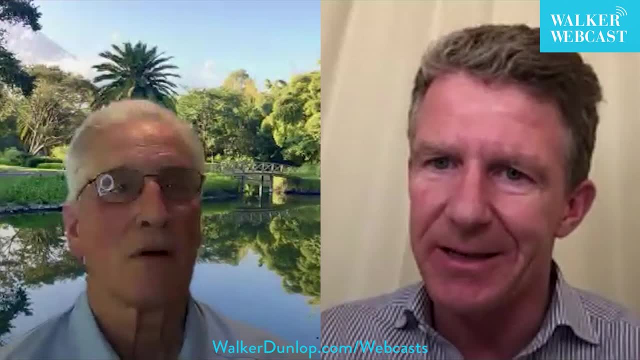 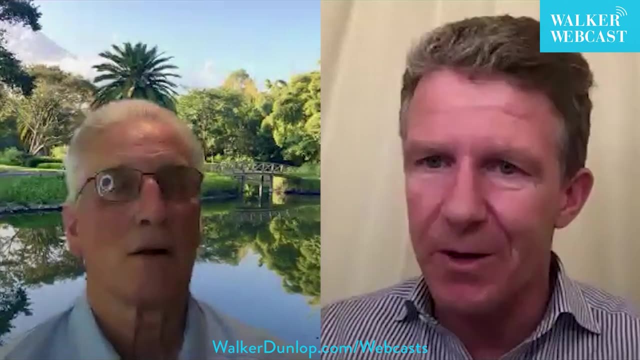 debt, but the value of my equity also goes down simultaneously. And so, and I say, here you run through those numbers. I sit there and say, yeah, that kind of makes sense, except for the fact that if, for whatever reason, we were to default on that debt, we will lose our place as the reserve. currency And the value of that 154 will come crashing down. to think of it in kind of a static way of- well, we'll just pay off the 17 and move forward, Doesn't, I think, take into account of people's fear that we actually default on the debt, that the cost of our debt goes up to a point. 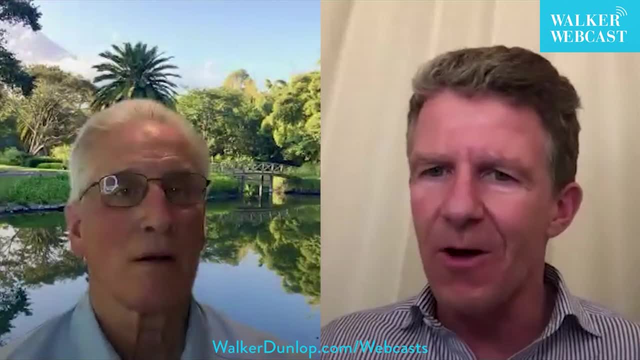 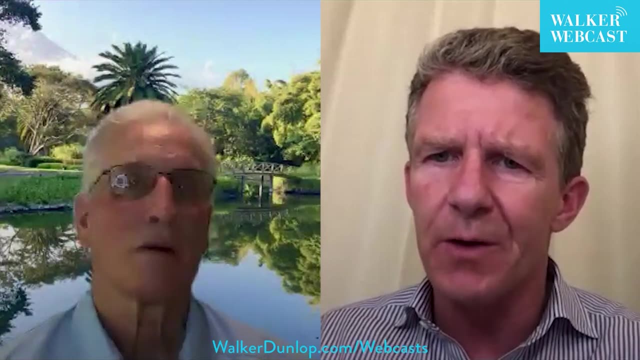 where we can't continue to pay it, And so I get the big numbers in the law of averages, but I don't get it in practice. If we find ourselves at a point where the debt has run up to a point where it's it's become a major thing for us to be able to service it. 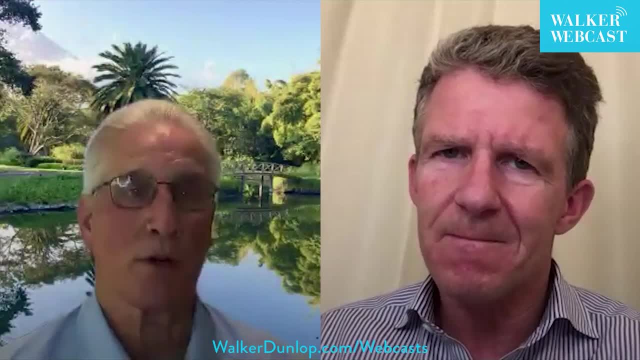 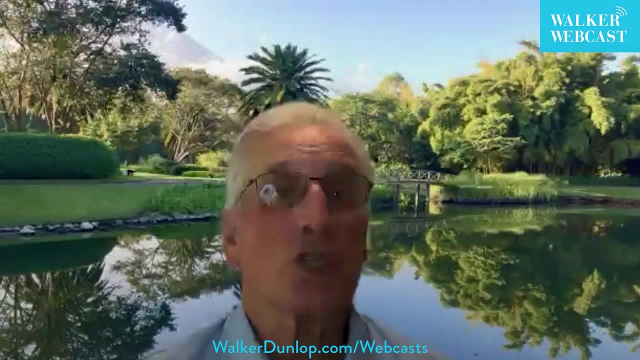 But it's not. it's not even close to that number. As I said, we could just decide to take 10% of our wealth and totally retire. Why would that? what's the problem, practically, with that? It's not an economic issue, right? Because, as I and remember, a lot of that is goes to us. It's not. 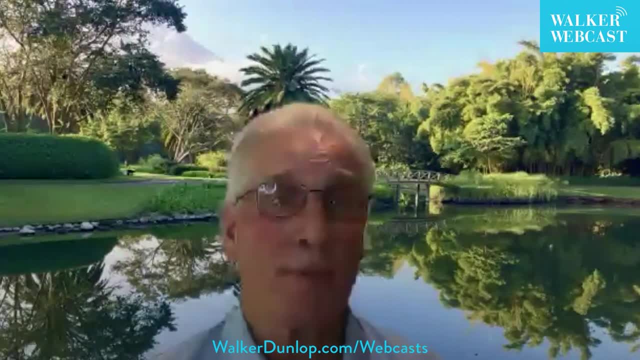 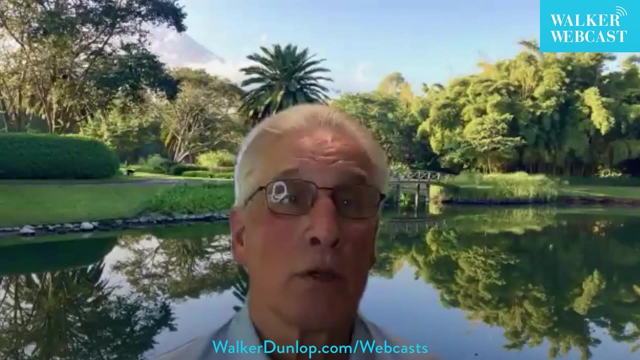 an economic issue. It's a political issue, Namely. okay, suppose we put forth a bill that says we're going to pay off the debt. That's going to be a massive political argument about how, exactly who- not us, who right? And, by the way, I'll start out by saying: 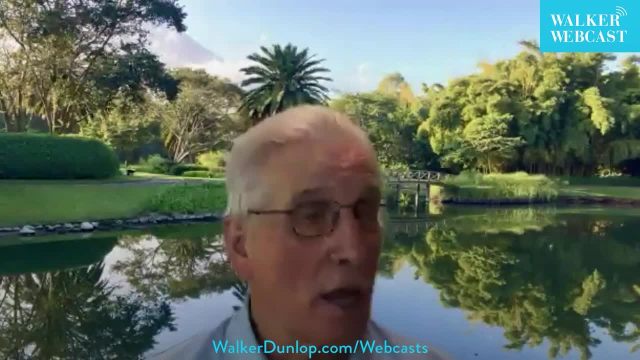 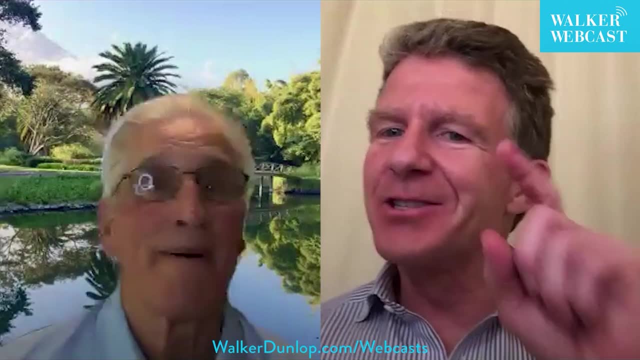 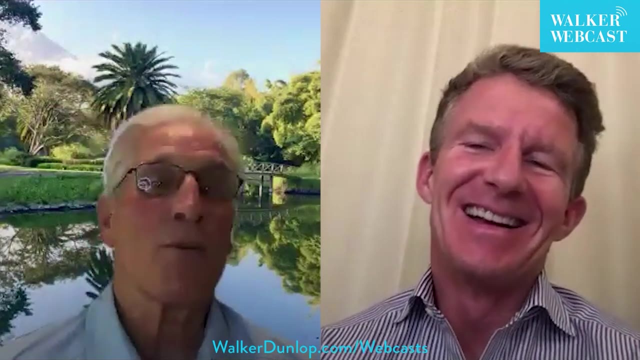 Namely, you should pay because you're young and vibrant and a CEO And I shouldn't pay. I just had a birthday. I just had a birthday last week. I'm catching you, Peter, I'm coming up. Watch out, I'm coming fast. I'm going to tell my Congress person that I'm old and I worked my whole. 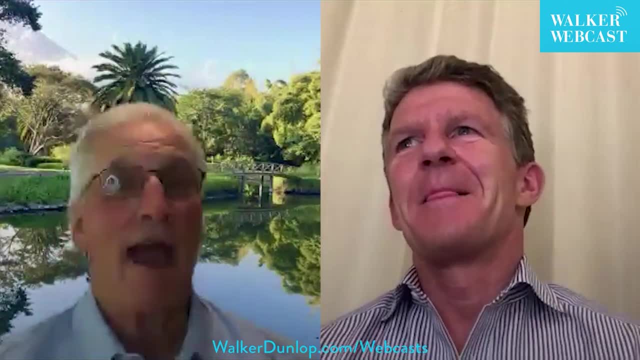 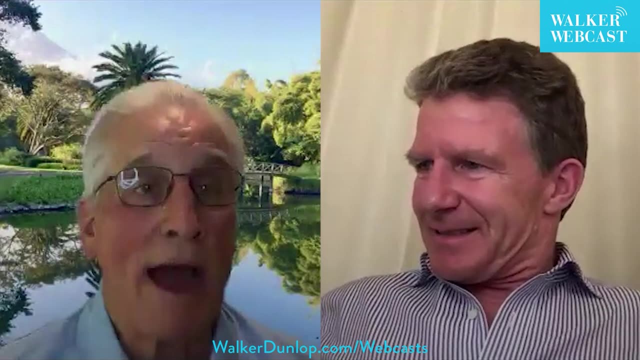 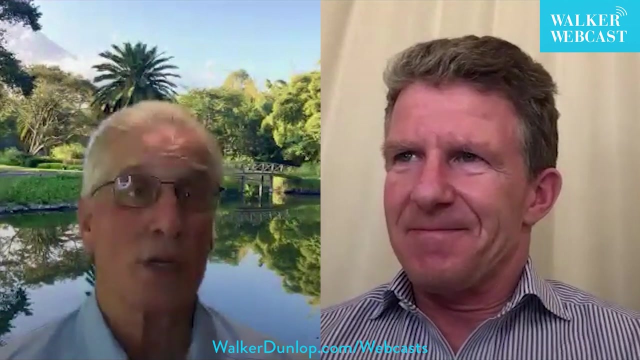 life and I can't afford to pay. And then the young person is going to say: don't take it out of me, And that's why it's a problem. So the debt has a problem because it's a political nightmare of how to deal with it, But it's not an economic. don't confuse an economic problem with a. 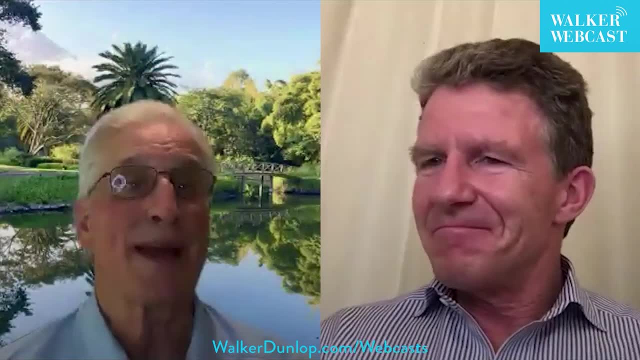 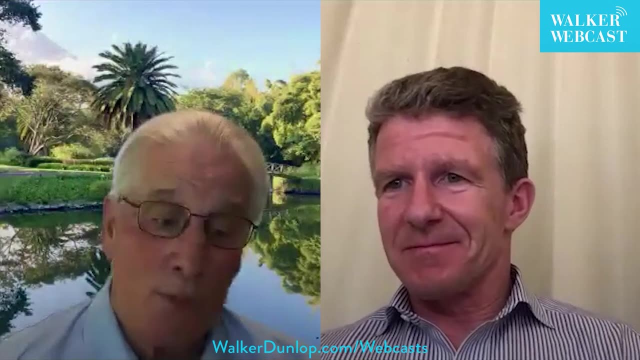 political problem. It is a massive political problem And it's a trivial economic problem because we have the resources. Now, the other thing I always want to point out on the debt is people say, oh, what about the deficit, What about the 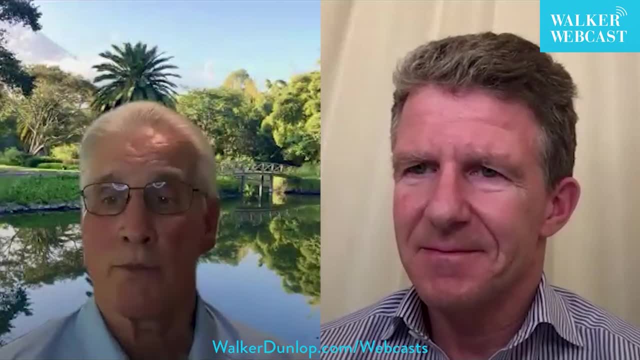 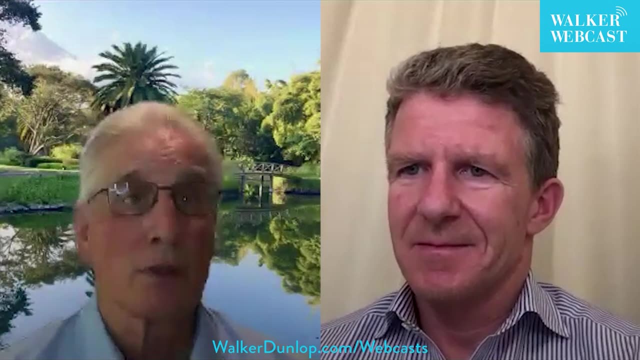 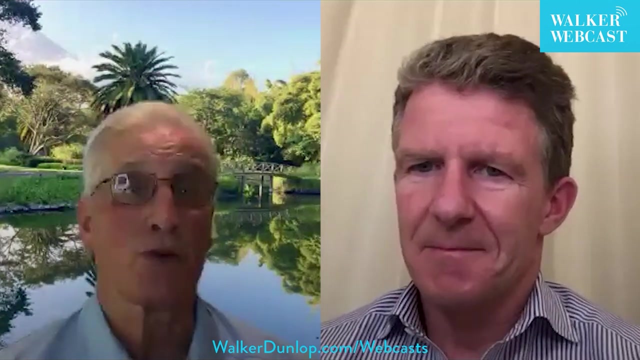 the budget deficit this year, the spending deficit. If it was tremendously productive spending, that the government's doing great. But if it's wasteful spending, it's wasteful, no matter what the number is. So if it's a tremendously productive spending, that's causing the deficit. bring it on. The economy will be better for it. But if it's wasteful spending, even if it's a tremendous productive spending, it's a wasteful spending. Even if we don't have a deficit, it's wasteful spending. 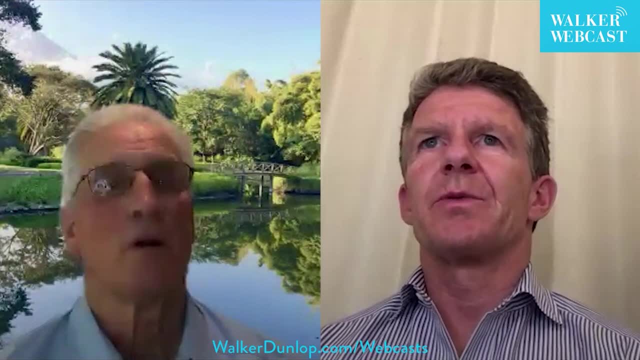 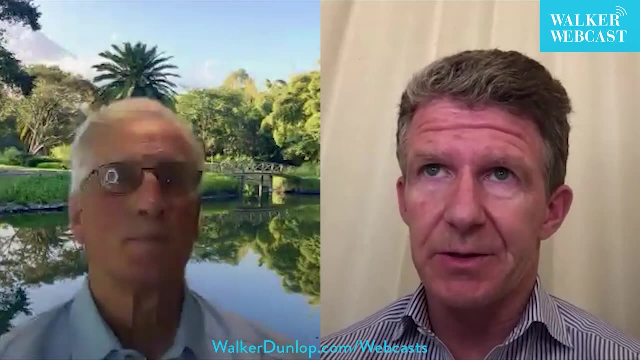 So let's jump to the consumer for a moment, because there's been a lot of concern as it relates to the overall health of the consumer, debt balances and credit card delinquencies, et cetera, et cetera. So just a couple data points to frame this. The first thing is that total household debt is about 18 trillion, which is just about exactly on top of total household cash holdings, So there's as much as cash In the homes as there is in debt, And one of the metrics that you put forth that, I think, is very. 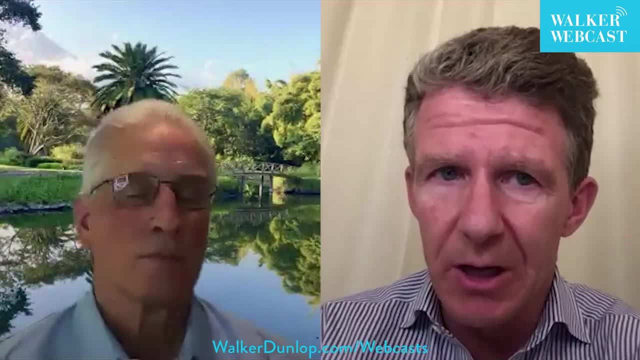 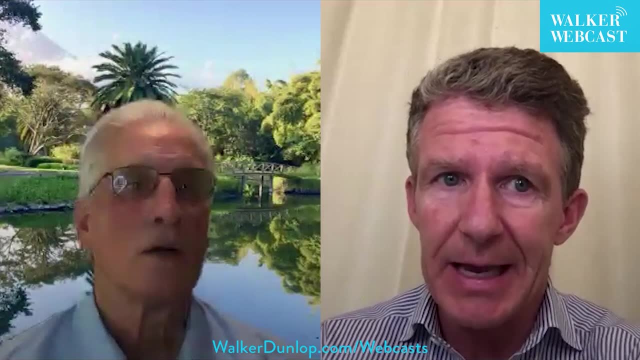 important is total household debt as a percentage of disposable personal income stood at 81% in Q4 of 23.. So at the end of last year it was at 81%, which is down from 88% in Q4 of 2019.. 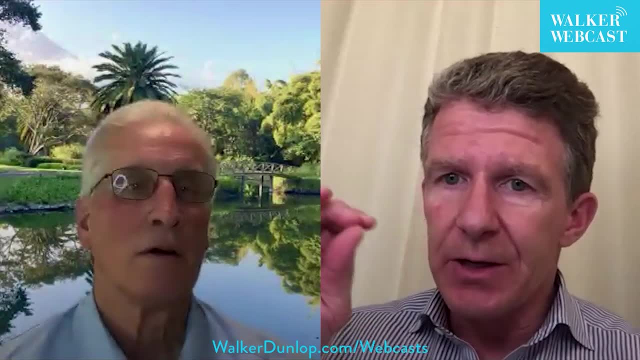 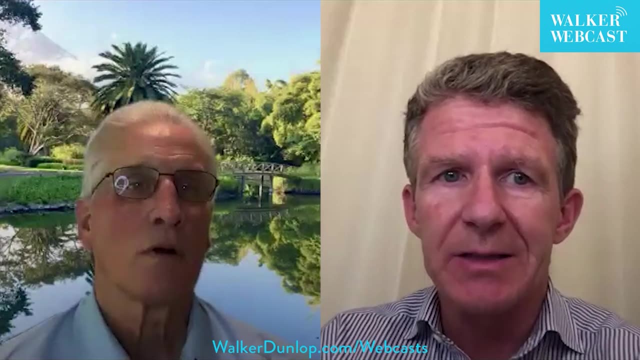 So back to this comparison of 24 to 19,. the consumer, as it relates to outstanding debt and disposable income, is in a much, much better position today. They were back in 2019 to other on credit card data points. And then I want to. I want to hear. your thoughts on the health of the U S consumer from a debt standpoint. credit card delinquencies: 2.6% at the end of 2019 and just under 3% at the end of Q3 this past year. That's the most. 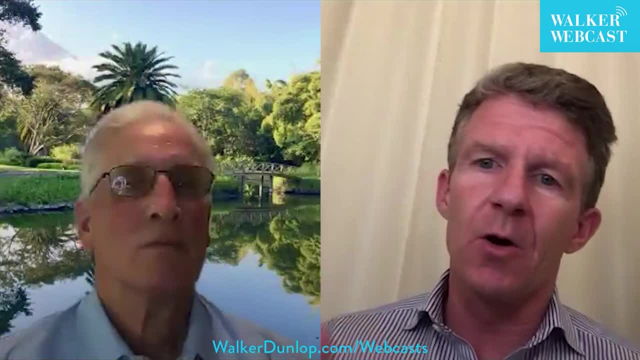 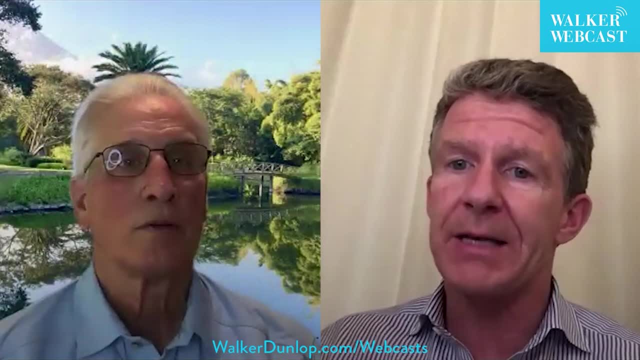 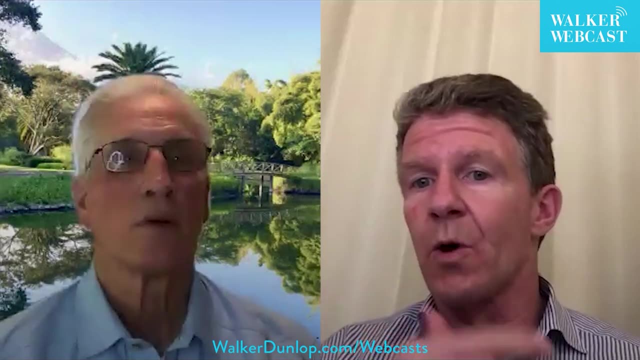 They're not. people aren't leaving outstanding balances on them, So you have a massive amount of increased outstandings, but that does not necessarily play into delinquencies. And the second thing is that if you look at where we were post pandemic, 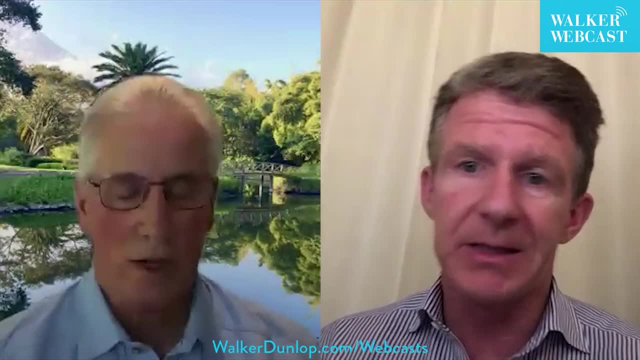 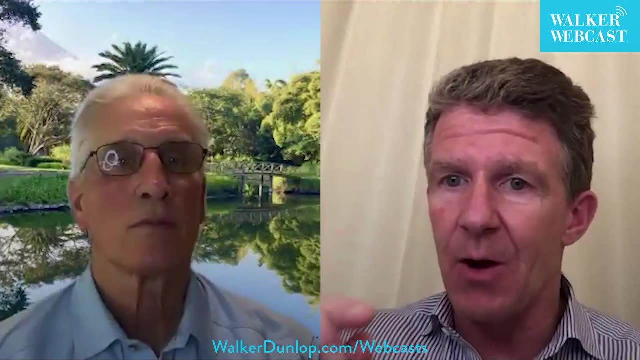 the delinquency number crashed down to basically nothing because everyone's getting the government. Now we're back to what is normalized delinquencies. Do you see anything? is it's now gone from 2.6 to 2.8 to three? It's just under three. Do you see that trajectory? 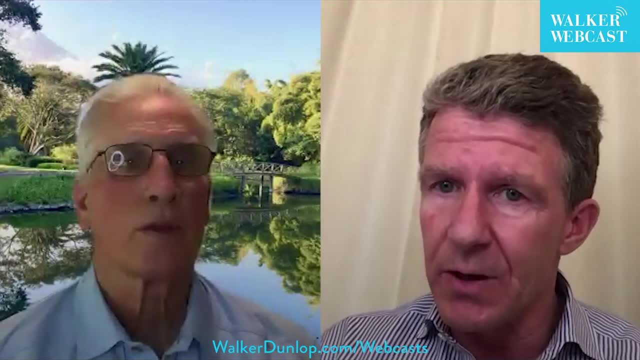 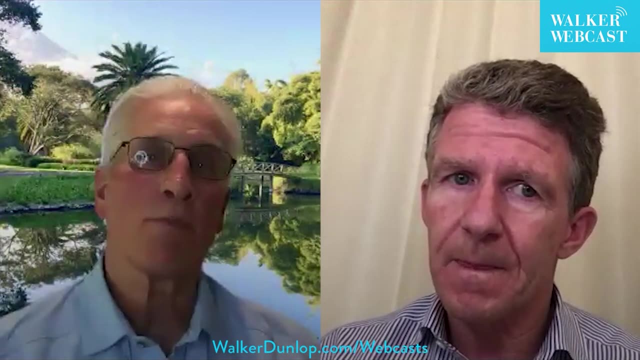 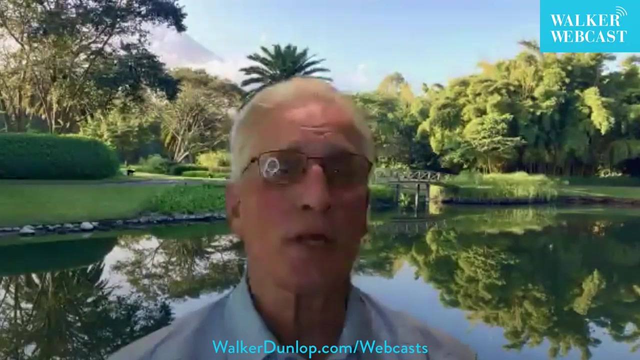 continuing where we might have some real weakness in the consumer as it relates to credit card defaults- Not deep weakness a little. There are certainly some people who got a little over exuberant right given the handouts and such, and probably did overextend themselves a little. 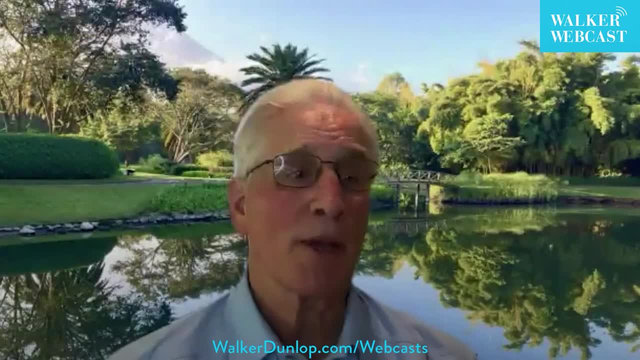 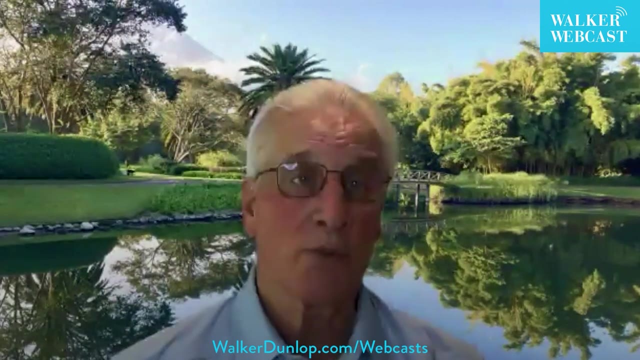 more than normal, But in the big picture, as you know from looking at the chart, the debt levels, the delinquency levels are nothing frightening. People still have jobs, they're still getting wage increases and there's still a lot of jobs available for people. And those are the keys. 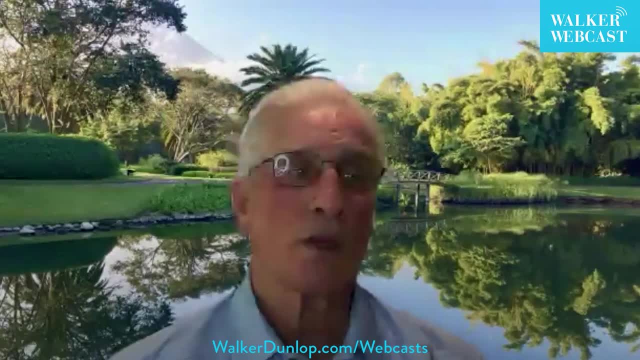 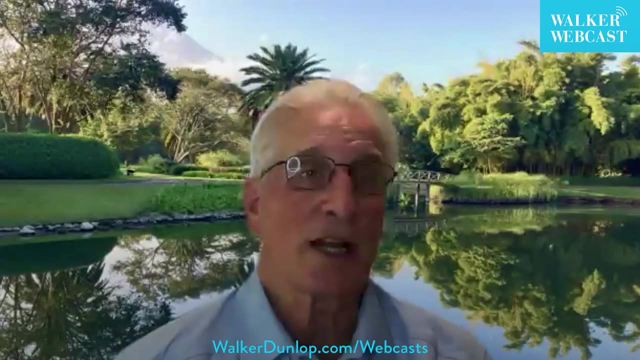 really in that regard And the debt number is really kind of understated because credit card usage falls For convenience. today versus 2019 is much higher. It's hard to know how much higher. That's very carefully guarded by the credit card companies. They don't want to let people know how much is. 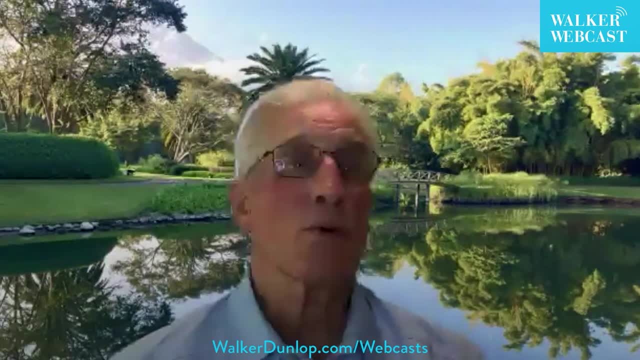 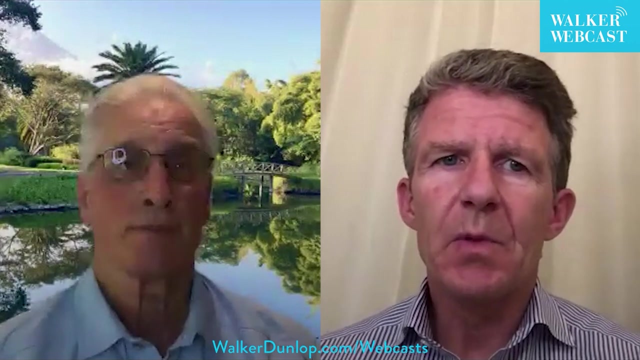 never paid interest on right. Remember that credit card companies do absolutely make money by charging interest to people who don't pay it off, But their main source of income is through the fee, The fee, The fee. They charge the vendor Right. Another thing that a lot of people and you go into it in quite some detail in the letter. 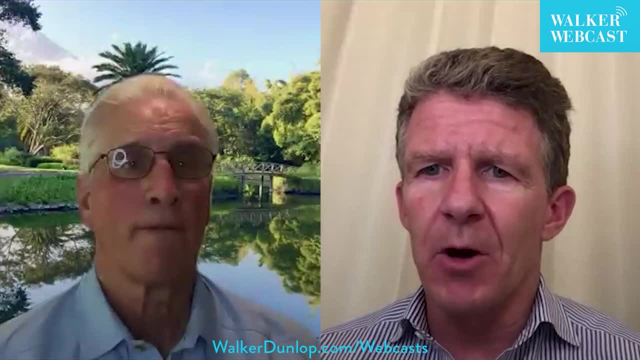 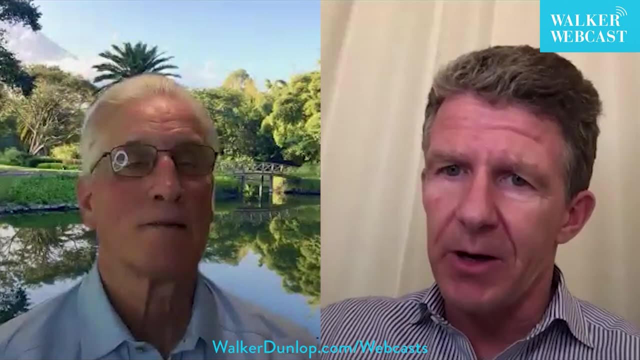 Peter, is the amount of money that's in money market funds. I think there's been this sort of people. as rates have gone up, everyone said, oh, there's all this. you know, there's trillions of dollars sitting in market and market funds And the moment that rates come down, all that money. is going to come flowing out of money market funds and back into the equity markets And it's going to be this big surge of capital because it's seeking yield today sitting in money market funds And it will all flow back into equities when rates come down. Tell people why that's not necessarily. 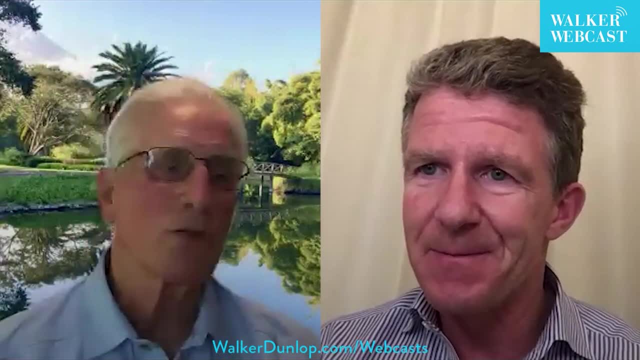 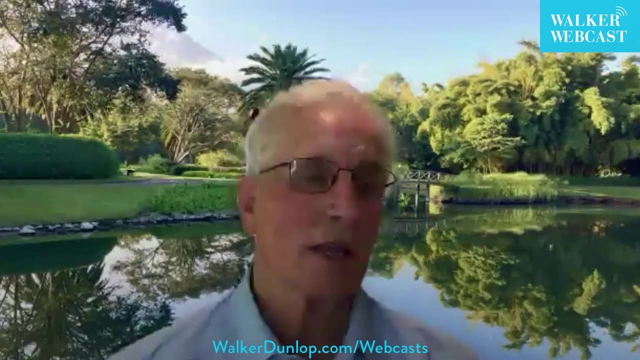 the case. if you look at the data over the last 15 years, Yeah, I don't think it will all flow back in. We never saw this much cash come in at once. The interesting thing to me is during the- I'm going to oversimplify, which I'm prone to do- 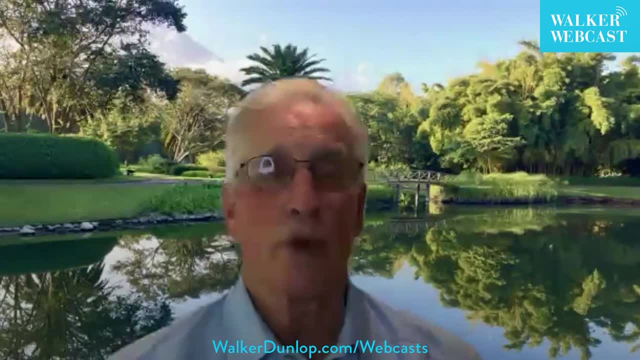 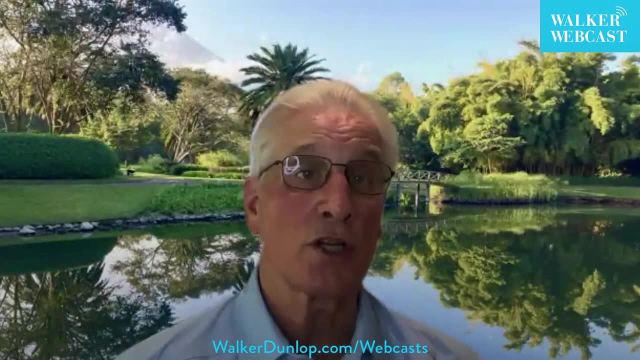 Um the we. we borrowed a lot of money. uh, during the pandemic right, We borrowed a lot of money and we gave a lot of it to citizens and businesses. about four out of every $5 we borrowed and gave to citizens, they saved, and they saved in the form of cash. That's one of the reasons we didn't have 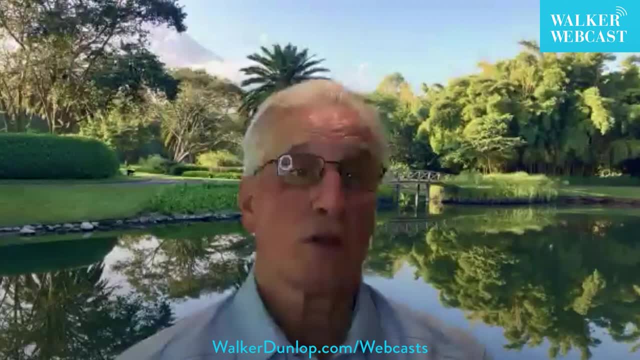 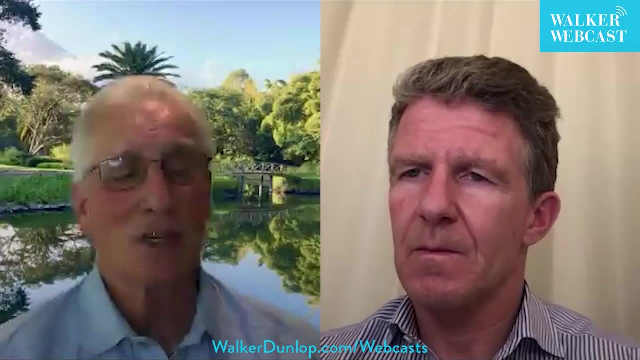 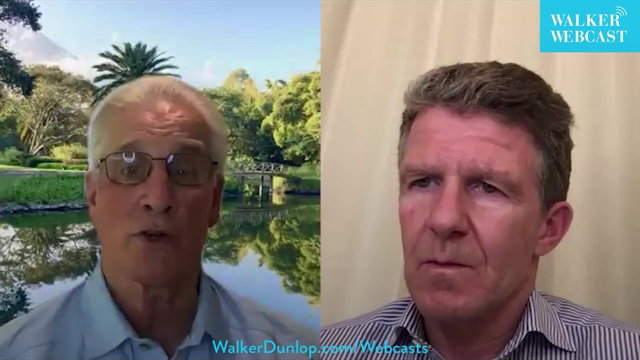 runaway inflation right away is they kind of kept the money. So as a result, there's a decent cash cushion that people have not normally had. Now it's slowly adjusting. It's slowly adjusting over time. I don't think they'll all go into the stock market. 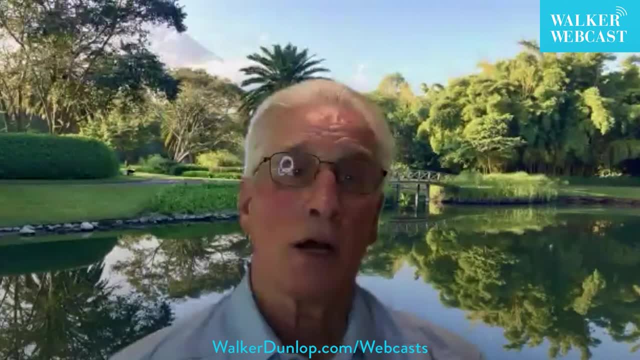 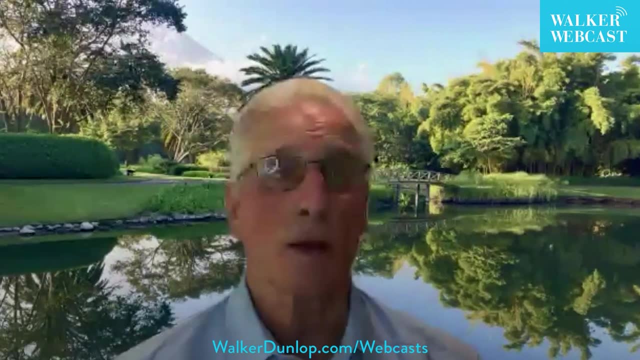 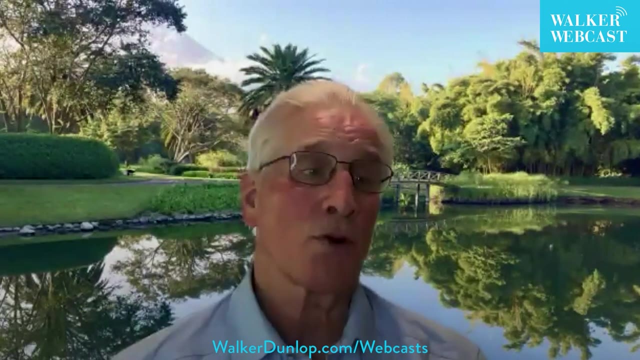 but it will find a home. Right now, it's pretty simple for people to say: well, I'm collecting 5% or something on my cash account, You know, I don't have to think a lot, You know, and so they're leaving it in cash. 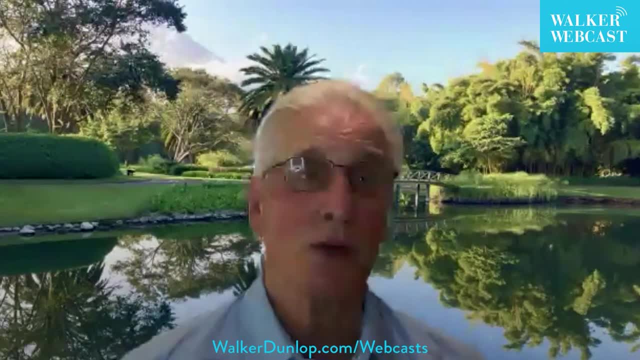 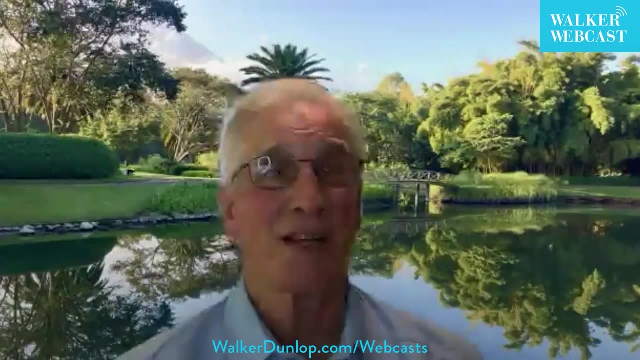 They kept it in cash originally when they got it because they were terrified And they didn't know what was coming next, And now they're getting a decent return on it. So I got a day job. I'm not going to worry about that right. 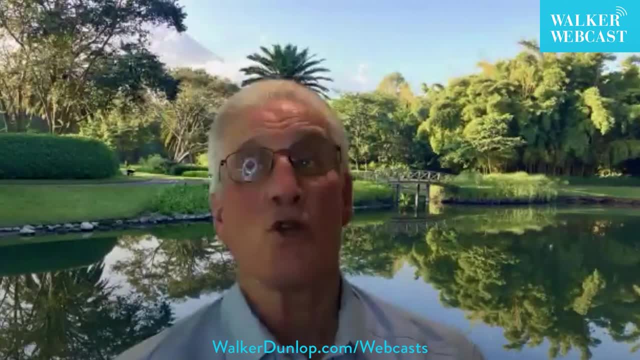 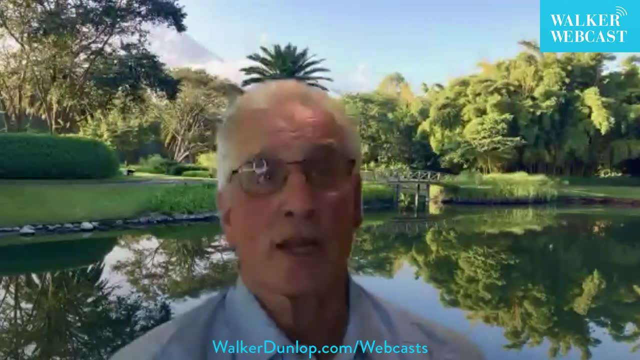 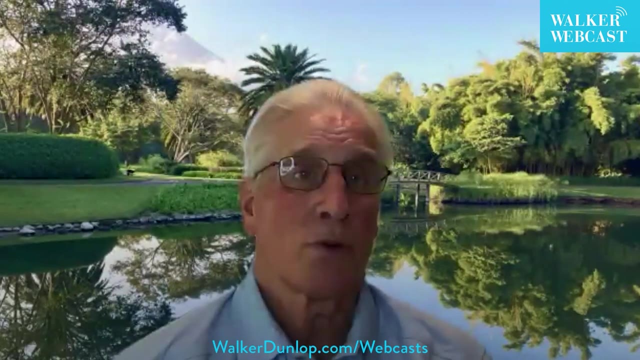 And as things normalize, as the interest rate eventually comes down, as the Fed comes to their senses, some of it will flow and some of it will stay in cash. By the way, some of that money is going into vacations and some of it's going into 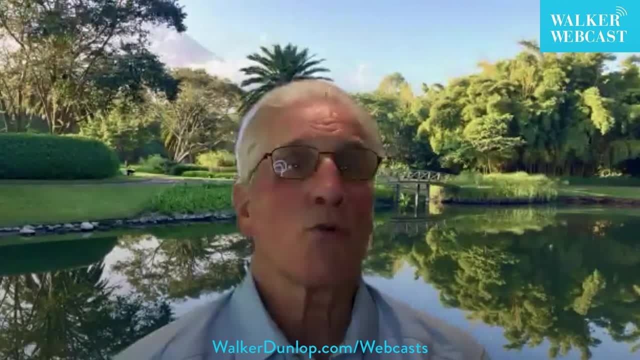 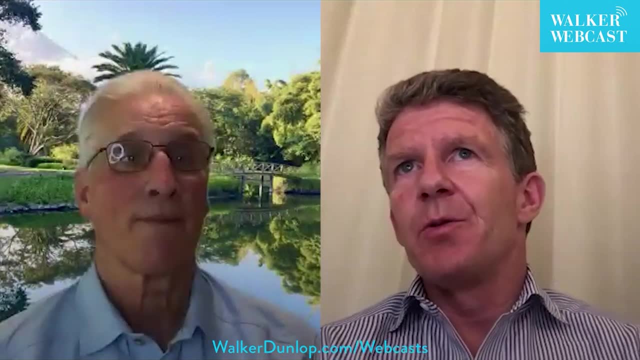 So it is trickling out, But trickle is more the word. A lot of money out there, still A lot of money. I thought what was interesting was, as you point out, during the GFC money market, funds exploded to $4 trillion. And then we went to the zero rate policy from 10 until whenever you want to put your end on it- 10 until 19 almost- And during that period of time you only went from $4 trillion down to $3 trillion. Right, And so, while people Right Taking no money on those money market funds they still held at $3 trillion, You now have $6 trillion in money market funds, The concept that that falls from $6 trillion down to $3 trillion again. I think is probably unlikely. You're probably sitting at $6 trillion to $4 trillion or $6 trillion to $5 trillion. So I mean, while $1 trillion is at, it's not that $6 trillion all flows into the equity markets. and off we go to the races. No, Probably $1 trillion. $1.5 trillion of it will float and the rest just becomes part of my overall portfolio. Right, It just becomes part of the overall portfolio, So let's go to Office for a moment. 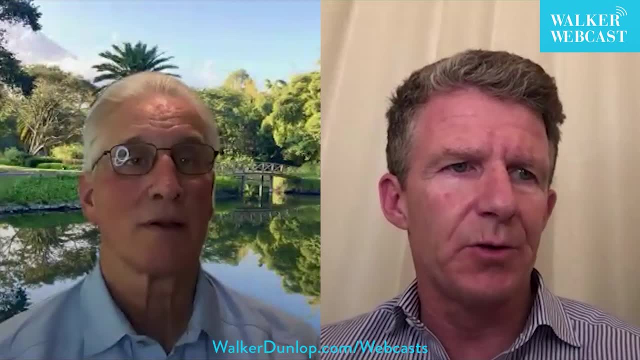 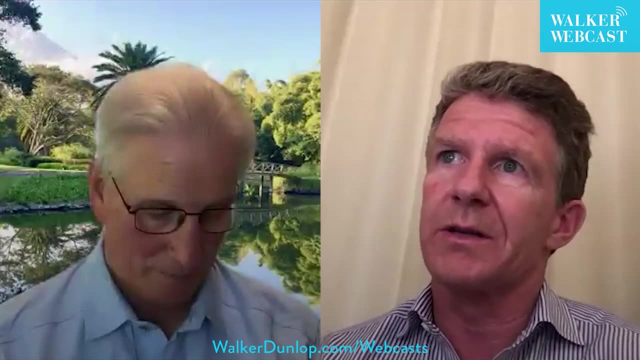 because a lot of people still have questions about it. I don't want to dwell on it too much, but clearly you've thought for a while. people are going to get back to the Office a little bit more quickly and more significantly, And they have. 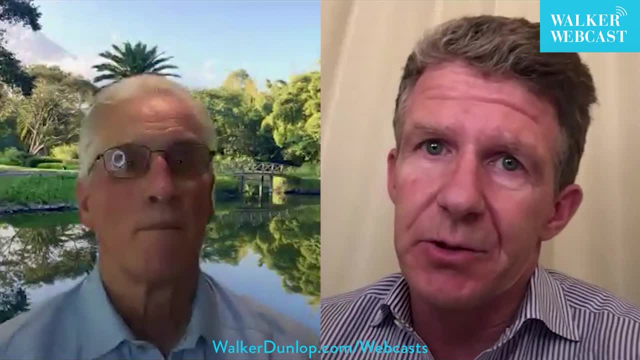 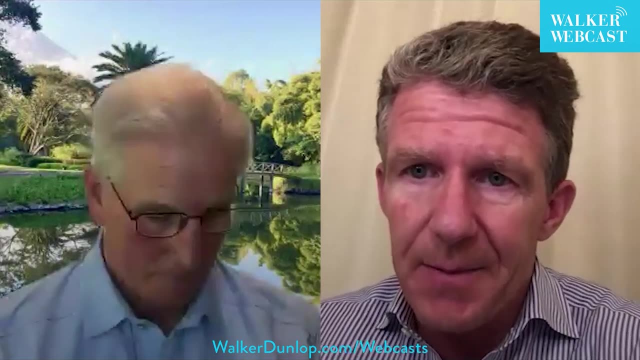 You have very good data that talks about the CASEL systems, tracking data of certain markets that have gotten back over 50% and then some of the Texas markets into 60%, But at the end of the day, people aren't returning to Office. 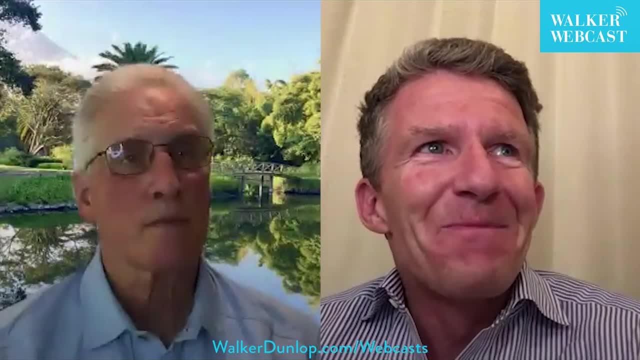 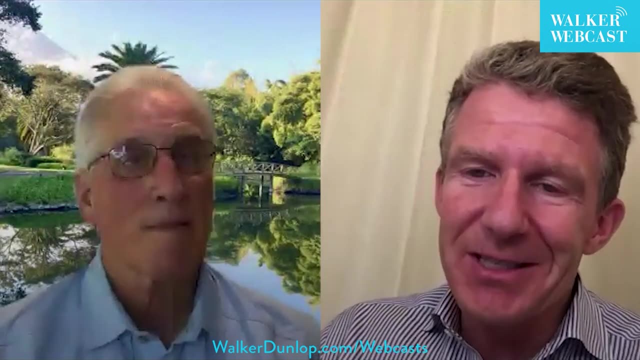 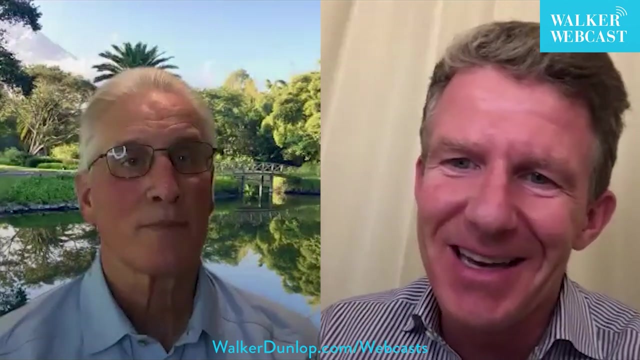 You also point out one of the best markets from a month-to-month basis on a decrease in vacancy rates is St Louis. It's your number one market. in this letter It relates to the month-to-month increase, And then on the front page of The Wall Street Journal today. 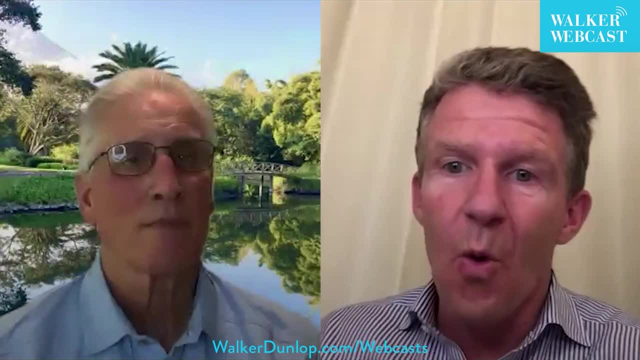 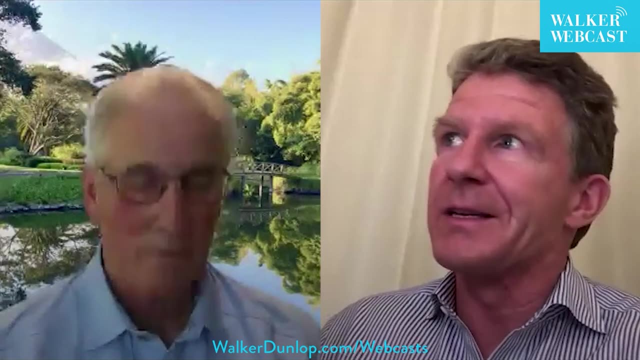 there's an article about the fact that downtown St Louis is basically a war zone right now, because all the office buildings are unoccupied, all the retail is shut down and people. not only is there crime, but the concept that they can revitalize downtown St Louis. 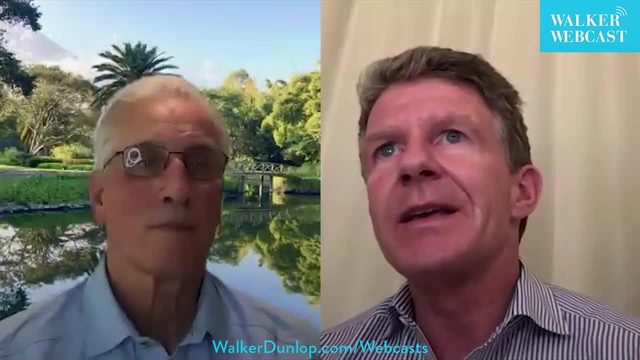 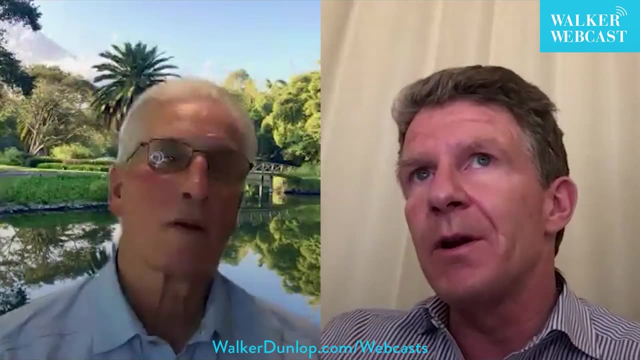 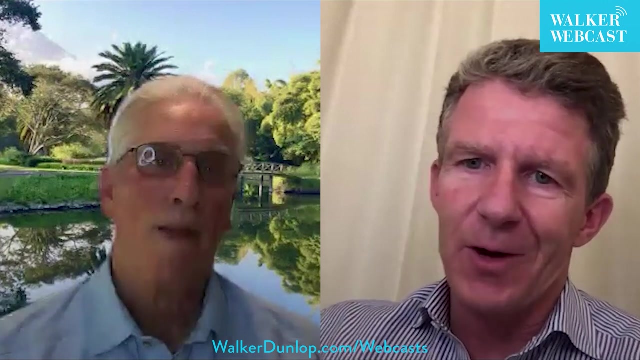 This article clearly puts some big question marks around it, So I guess the real question is how I mean. in your projection, given employment growth of adding 8 million jobs between now and 2028, you think that the office vacancy level comes down by close to 300 basis points. 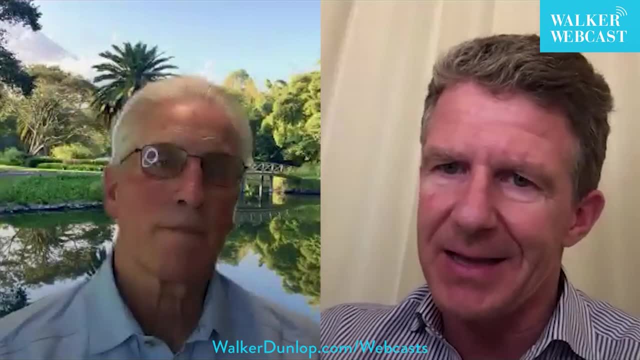 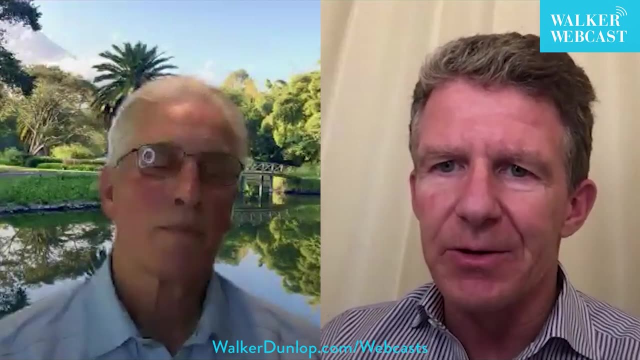 but that's from 14% to 11% or something like that, So it's not going to make anyone's day that you have projections in there. You also point out, Peter, that there's still $80 billion- $80 billion- of money going into new office in the United States right now. 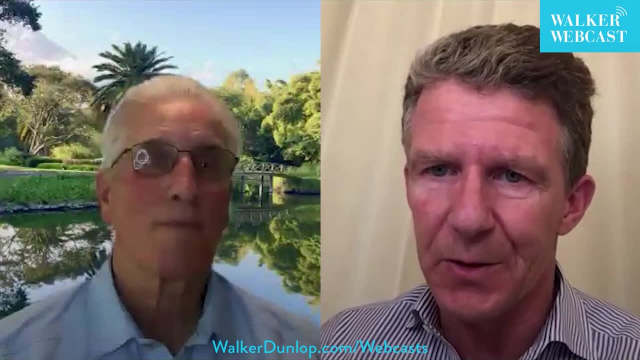 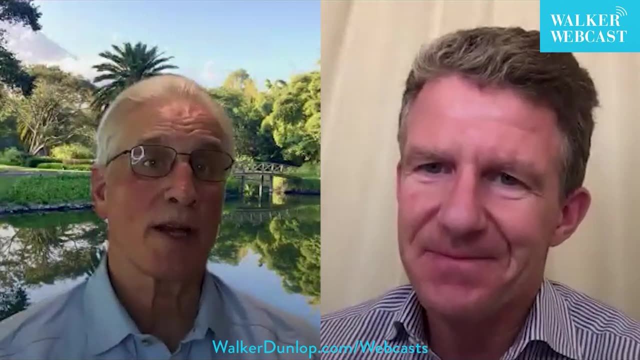 which just baffles anyone's thought about: why is anyone building a new office building today? So let me let you riff on office for a moment. So some of it is build out, to be fair right, Some of it is expensive build out. 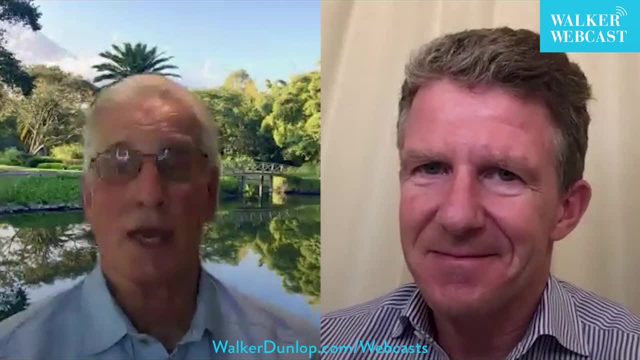 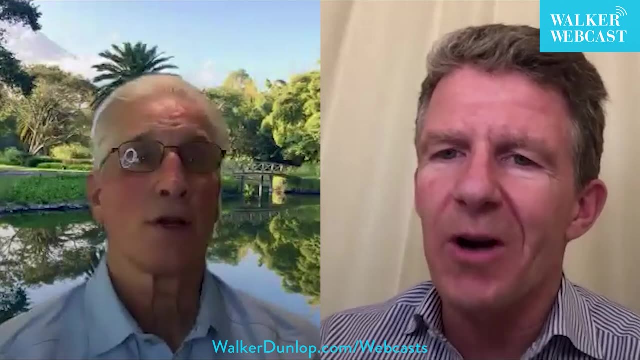 And, as you know, some of it is. if I build the shiniest, newest thing, that's the one that will get used, Because Walker and Donald is going to leave some space for you, which we're doing across the country and really nice. 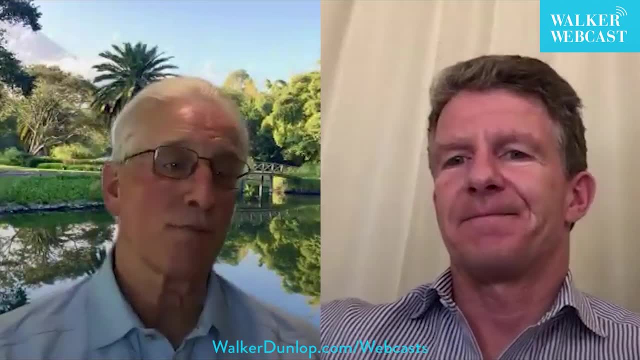 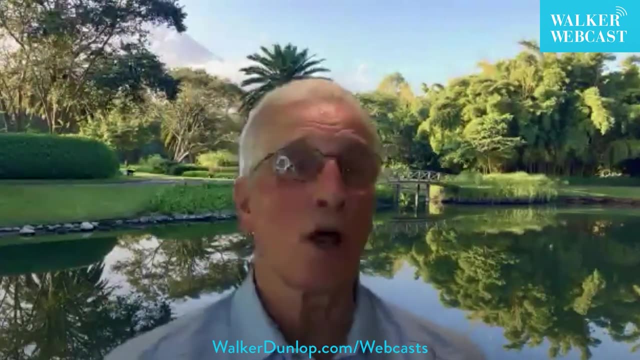 Right, You'll move out of your nice A minus B plus building to move into the shiny shiny. And if I can get you and a law firm as my tenants, I can get maybe a construction loan. blah, blah, blah, Right. So yeah, it is kind of stunning that it's being built. 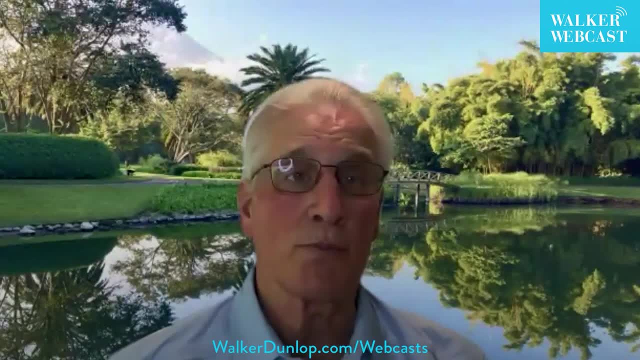 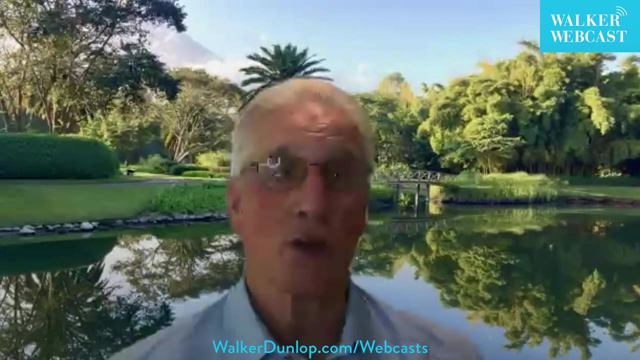 There's the. the number of properties being taken back by lenders is still quite low because they don't want them. Now there are some, there's no doubt there are some, But this is like the misbehaving 16 year old I don't want to do you. And so nobody wants these properties because they're going to have to have money go into them. 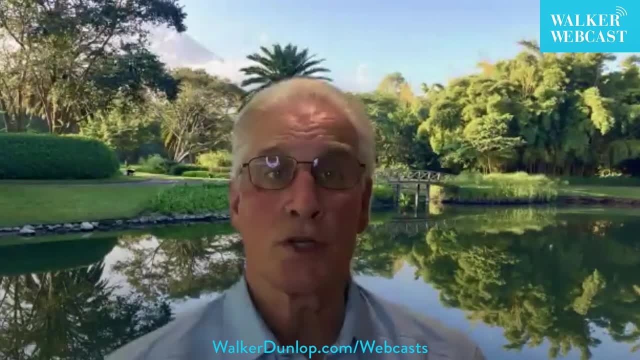 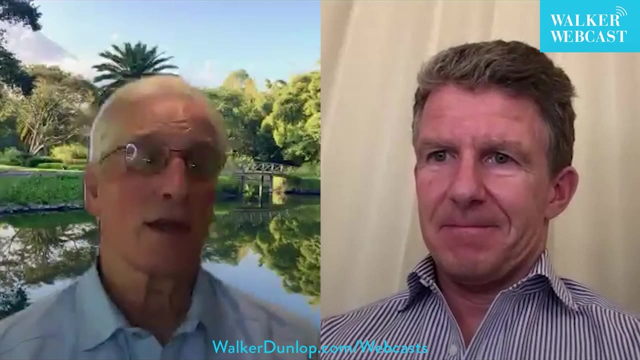 The really good buildings that have long term leases with good tenants, OK, Right, The kind of Boston properties, kind of properties for lack of better, They're OK. That's about the best you can say. It's hard And until people decide they really want to work in offices, it's going to stay hard. 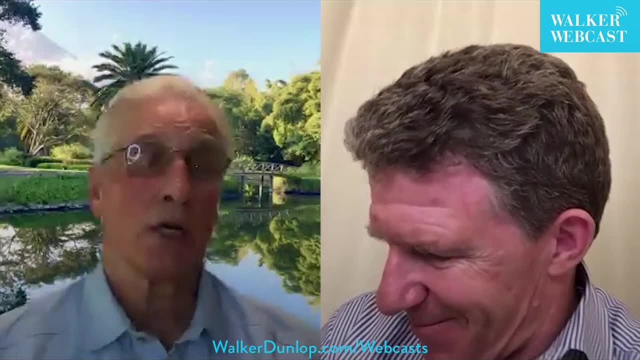 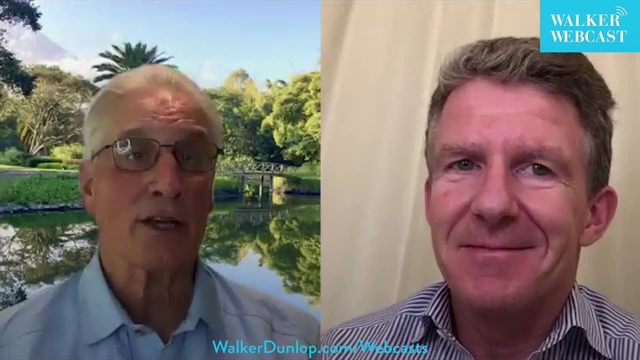 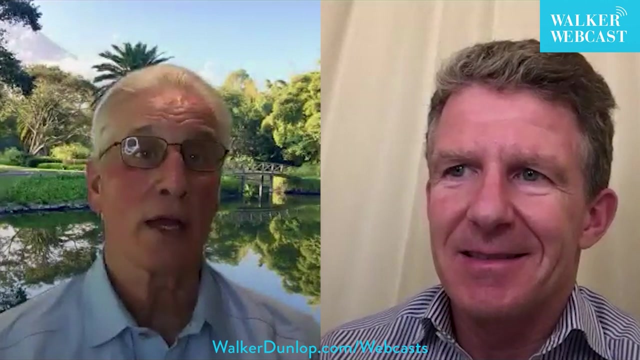 So I still believe they come back Interesting. You know, I was just. I'd be curious in Dubai if you could do me a favor While you're there, ask what the returned office is. I asked this in Casablanca the other day and the answer is everybody. 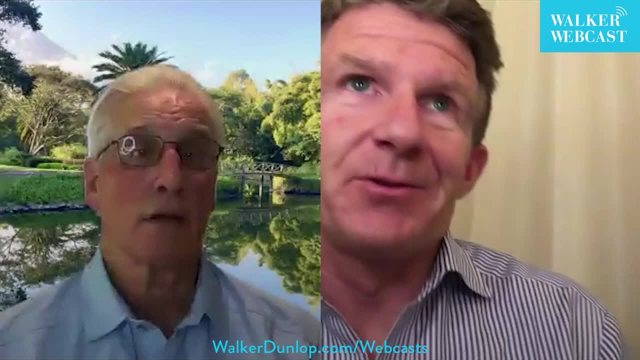 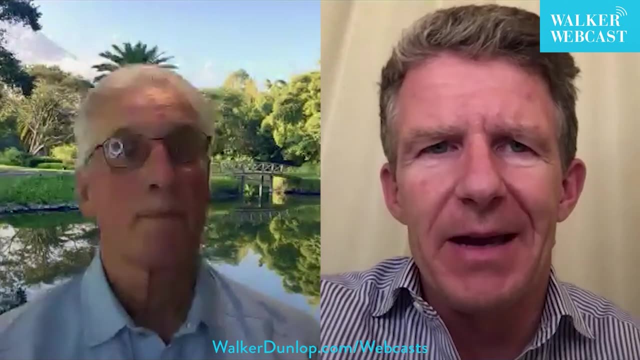 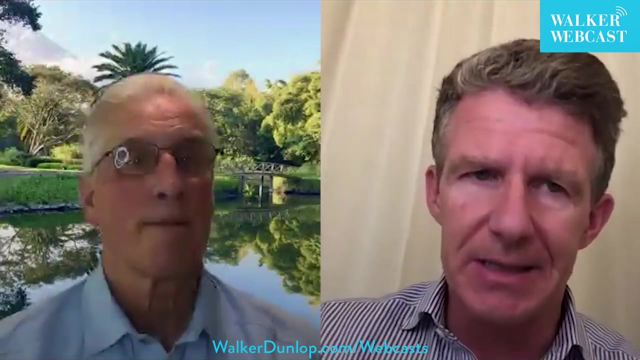 I'm sure everybody. I mean it's just. I mean driving here tonight was just incredible, But it's just. I mean you're out of construction and everything else going on. But let me double click for a second there, Peter, on the banks, because a lot of the questions that came in before this call were about bank default rates, delinquencies and when the sort of crisis hits. 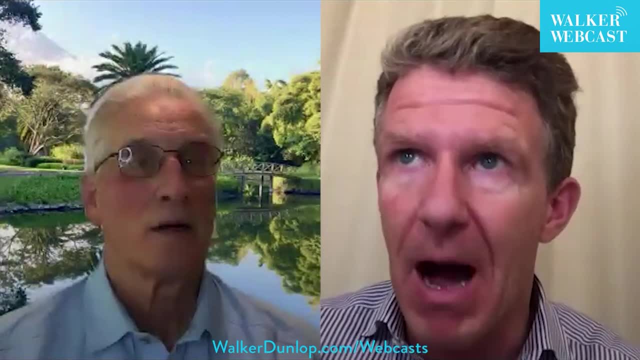 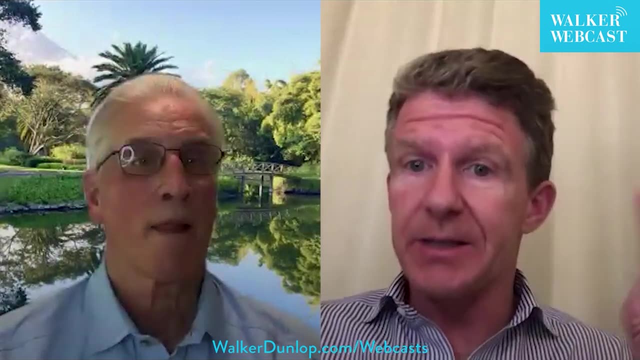 And you put in the letter some data points that I think people have to Keep in mind to understand where we are today and where we were in the GFC, because a lot of people like me sit there and say, oh, crisis in the commercial real estate world looks to me like the GFC. 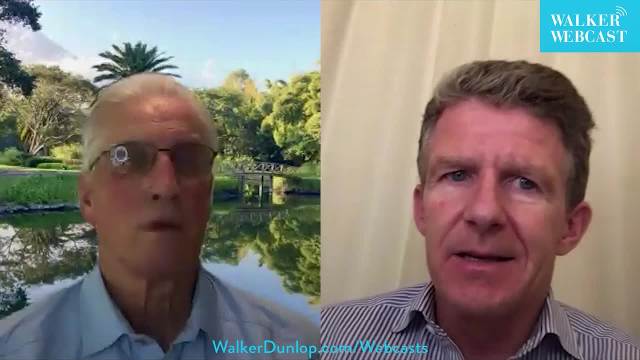 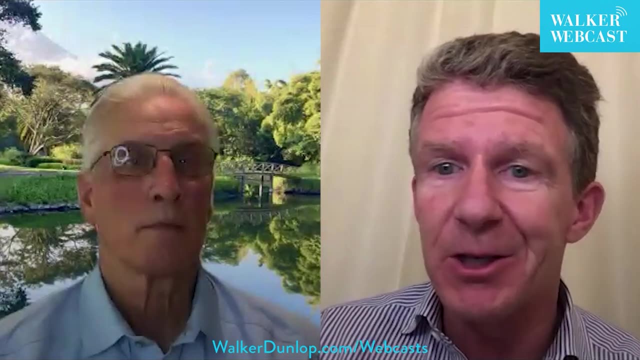 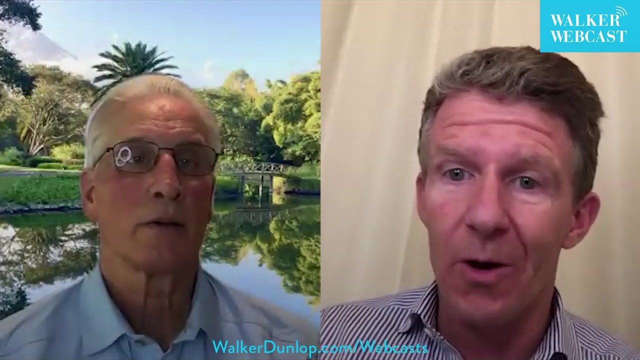 OK, so on, on, on, on, on banks charge off rate of six basis points in Q3 of twenty three, six basis points, which compares to two point eight percent, or two hundred and eighty basis points in 2009.. OK, quarter to quarter: Two thousand nine. 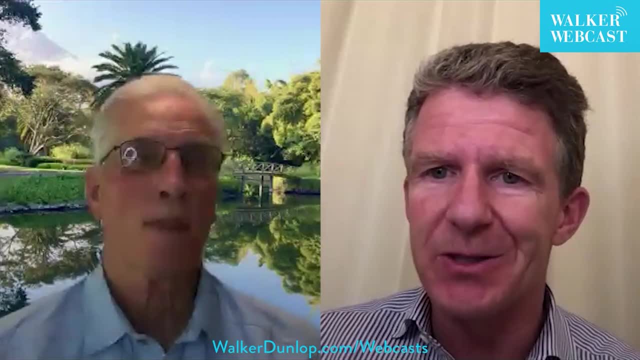 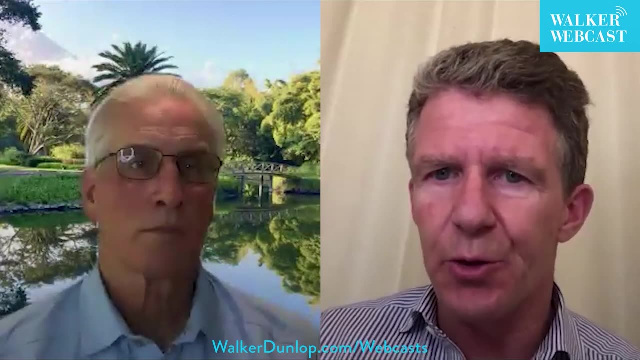 To today, six basis points versus two hundred and eighty basis points, so not even close as it relates to charge offs. And then delinquency rate was one point, oh, seven percent in Q3 of twenty three, which compares to eight point nine percent in Q1 of two thousand and ten. 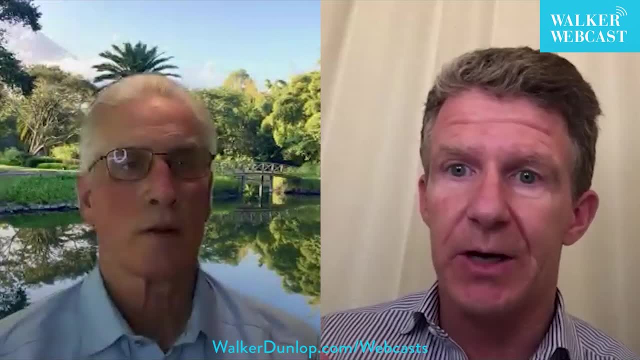 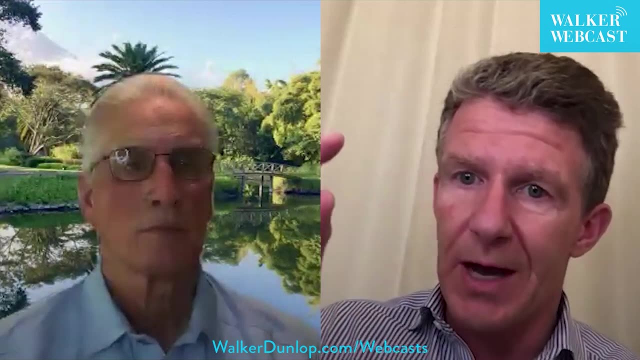 So I think a lot of people sit there and say bank balance sheets are really stressed right now and they got a lot of exposure to CRE and office and all that stuff. But if you just look at the numbers in Q3 of two thousand and twenty three versus Q3 of two thousand and twenty three, 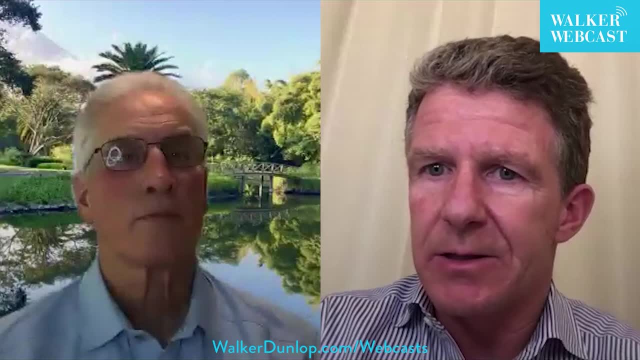 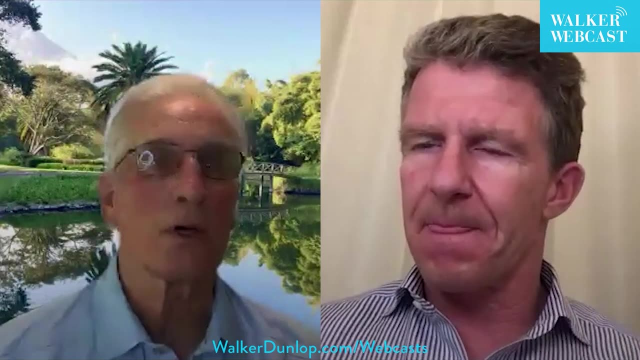 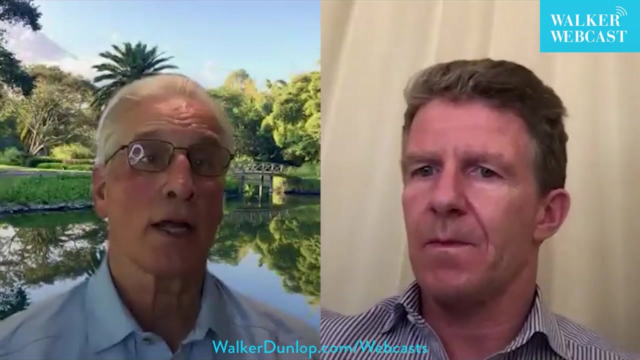 Two thousand and nine in the midst of the GFC, it's, it's not. I mean it's not even, it's nothing close. So it's not close. And they know, and they know the government has their back. If you go back to two thousand early, late nine, early late eight, early nine, you didn't know if the government had your back or not. 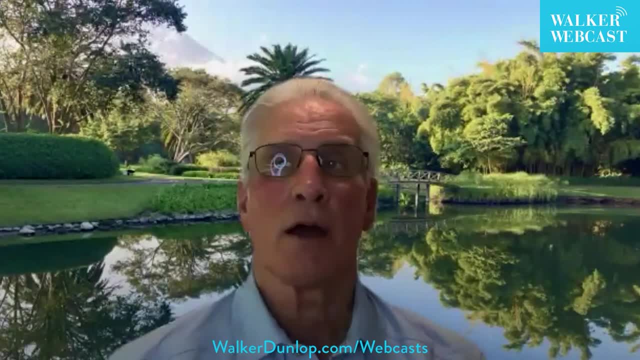 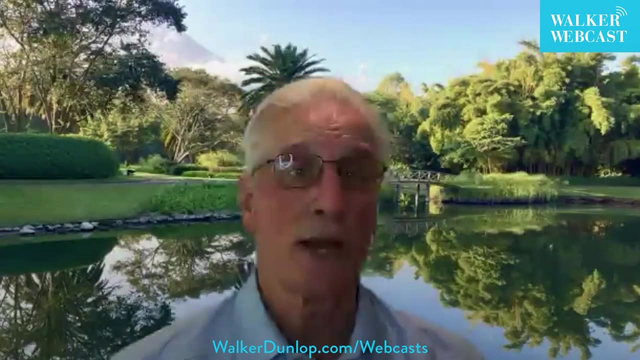 You could have an interesting discussion whether you were good. I think all everybody knows that the government's got their back. May not know exactly how the government's got their back. They have a lot of excess reserves. We saw when SBB happened that they weren't going to let depositors lose money, et cetera. 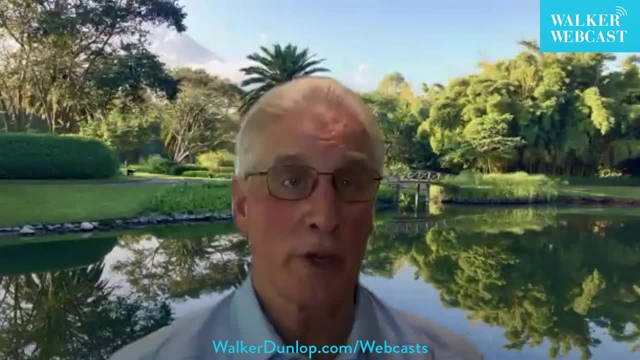 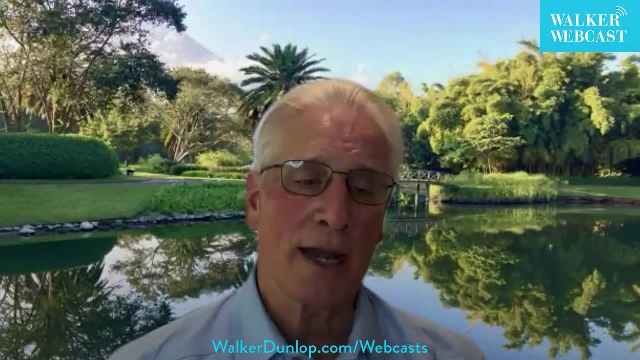 I'm not arguing whether they should or shouldn't, We're just arguing did or didn't. And then you add to it- and I have the numbers in Lindemann letter. People just lose sight of the scale of single family mortgage market Versus all. All of the rest of multi, et cetera, And single family is like four times the size of everything else put together as a mortgage market. And also remember that when the single family mortgage market got in trouble, that was the GFC. Ultimately, the typical down payment, the typical loan devalued was like ninety, eight, Ninety, nine, Nine percent. So any loss just blew right through the equity. And if you look at office, yep, right now there are, let's say, office values are down 50 percent for a number. And let's say they had a 60 percent loan. Well, the first 40 of loss was absorbed by the equity Right, And that wasn't the case with the single family. because of the liar loans and all that stuff, It blew right through the debt right away. 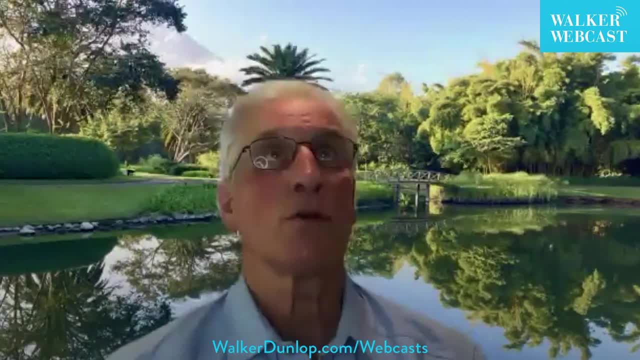 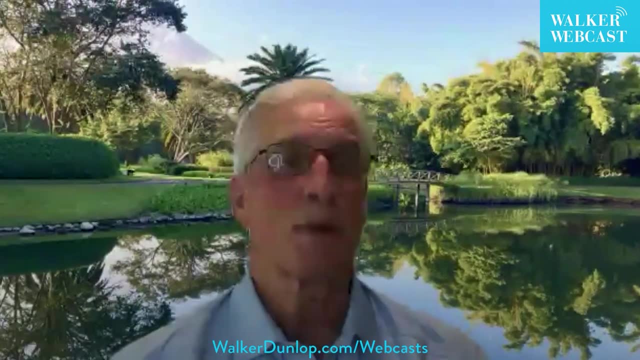 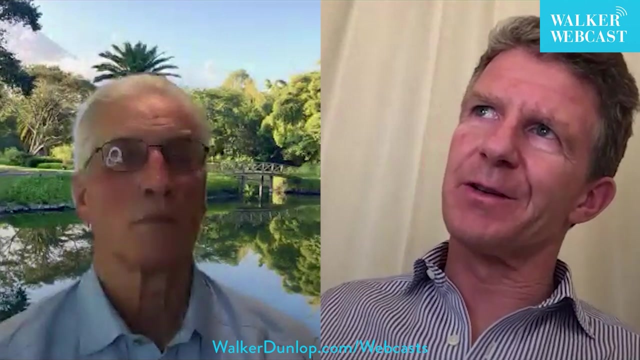 It was a massive number, You, it's not to say there aren't going to be problems, It's that they aren't of the magnet. It's just impossible to be of the magnet. Yeah, you, just to size that you know, there's about four trillion dollars of commercial real estate debt outstanding. There's over 13 trillion of single family outstanding. I mentioned in a moment ago about office that there's about 80 billion dollars of capital Capital that's in construction of new office. today You put in the liniment letter that your estimation is that in 2024, there will be between eight and nine hundred billion dollars spent on new single family development. 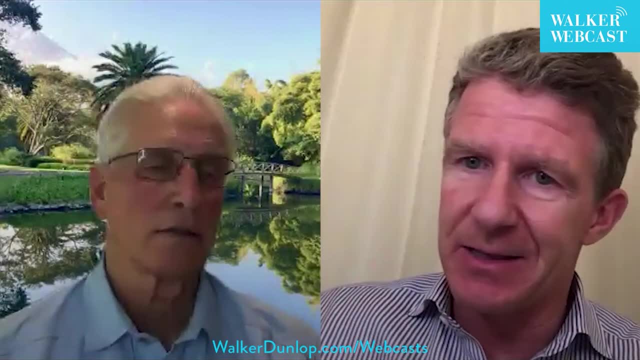 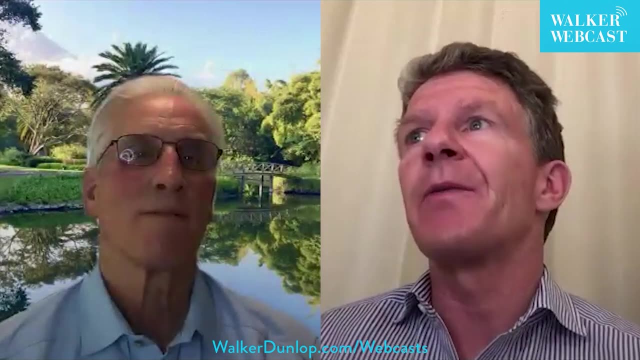 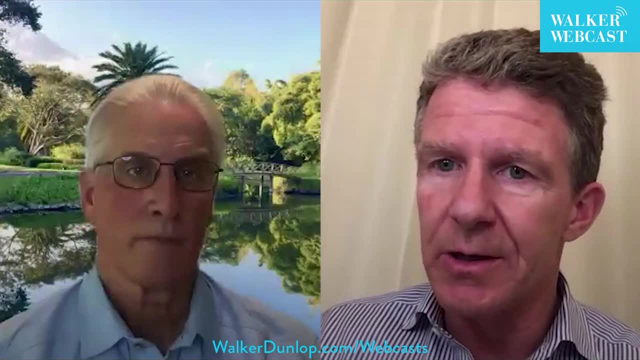 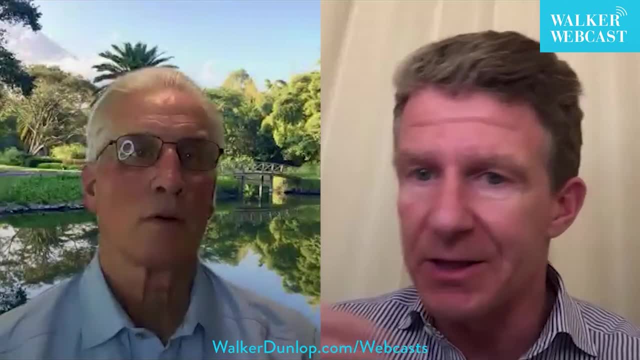 And you're pulling almost a trillion dollars of investment out of the market, Whereas you pull $80 billion of investment in office out of the market. let's just say no one ever built another office building in the United States. It doesn't move the needle as it relates to GDP growth. 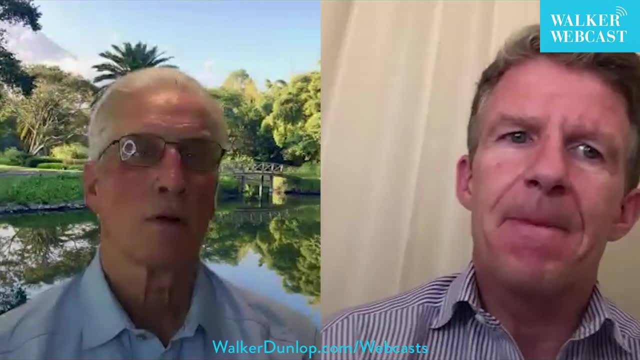 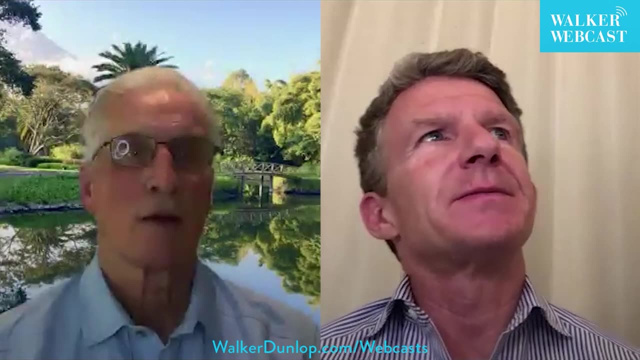 Right, It's a totally different. It's a totally different scale, just totally different scale. So, on supply of single family and multifamily, I think you have what I would call reasonably conservative estimates as it relates to new development over the next couple of years. You have essentially single family at 1.1 million new homes in 2024 and then flattening out at a million new homes for 25,, 26,, 27 and 28.. And on single and on multifamily, you have 350,000 deliveries in 2024 and you basically leave that 350, you bring it down to 300. 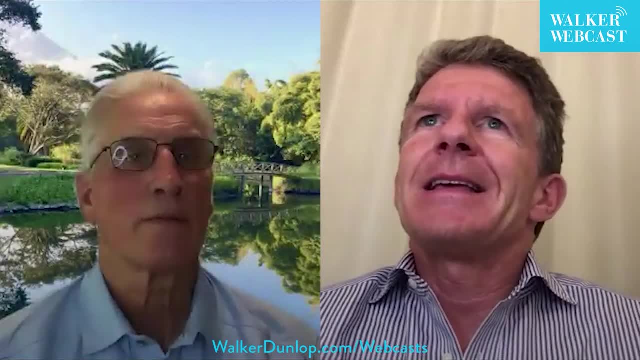 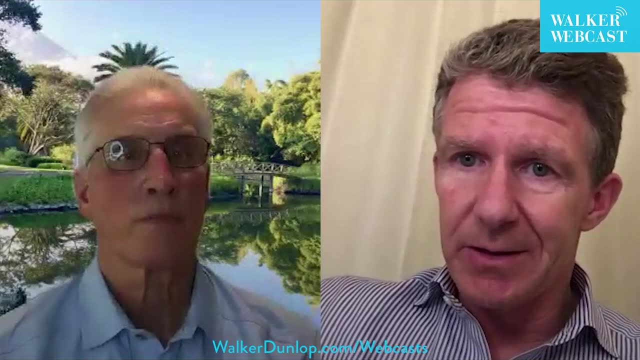 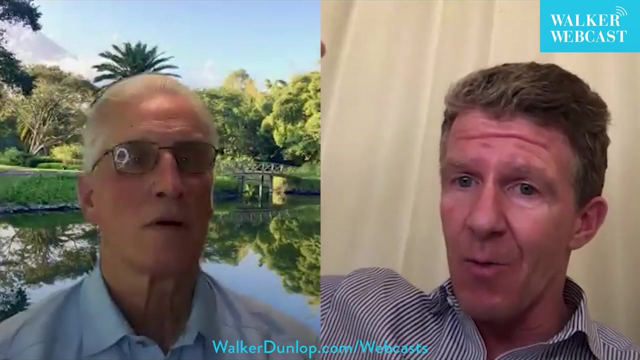 And I guess my question to you, Peter, is this: If you get multi stepping down from 650,000 deliveries to- and you mentioned it briefly in the letter- that it's probably more like 250,000 in 2025, given how much it's fallen down as it relates to new 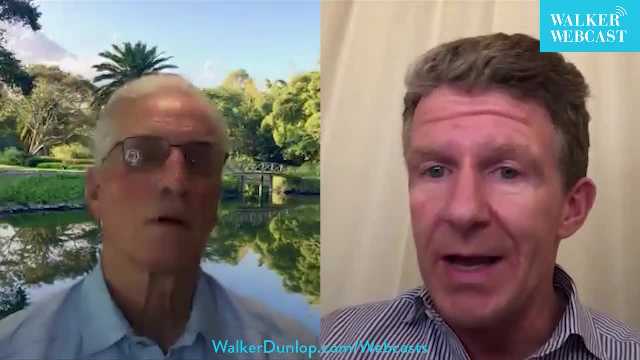 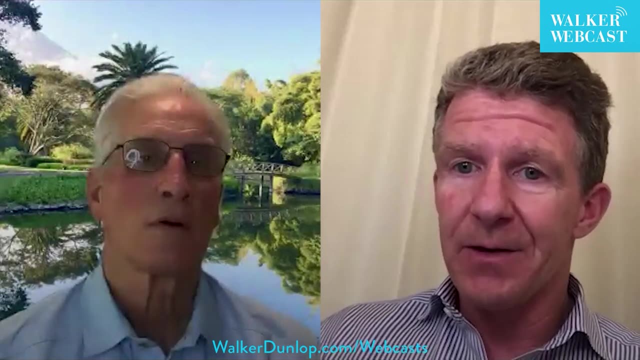 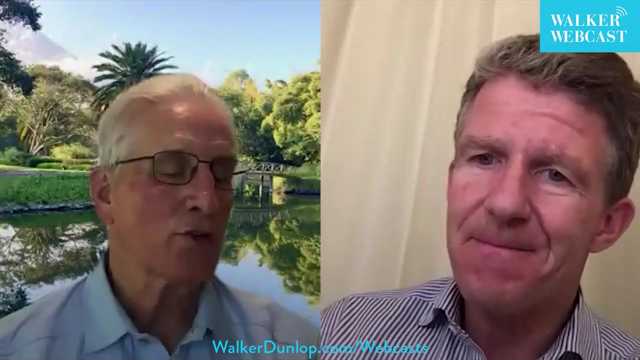 Shovels in the ground. The concept there is: rents move. You think that when rents start to move and get back to significant growth again, that you're going to have new deliveries stay static at 300,000 for the next years? Yeah, The answer is not really, but it's. I can't get that sharp a pencil. 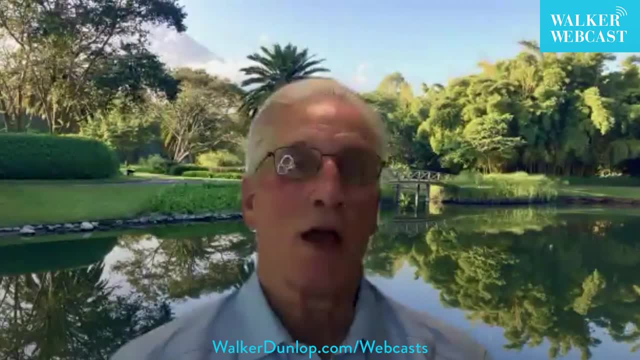 I mean, I'm just being honest. you know what I'm basically saying, is I? The rest of this year is going to be real tough for multifamily. The thing that keeps it as strong as it is are various subsidized and so forth. Product as opposed to market rate next year. first half will be slow, second half will pick up because the worst of the spirit of supply will be over, the worst of the rental adjustment will be over and will be more normalizing. We've done some work on that. We'll have that in a future issue. Single family, I think, is a different story. I think single family has become difficult to get much beyond about one point one million units, and that's because of NIMBY ism. So let's suppose just you know. I think everybody agrees there's a shortage of single family homes. And it's as represented by the home prices keep outstripping inflation for over 10 years. now, right, And notably outstripping it. If let's just say my number is like three and a half million units single family short, let's just assume I'm right, Okay, And we need about 1.1. million just to deal with normal population growth et cetera. Imagine the home builders showed up and said: we want 4.6 million. We're going to build 4.6 million units in the next 12 months. I don't think. I don't think communities would allow them, I just don't think they would. 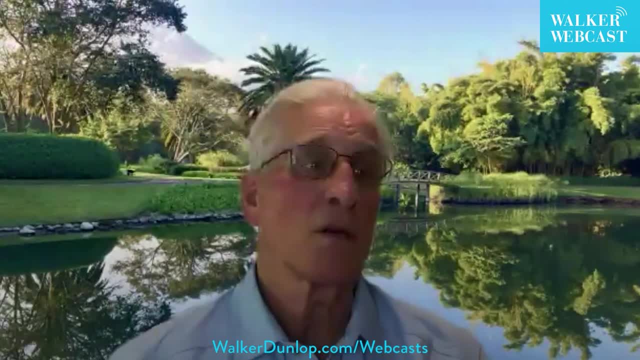 allow it, I think they might allow them to do a million, three million, two. I think the framework of NIMBYism is very different than we've seen in the past on some of these ups and it dampens it And let's say it's a 3 million shortfall, Even if you made it up 300,000 a year for the next. 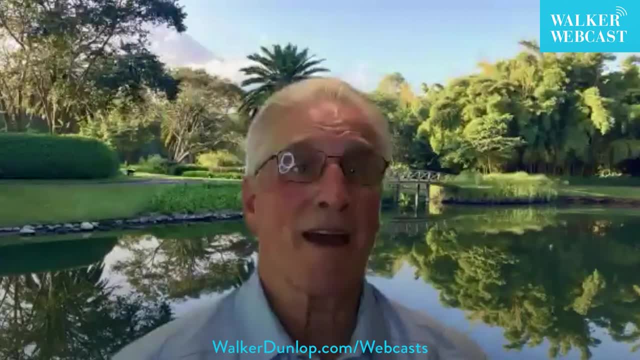 it takes a decade to chew through it And I just don't think NIMBYs will allow it to be a big catch up. And that means that we were in a kind of permanent position of single family home prices are going to go up notably faster than inflation. 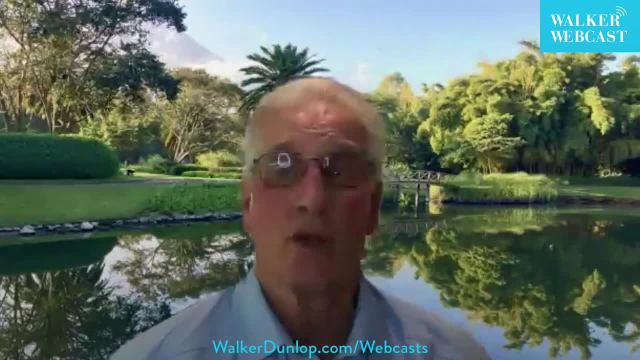 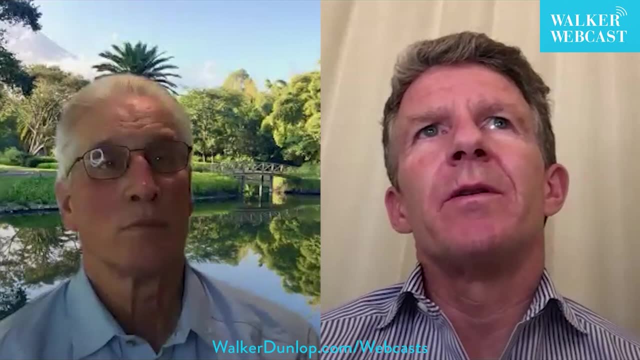 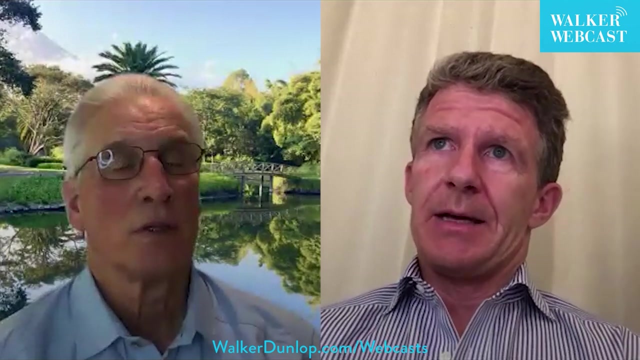 but we just don't have enough housing units. It's something people want, So I think that the let's talk for a moment. You have some really good data in the letters that relates to private REITs, and then your CAPM model on REIT valuations. As, as you know, 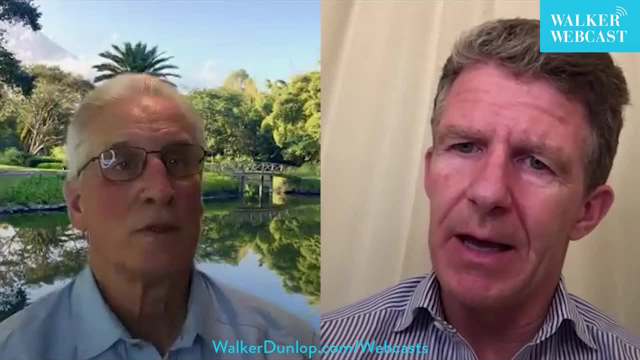 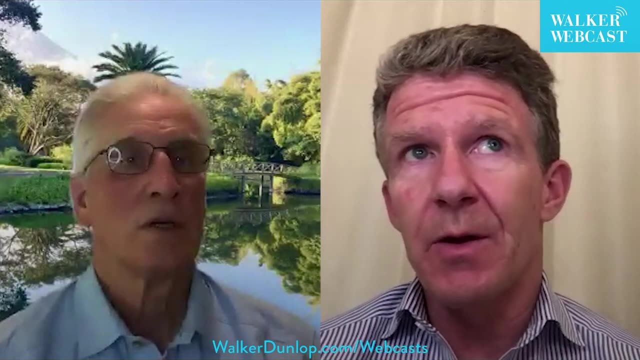 well, Blackstone bought Air Communities on Monday at a 25% premium to their trading stock price. I think the cap rate, the underwritten cap rate, on that deal was a five, nine cap rate. It. it. it makes sense, if you will, if you look at the data that's in the Lineman letter. 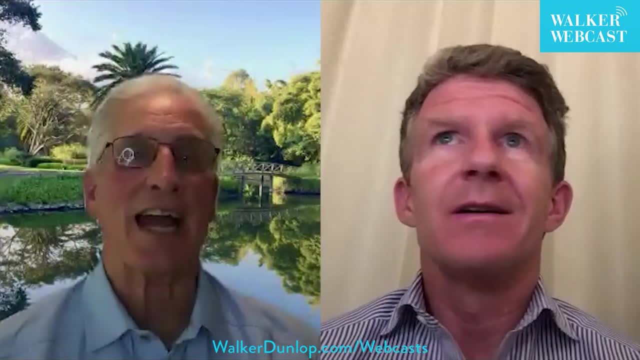 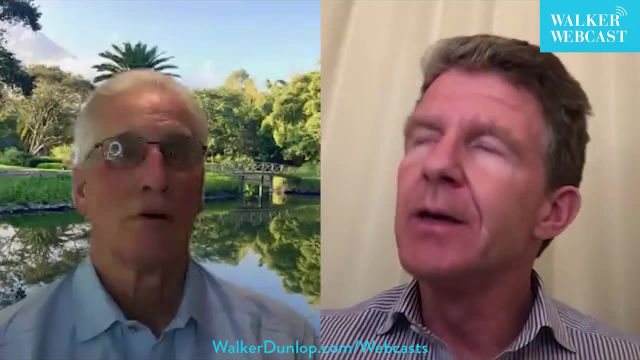 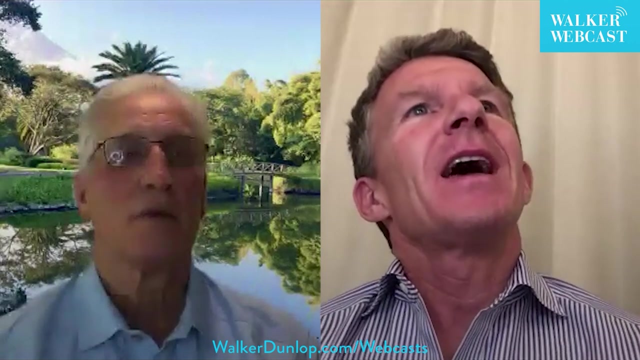 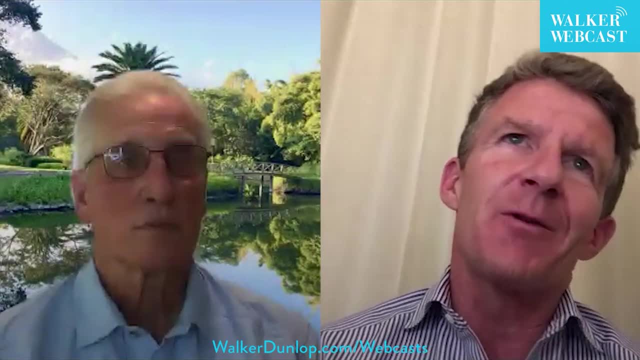 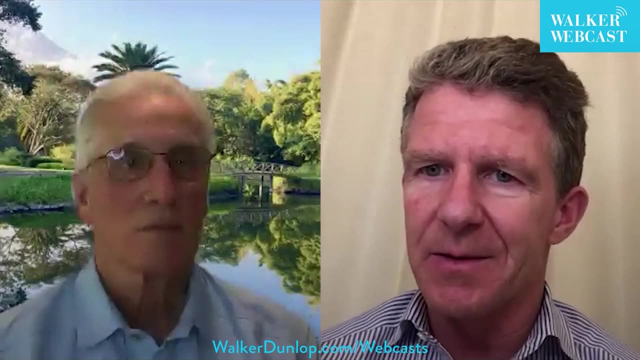 Is this where the market starts to turn again the light that's coming through the clouds, And I think I was going to be coming into this call today if we'd gotten a decent inflation print and we didn't have a 451 10-year saying yeah, things are about to really get going. 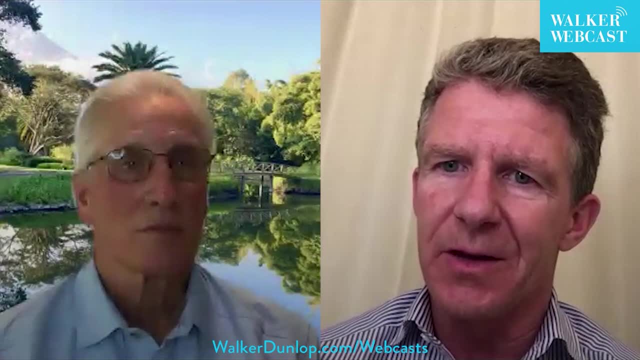 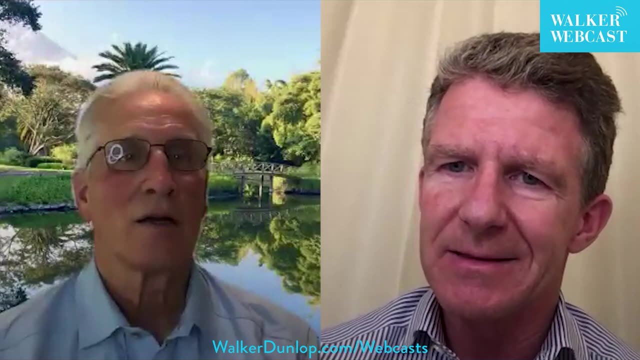 Should we be focused on Monday's deal And that is the beginning of the next phase, Or does the 451 put everything on hold again? Yeah, you know, I think you're going to look back and view that as the beginning of the. 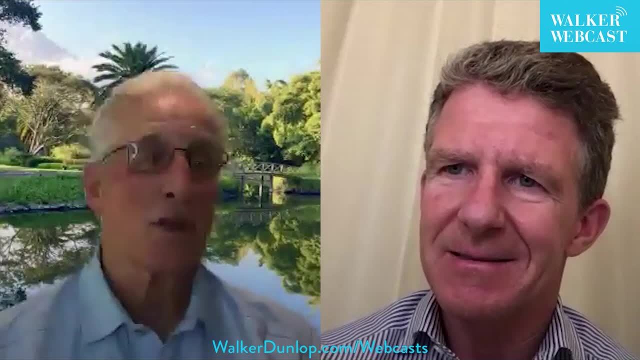 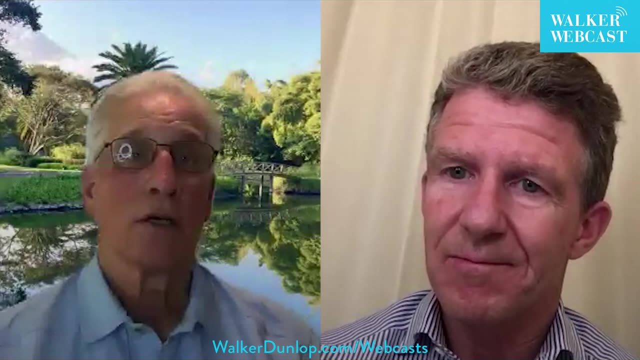 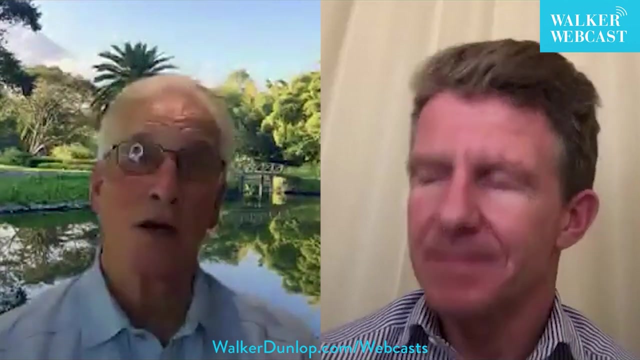 end. Right, That that was the beginning of capital. coming back to real estate in general and maybe to public companies specifically. Now obviously it's going to go private, but to the arbitrage, if you will. that's been there and it really is there. 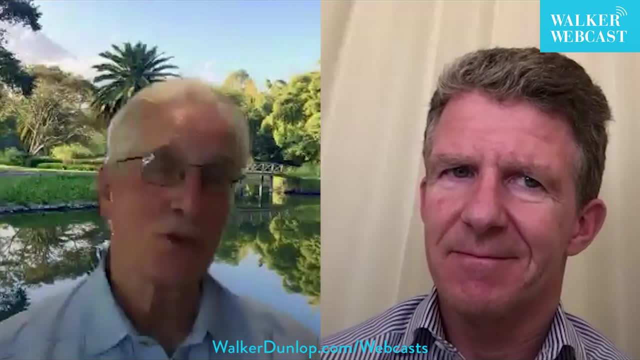 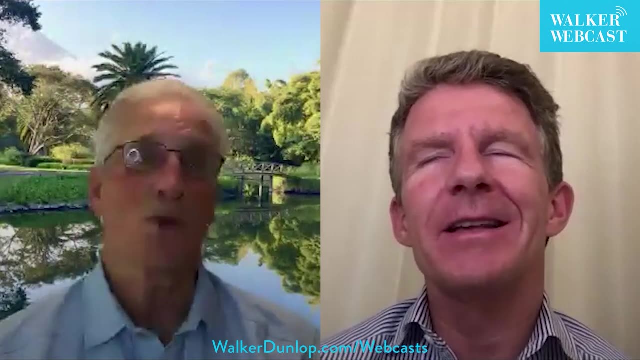 And yeah, it is funny, I did the same math. It almost is exactly where I mean. it's not like my stuff's rocket science, right, It's a broken down old PhD. It's uncanny how closely the numbers lined up as it relates to where you are on both. 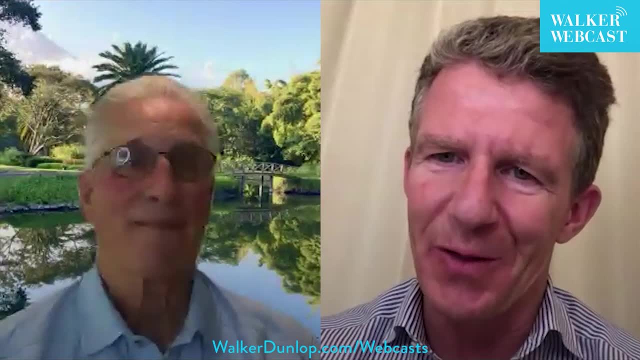 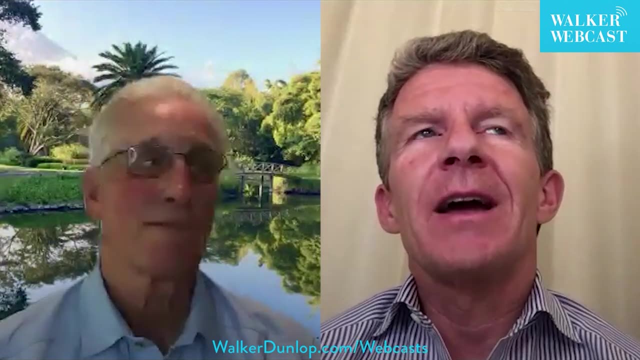 cap rates as well as the public private discount. Let's just, let's just put it there, which is, which is basically: it says the deal works. It says you know it was underwritten. Well, I hope you're right And I would say this, that the B? REIT met all redemptions in February as well as in March. 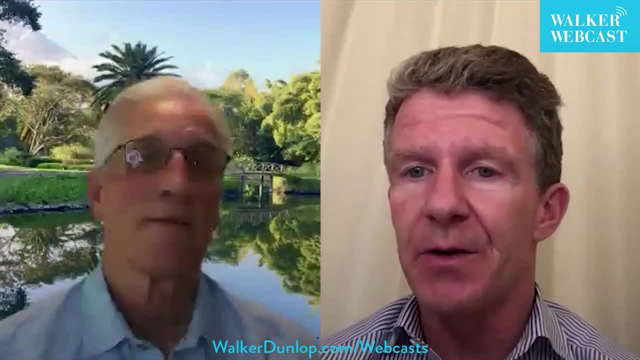 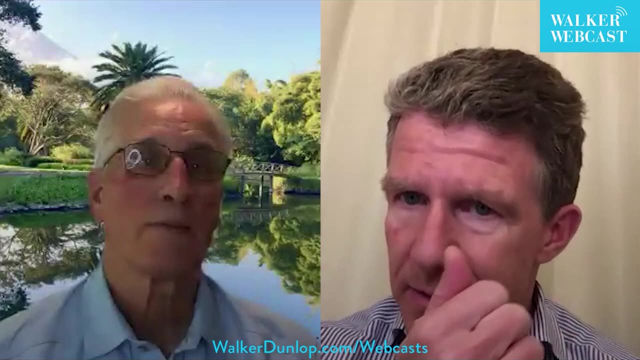 and meeting redemptions And the redemption queue I do think is a very significant point as it relates to equity capital having flown out of private REITs in such a massive way and now meeting the redemptions and then turning around and starting to be inflows that will allow for more capital. 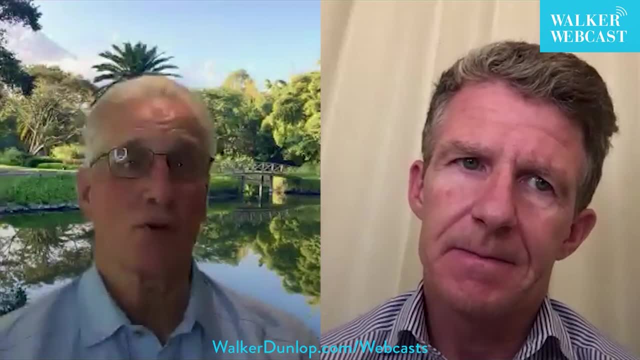 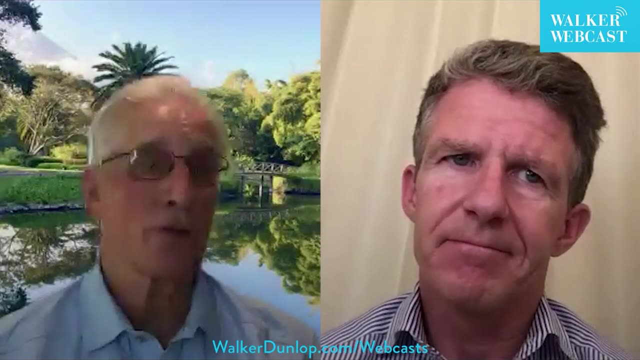 to come into the system And, as you know, I basically view cap rates movements as flow funds and and the B REIT and the S REIT and so forth, as well as bank lending. You could say it all got triggered by Fed. Policy, but in previous times it didn't get triggered by Fed policy. It got triggered by housing and the way we were just talking about the GFC, et cetera. Anytime money disappears, real estate suffers because it requires a lot of money. 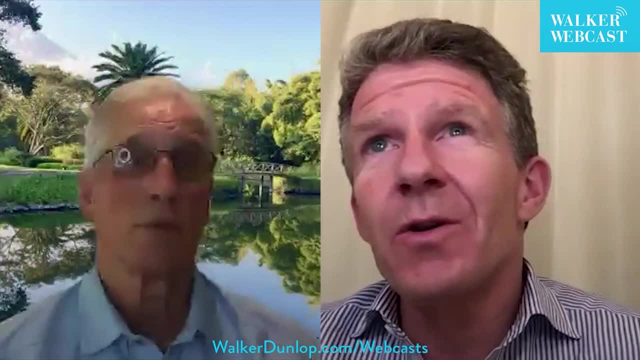 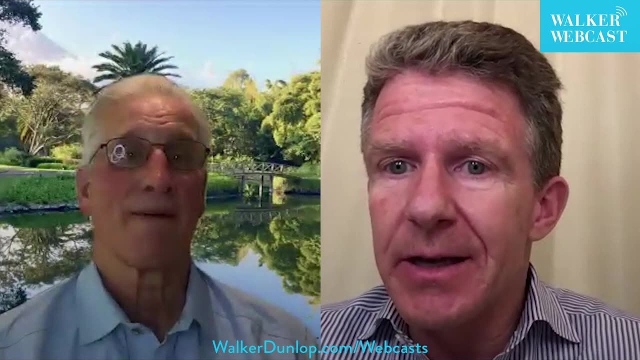 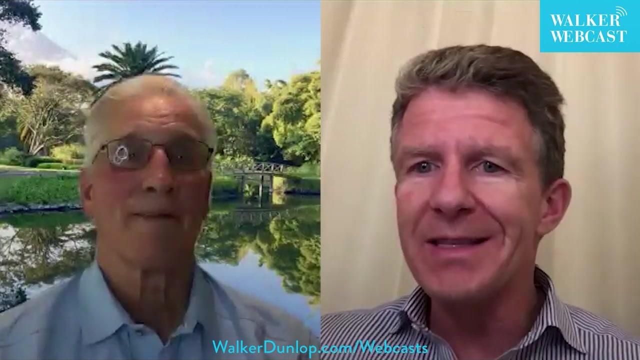 And anytime money comes back, it does well. And I will say, though, your, your, your Lineman real estate index number for Q4 scares me, because it's an, it was a, it was, In my view, too good a number in the sense that it's at 150,. OK, so you got 170 in 2009,. 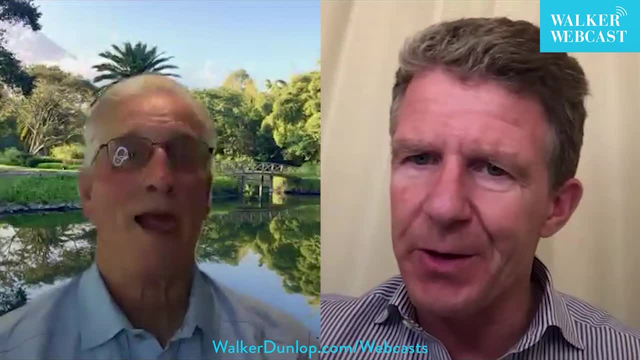 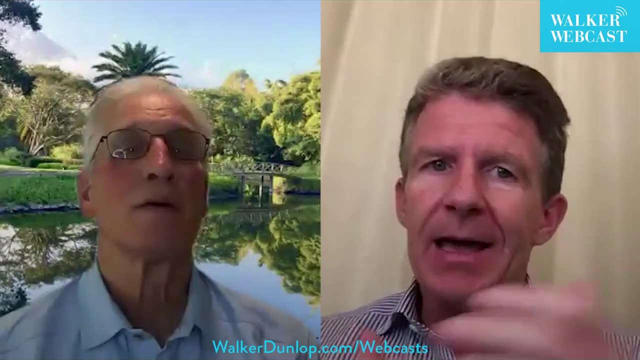 OK, and then the LREI drops down to 133 in 2014.. So that's sort of that brackets it as it relates to the worst point where it was really great- And it's been at 150 in 2018 and 2019- that it moves all over the place because of the 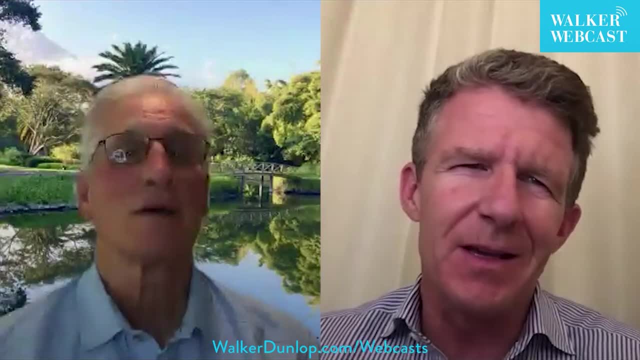 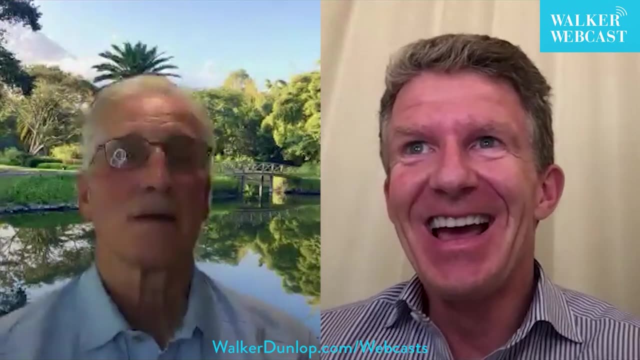 pandemic, But in Q4, it was back at 150, 151,, I think, was the specific number, And I'm And they're going geez if Q4 2023 is a 151 Lineman real estate index. that's quote, unquote. 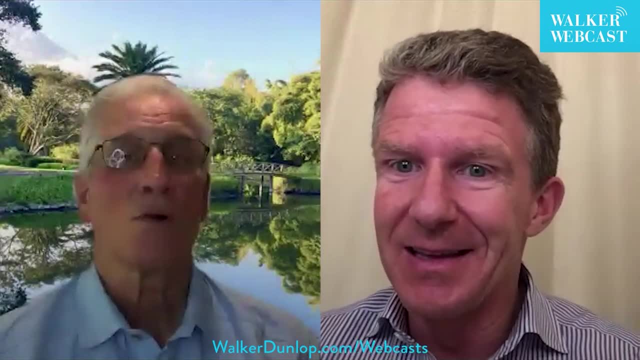 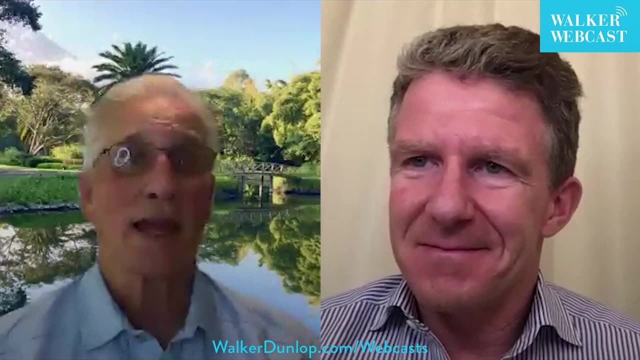 normalized Q4 did not feel normalized in any way. Wait, wait for what's out there with all the dry powder. Wait for what's out there in the people recalibrating denominators. Wait for what's out there in terms of banks: have a lot. 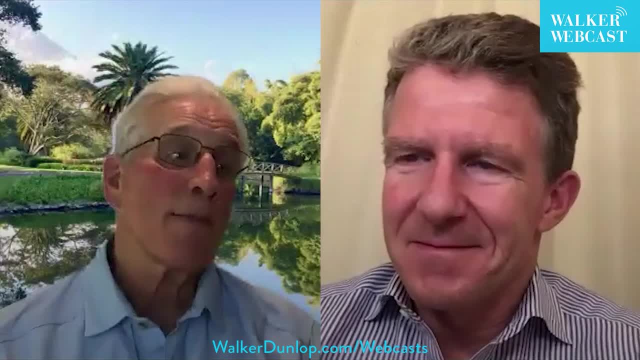 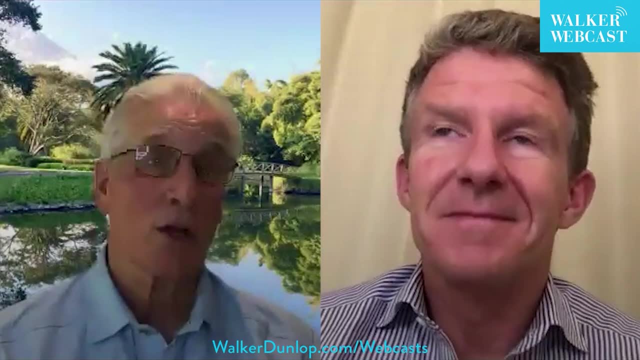 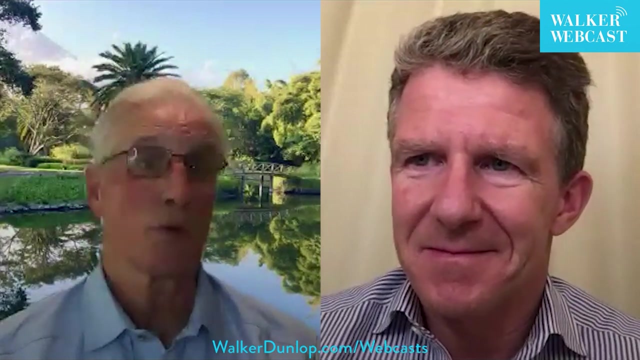 The major banks have a lot of reserves And remember. meanwhile People are buying insurance policies and they have to be put to work by making loans And you know the growth occurs and that growth capital has to be put to use And real estate is one of the places that will get put to use that. 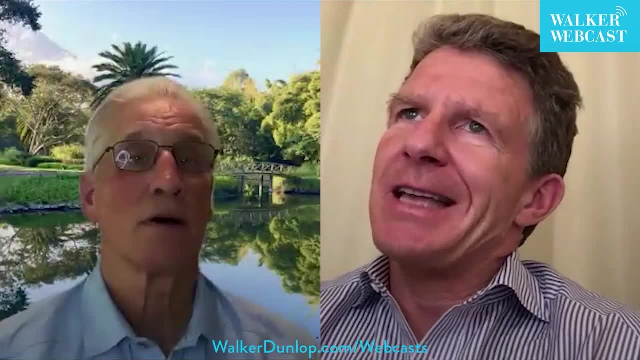 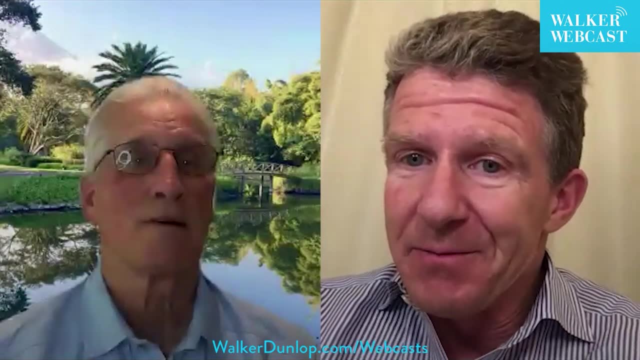 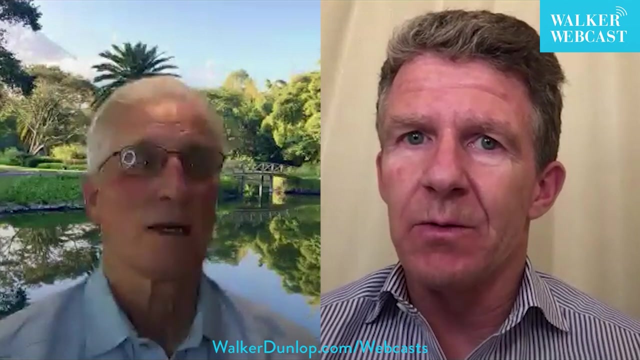 So final point, that you spend some time on and that I just had to get into this call because I've just come from India and you write extensively about, if you will. You know you've got a lot of people who are trying to sell the bad deal of the Paris Accords and trying to bring down global temperatures by two point seven degrees Fahrenheit. 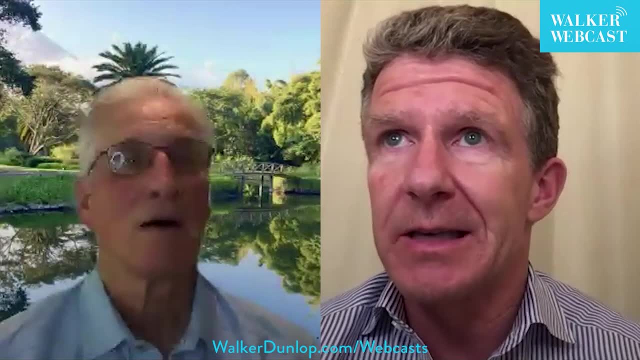 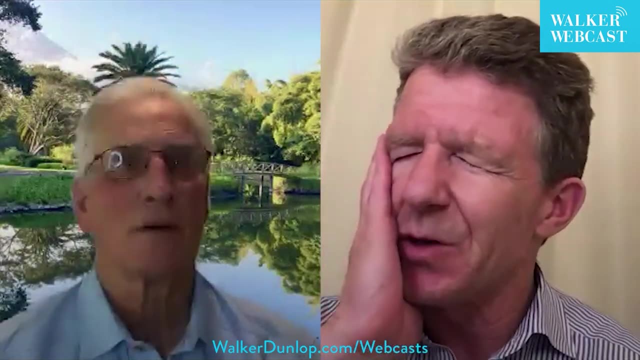 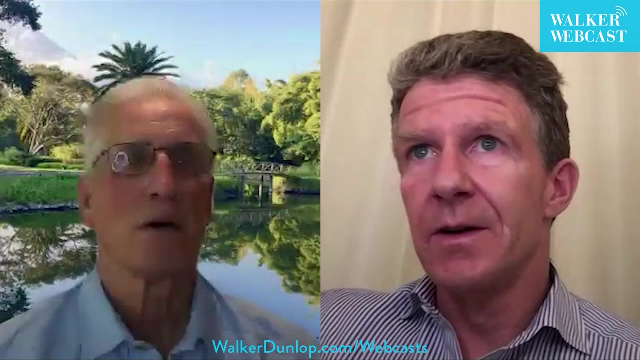 And, if I recall correctly, you basically say that it will benefit. First of all, you go to a big meta analysis by a gentleman- What's his name? Paul, Yeah, Yeah, Paul- who pulls together thirty five reports on the cost of trying to get to the Paris Accord goals. 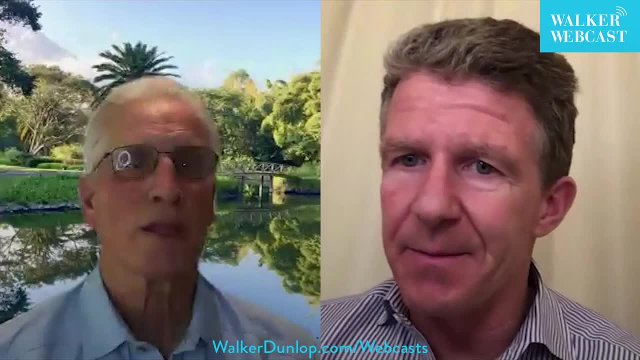 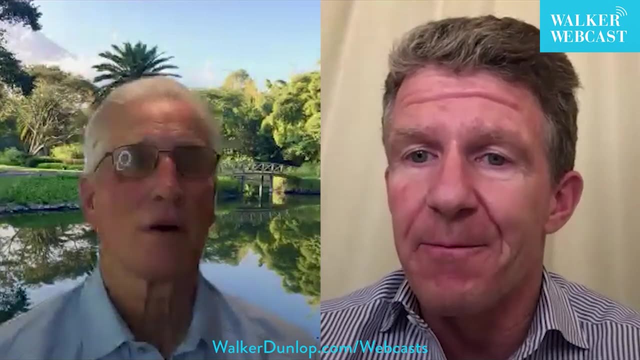 Yeah, Yeah, Yeah. And basically, out of all of that, it basically says that the benefit of trying to get to the Paris Accords is about four to five trillion dollars a year of benefit and a cost of somewhere between twenty and twenty five trillion dollars a year. 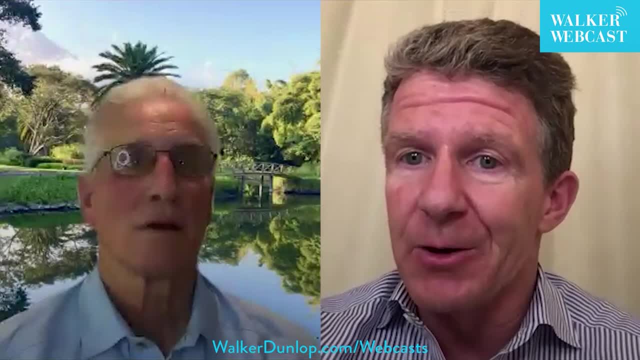 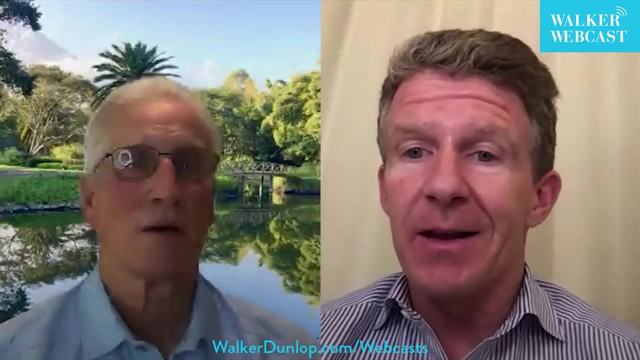 You say basically, on a global economy of one hundred trillion dollars, we're going to lose a quarter of our growth And, given the benefits of it, it ain't worth the investment. And I read it and the math made perfect sense to me. 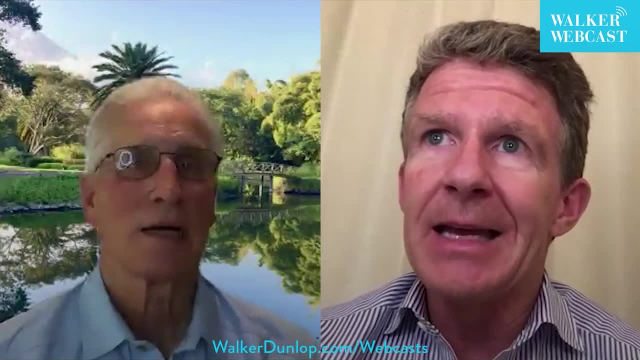 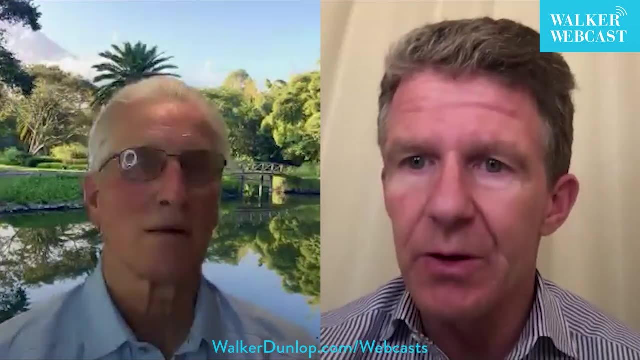 But I just spent four days. I was in India and I could barely breathe. I landed in Delhi this morning, Peter. it was one hundred and two degrees. I didn't see the sun for four days. I literally could not see through the smog layer over India, through the fall through it. 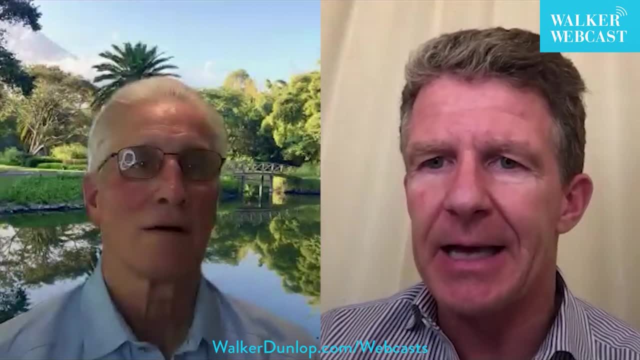 And the pollution index was at one hundred and eighty today. And I asked someone on the bus taking us into the terminal: how bad does it get? Is this as bad as it ever gets? He goes, oh no, it's one hundred eighty today. 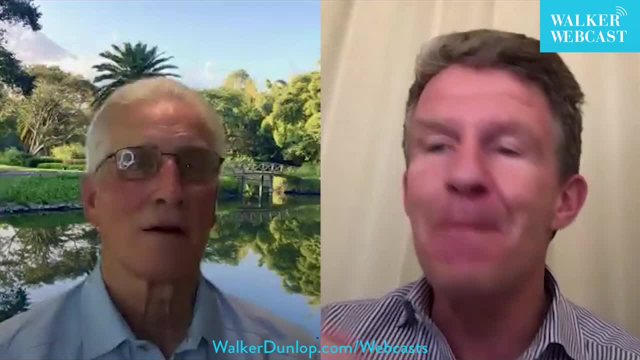 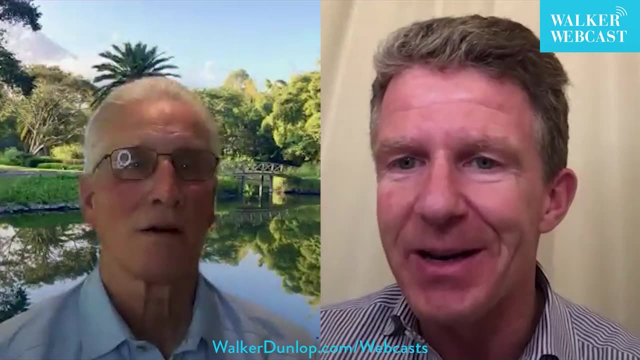 It can get to three hundred. I have to tell you, I cannot imagine what it would it be like to be in Delhi. I can't imagine what it would be like to be in Delhi with a hundred and two degree heat and a pollution index of three hundred. 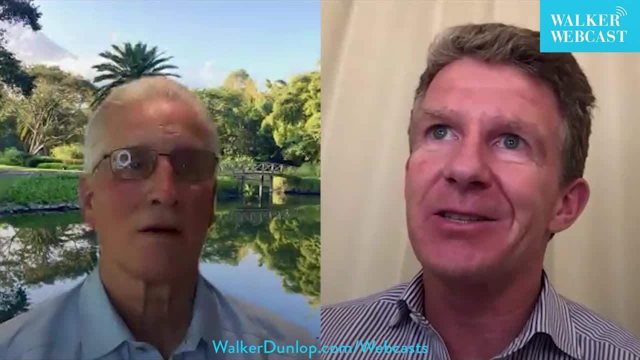 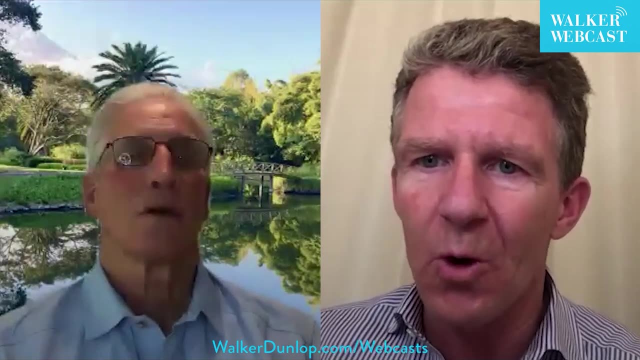 So I guess my question to you is: the math in your report makes sense that it's going to cost a lot and it might not be worth the trade. And at the same time I see Aaron saying who wants to live in the type of world that that one point two billion Indians are living in today? 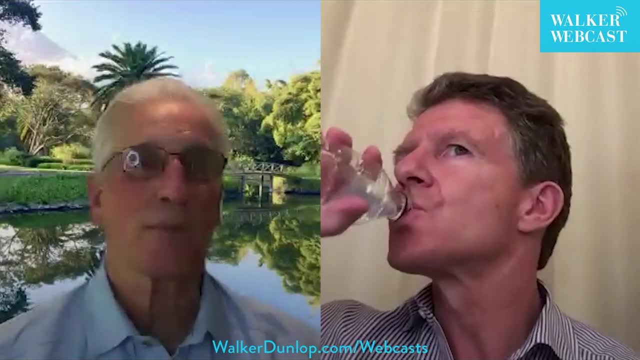 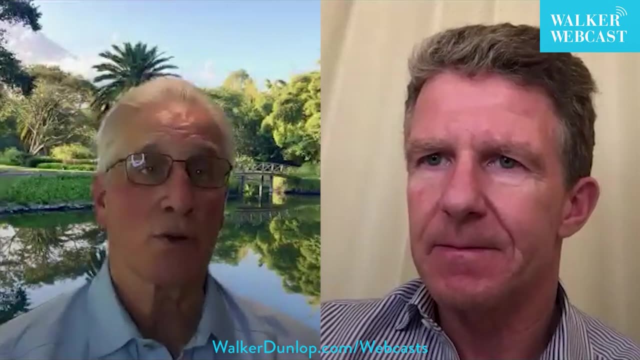 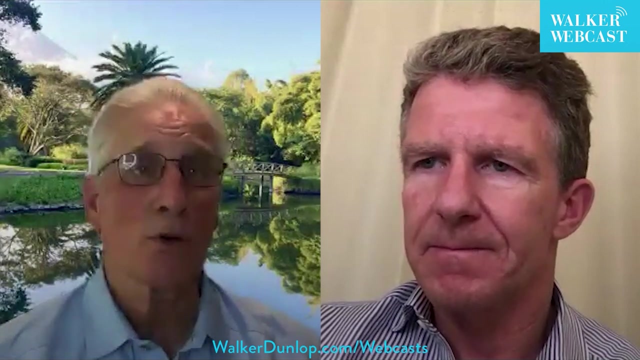 And the answer is no one. And the answer to solving it is very simple And it's economic growth. And I go back. I go to university in 1969 in northern Ohio and the headline for a week, basically as I arrive on campus, is the Cuyahoga River in Cleveland is burning, really burned. 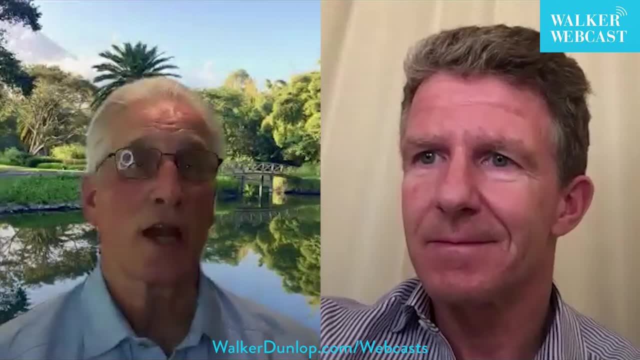 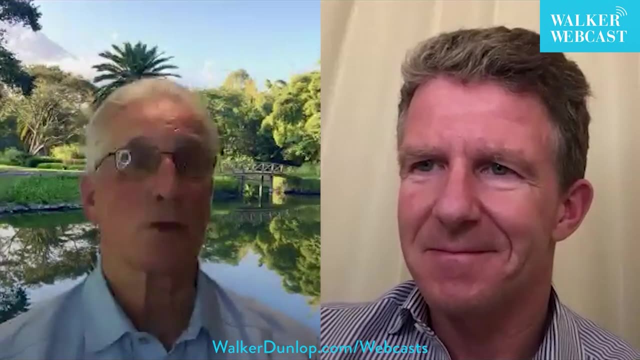 And, by the way, if you've gone to Los Angeles in 1969, the headline or Johnny Carson's quips were: the smog, the smog, the smog. You don't hear the discussion of smog. You don't hear Cuyahoga River burning. 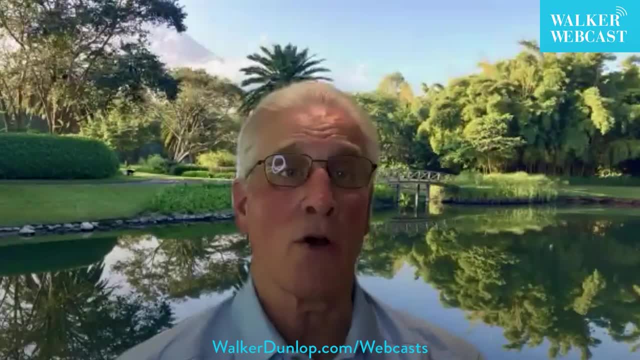 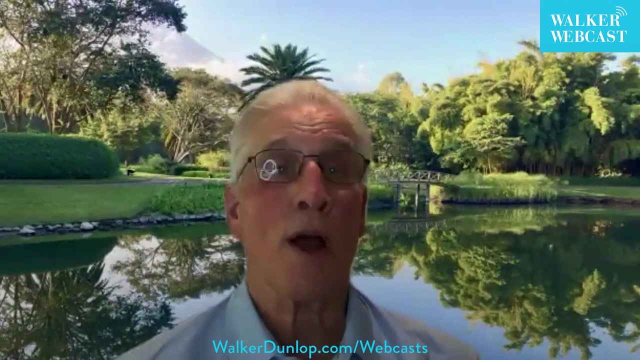 They catch fish, apparently, and eat them out of the Cuyahoga Now, and you know and why? And that's because we grew and we got richer and no because no one wants to live. You said, no one wants to live like that and getting rich enough so that we can deal with those problems rather than just feeding ourselves and clothing ourselves. 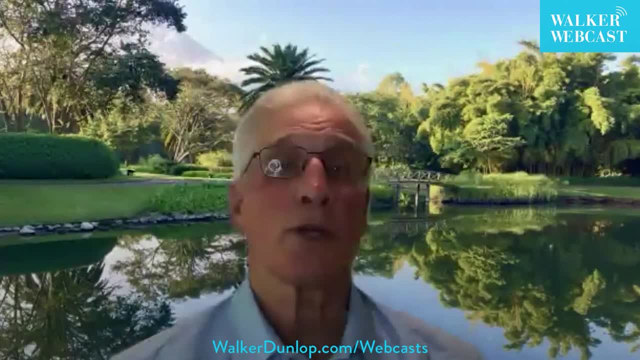 And so we should be trying. my view We should be trying. We should be trying to get the rest of the world as rich- quote- as possible, as quickly as possible, because they don't want to live like that. They would like to have cleaner converters. 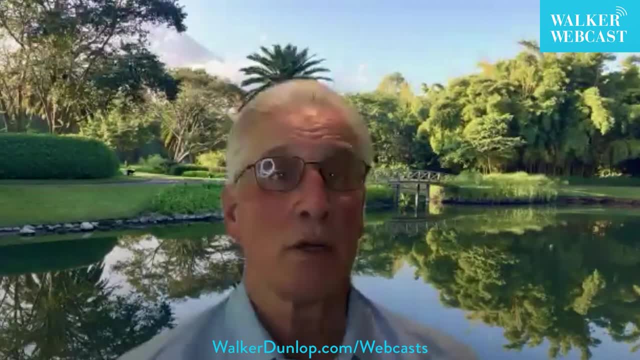 They would like to have all the things that we've done as we got richer. So it's very myopic to think that you or me using an EV is going to solve the problem. The problem is where you saw it and the solution is they need to get richer so that they have the money to do more than just feed their children and send their children to school. 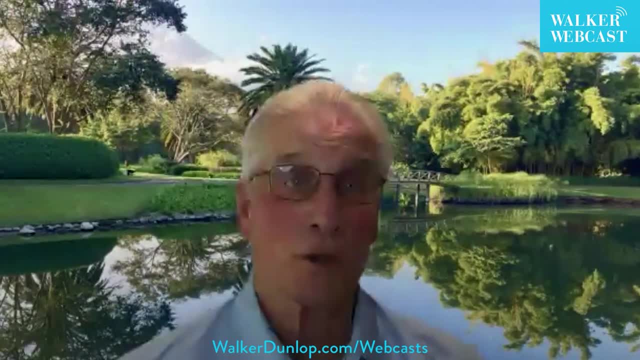 Given the choice of feeding your children, getting your children in school or cleaning the smog, what do you think most people in most places in history choose? Once I can comfortably feed my children Once, Once I can comfortably get them shoes, Once I can comfortably get them educated. 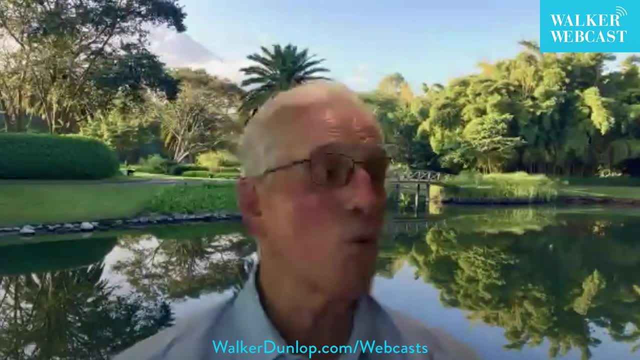 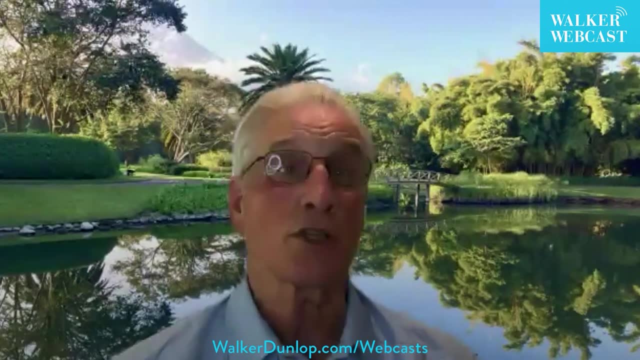 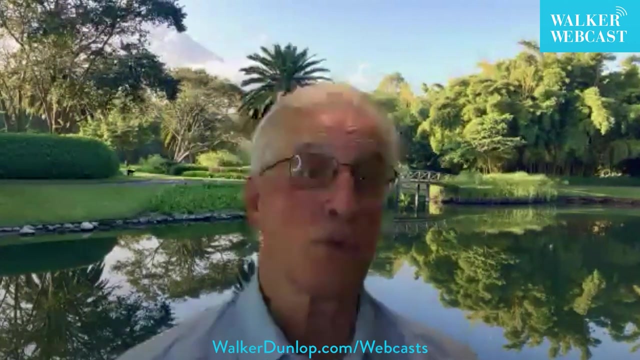 Okay, Things like smog and warming and such, those are. they're not luxuries. They are luxuries compared to I just got to survive. I want clean water, for example, Given the choice of clean water or, which I can die from, non-clean water, right. 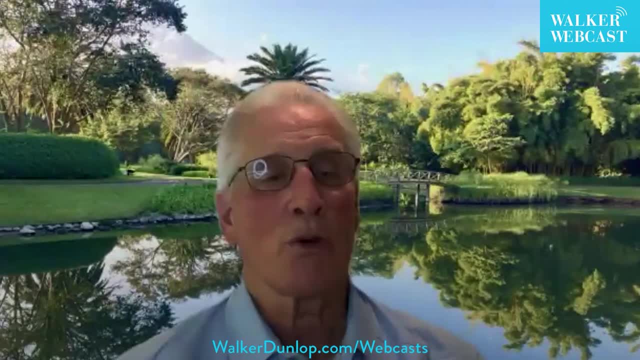 I mean We just have to be realistic that us using a Tesla is going to have any mathematical effect on, I mean, maybe a great car, That's a different discussion- but it's not going to have any effect, any effect that anybody will identify. 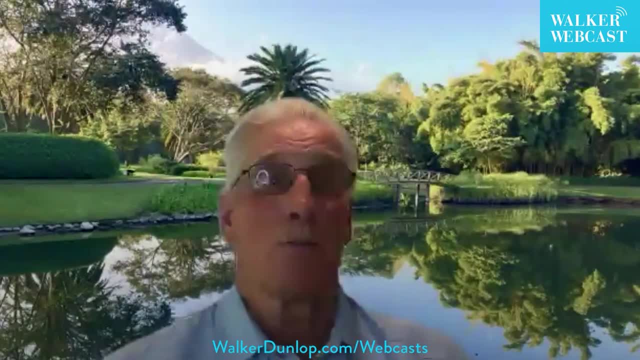 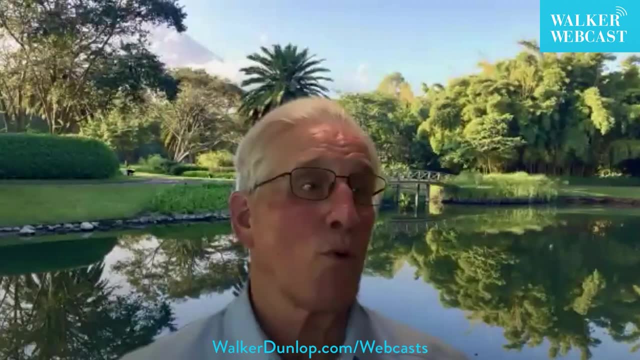 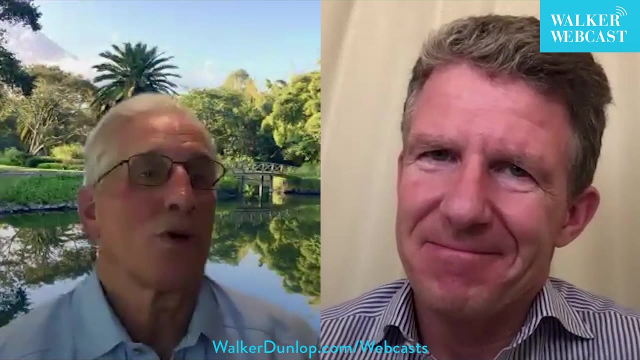 By the way, by the models, by the- not my models- by the models of the people who are proposing it. you know it's like One-tenth of one-hundredth degree. you know doesn't mean don't do it, do it if it makes sense. but where's the real issue? 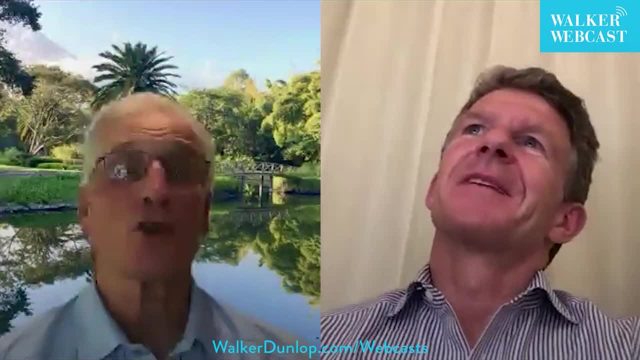 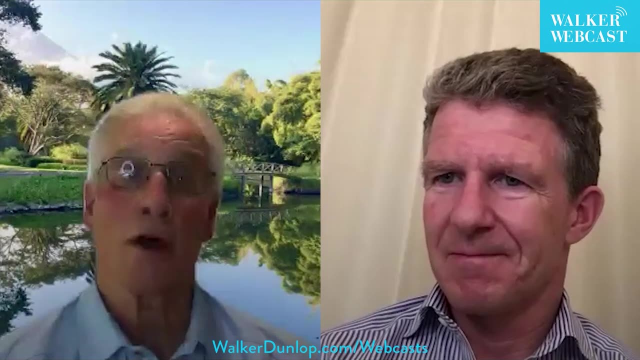 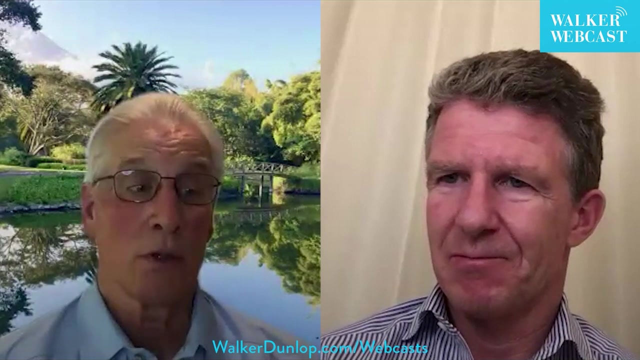 It's where you just came from, places like that, And the answer, unfortunately, is obvious and difficult, Like many things in life: get them rich enough that they don't worry about their children eating or going to school or being housed, And once that happens, the other will come. 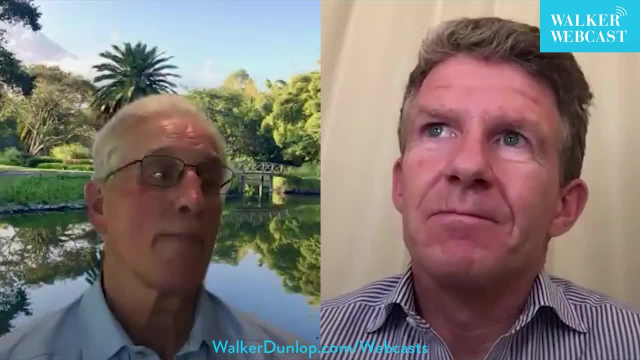 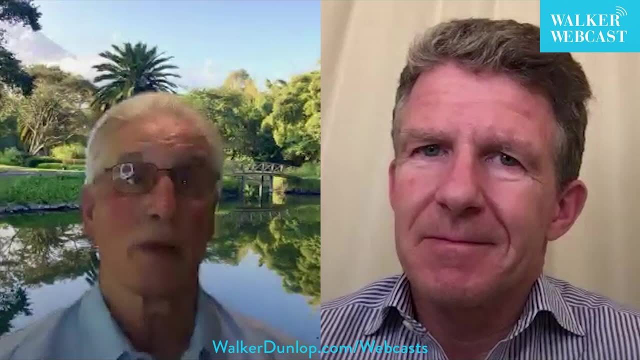 It's had come everywhere. It's come everywhere in history And, as I say, don't, don't? I remember 1969, smog and the Cuyahoga River burning, and we got a lot richer and we put a lot of that money towards solving those. 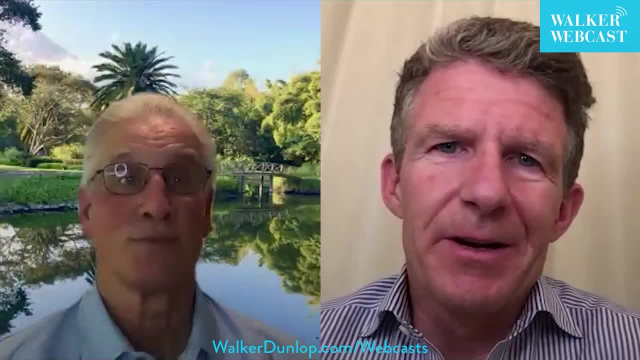 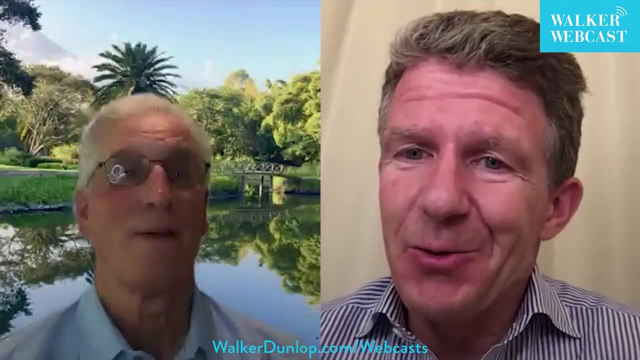 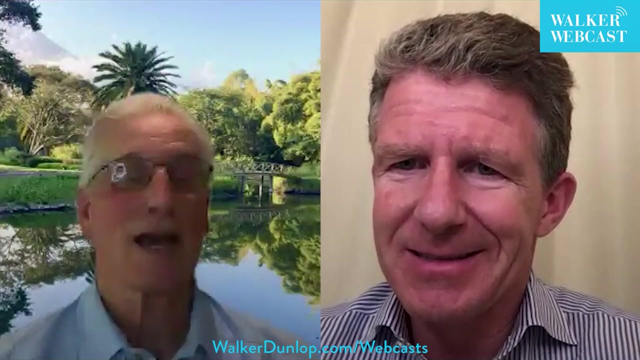 Clean, safe nuclear energy. Get out of burning all that coal. Yes, yes, Wow, Peter, Thank you. You're still holding. you're still holding firm on seventy five to two hundred basis points of cuts this year. Yes, yes. 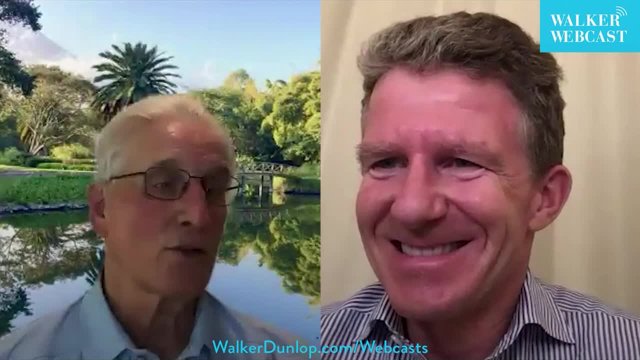 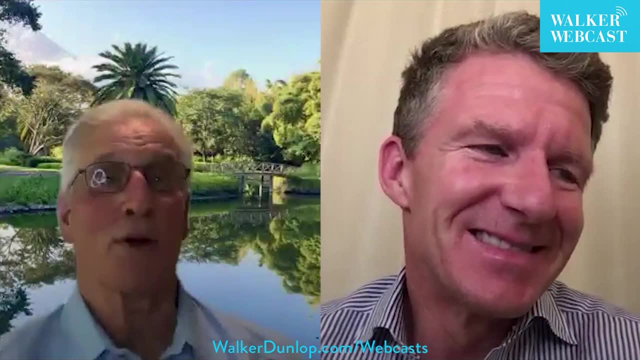 And I'm still holding firm that someone will win the election. Yeah, I didn't get to that today, We'll get to that next time. By the way, I get a lot of people asking my prediction about the election, and my prediction is: somebody will win. 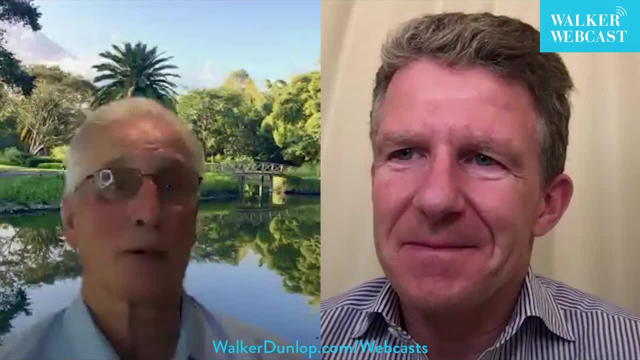 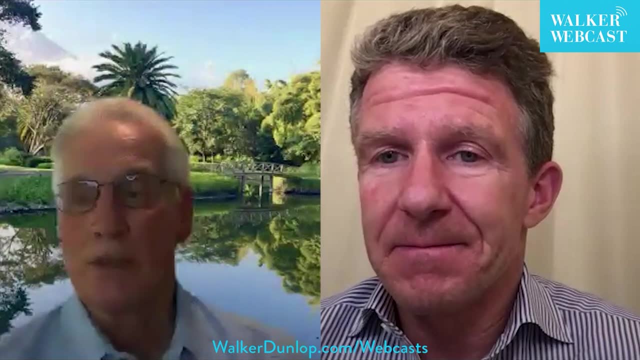 And no matter who it is, a whole lot of people are going to be unhappy. I feel comfortable in that. I feel comfortable in that prediction. Would you say that one is better for commercial real estate than the other? Not notably, Not notably. 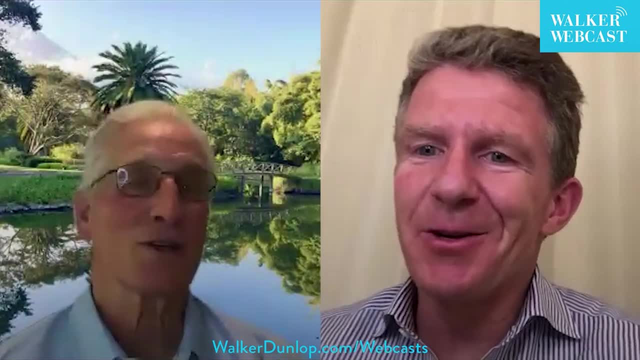 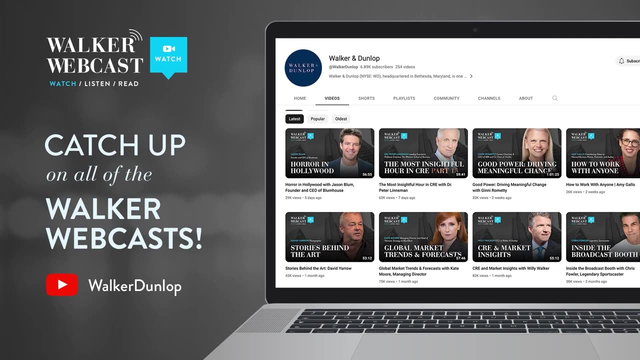 We will leave it there. Peter, great to see you, Look forward to seeing you in two weeks. I look forward to seeing you live in two weeks. Very much looking forward to it. See you soon, Be good, See you, Bye, bye. Bye, bye. North Carolina is a hotspot for state-to-state migration. There's no denying it at this point. This has been going on for a handful of years and I honestly think this is the beginning of a 10 to 15-year stretch of insane growth. And as this migration picks up steam, more and more people 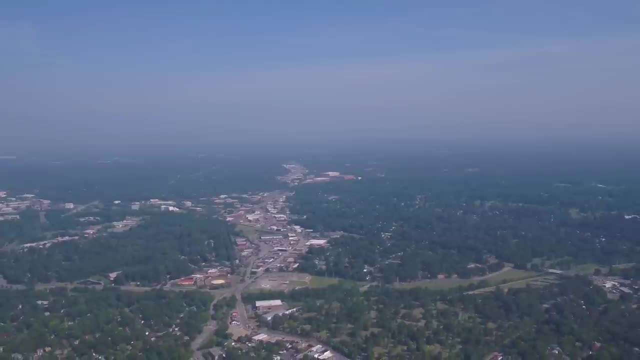 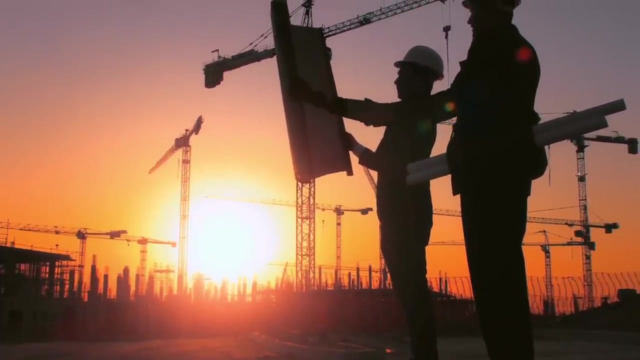 will be moving to the suburbs around North Carolina's major cities. Right now in North Carolina they have a lot of new developments going up around their biggest cities. North Carolina ranked fourth behind Texas, California and Florida, for new home construction in 2021. 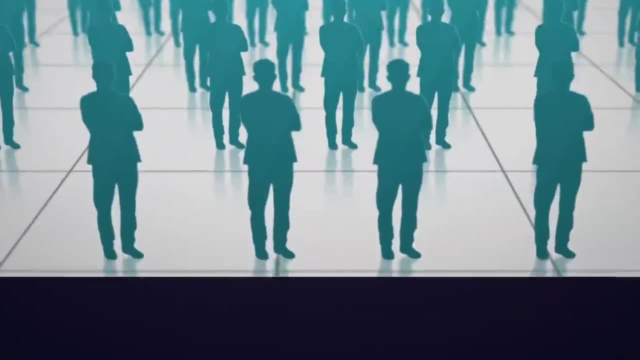 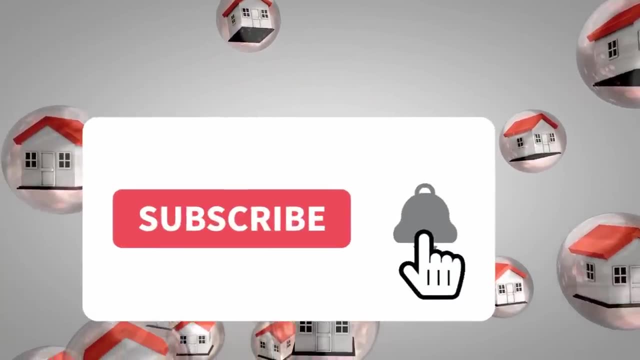 and in 2022. And that should tell you they're planning on a big surge in people, because developers don't build if they don't have a market. Today we're looking at the best suburbs to move to in the Tar Heel State in 2024.. All right, let's take a look. town life. The community is super diverse, which I love, like I've said before, because this means you're going to get some great food options, from tacos to authentic Chinese food. The town's parks are like little green escapes, perfect for afternoon jogging, going for a little hike. 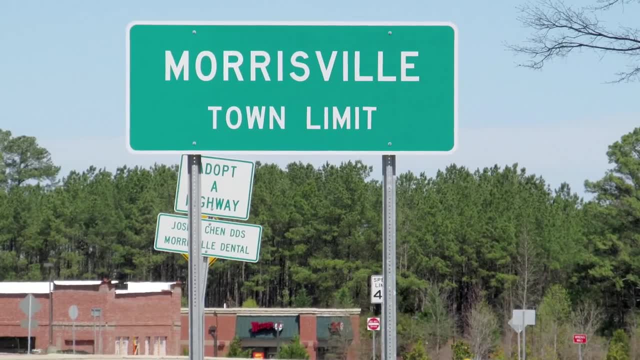 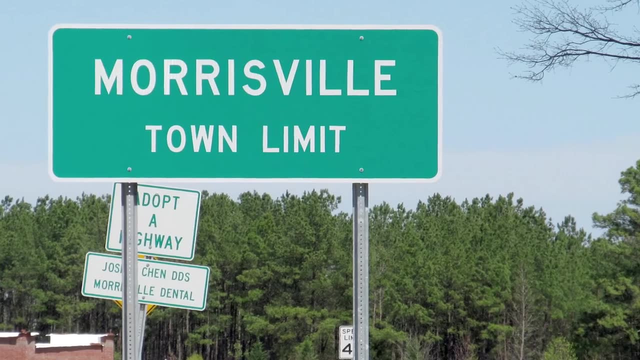 weekend picnics, Stuff like that. Another cool thing is Morrisville's not too far away from the airport, so it's a breeze for those who have to travel a lot. It's got this friendly, bustling atmosphere that's sort of contagious. You can't help but feel at home here. It's kind of this thing with North Carolina. I've